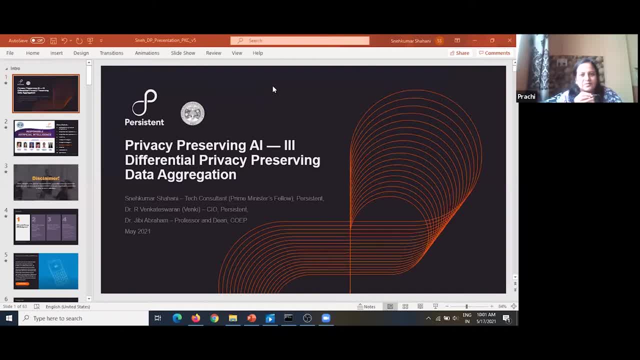 Just I want to share this with everyone. Sneha Kumar is not well today, but he has agreed He is willing to take the session today. We are very happy about it And I would request you, Sneha Kumar, to please take breaks in between. It is a long session- one and a half. 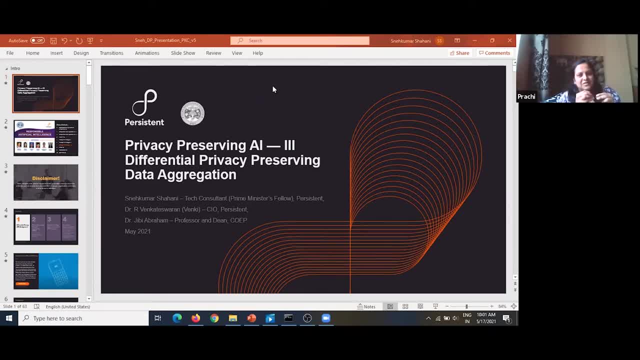 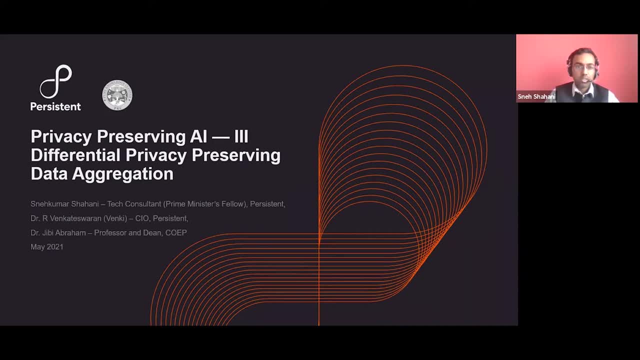 hour session. Please take sufficient breaks Over to you. Okay, thank you, Okay. so thank you very much for the good, wonderful introduction. So my name is Sneha Kumar Sahani and today I will be presenting on the third session of the Privacy Preserving AI. The topic of today's presentation is related to differential 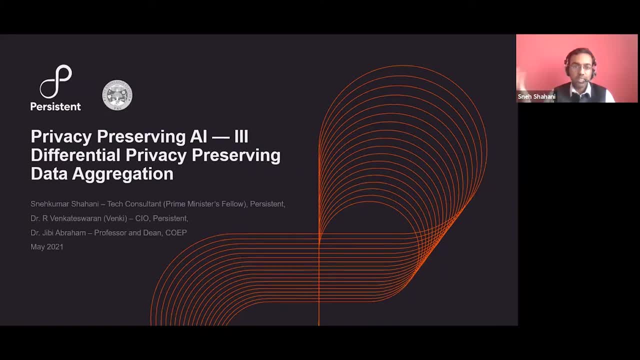 privacy, and we will be focusing on differential privacy, preserving data aggregation. So this work I have done, along with my PhD guides, Dr R Venkateshwaran, who is CIO at Persistent, and Dr G B Abraman, She is Dean and Professor at CUIP. 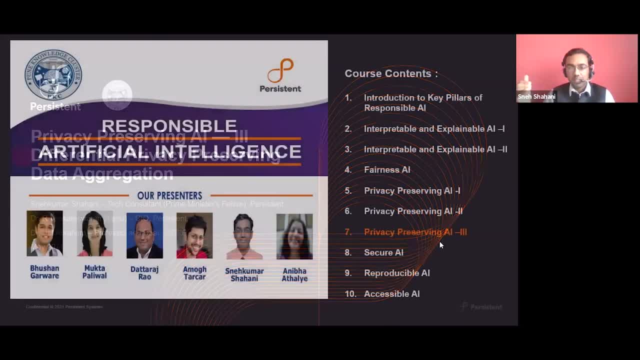 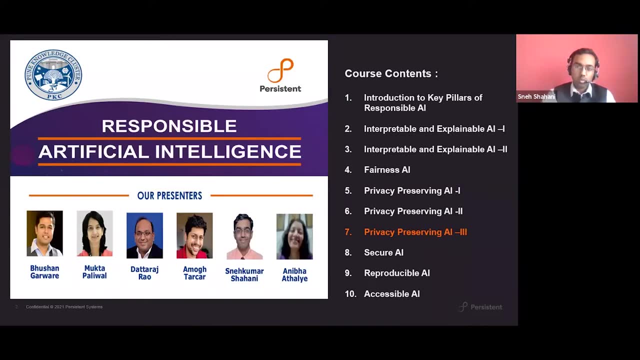 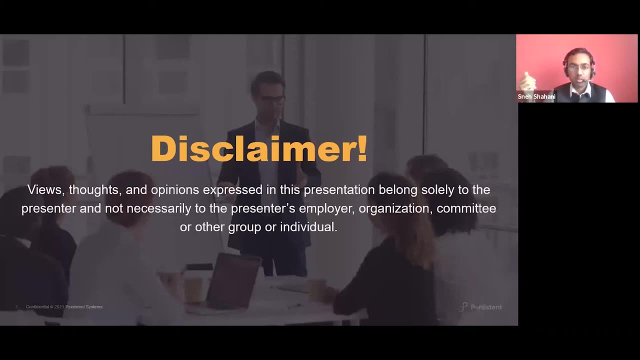 So this session is the seventh in the series, of the Responsible AI series, And we still have three more sessions to go. The disclaimer: all views and thoughts that will be expressed in the presentation solely belong to me and they don't necessarily reflect the Persistent's or any other organization's. 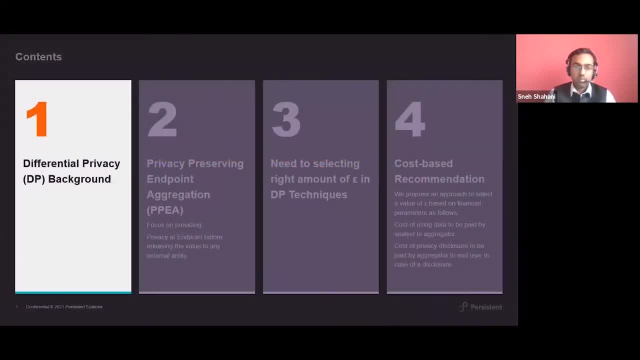 point of view. So, before we start with the presentation on differential privacy, preserving data aggregation, I would like to say thank you very much to all of you who have participated in this session. We are very excited to be here and to share with you a brief overview of what is a differential. 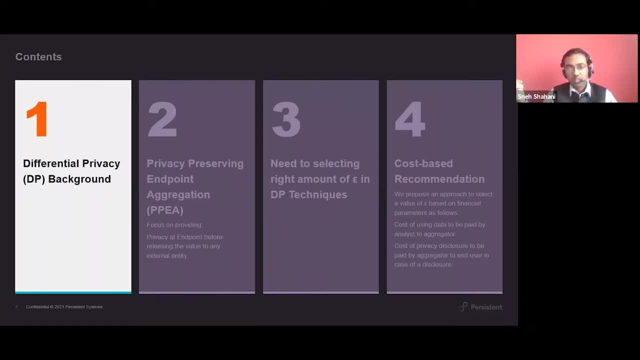 privacy, preserving data aggregation. So let me ask a question to the audience. We use this term security and privacy rather interchangeably, But still these two are different. So can anyone give some points of difference between security and privacy? Maybe you want to unmute yourself and give. 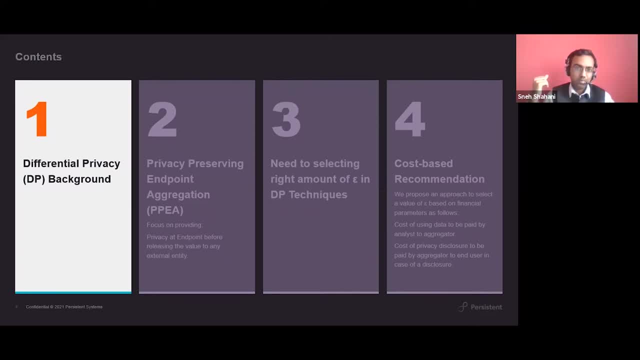 some point of difference between security and privacy. Any computer that has an AI device that is able to provide security and privacy. what do you think is the difference? So any computer science graduates who have learned about this difference between authentication and authorization? it is very similar to the difference between authentication and 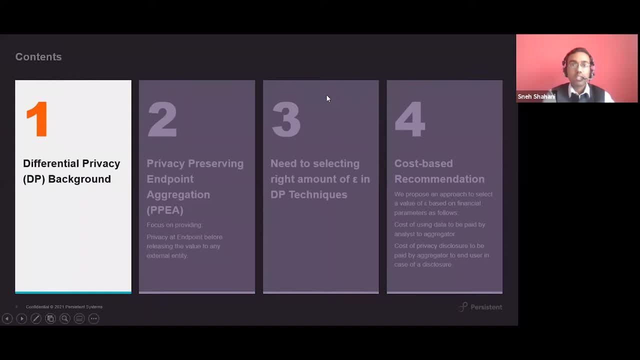 authorization. So are they allowed to unmute themselves, or you are going to answer in chat? Yes, they can unmute themselves and answer, or in the chat box also they can. So we have one answer from Dr Shamsundar and he is saying that security covers all. 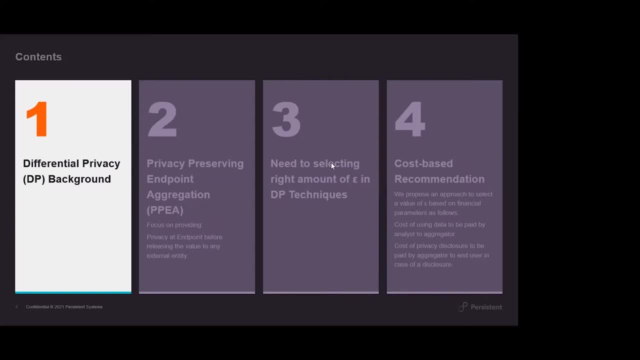 aspects end to end, and privacy is related to granular aspects of the data and its usage. Okay, that's close enough. Okay, so maybe I have given a hint. now It is very much close to authentication and authorization. We have something else also. 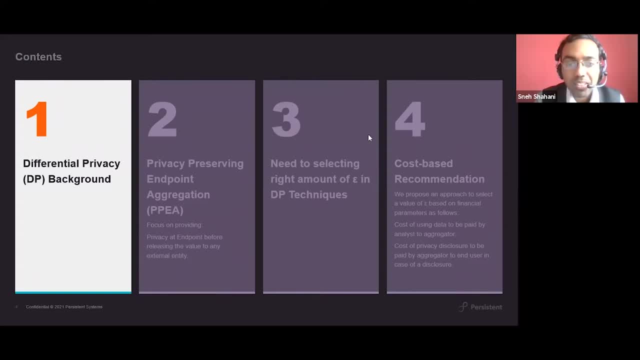 It's keeping your data secure and privacy is not identifying. Glad you didn't say that privacy is keeping private. Okay, so the security, authentication and authorization is something like authentication is binary, while authorization is what you are authorized to do. Okay, So security is also like that. 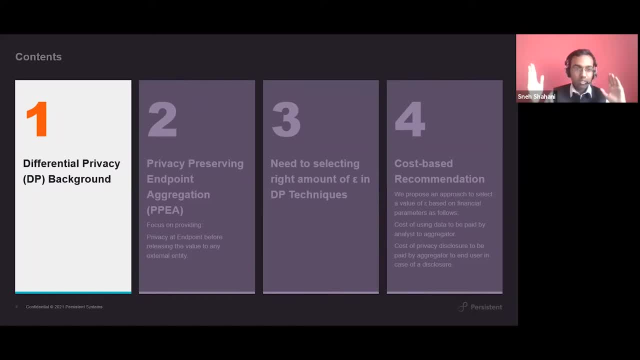 Security is binary, whether your data is secure or not secure. it is binary whether it can be accessed by the authenticated people or not. So in security, the attacker is outside the system, So genuine users should be able to access the data and do anything with it, while outsiders 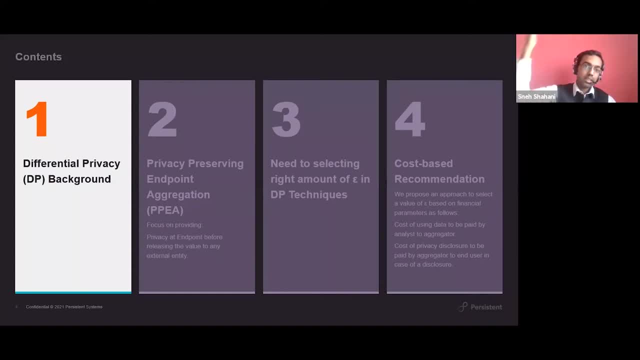 should not be able to access the data If it is not secure. outsiders can access the data. Yeah, I think it's very clear: can access the data. so it is like attacker is outside the system and genuine people are inside. the people who are inside who are allowed to access the system. they are inside the system. 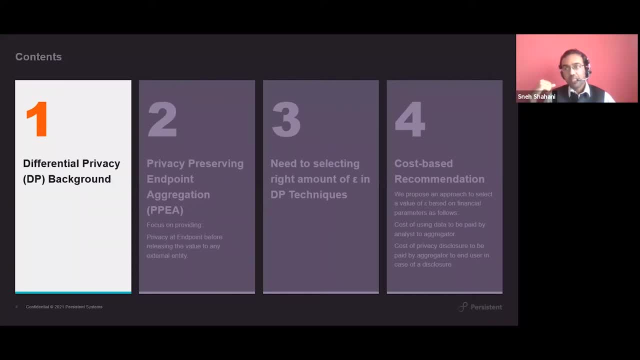 in privacy. it is not totally binary. privacy is like selective disclosure of the data. the ability to seclude information about yourself and disclose only in the selective manner is known as privacy. so the data should be use allow. you should be able to allow your data should to be used only for the purpose that you are allowing to. it should not be useful for any. 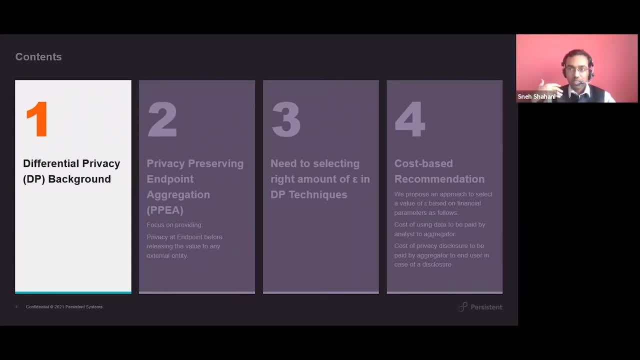 other purpose. that is what is we understand from privacy. now, in this case, attacker is inside the system, say you. you are a genuine person who is allowed to use the data for a particular purpose and you misuse it for some other purpose. you are a genuine person who is allowed to use the data for a particular purpose. 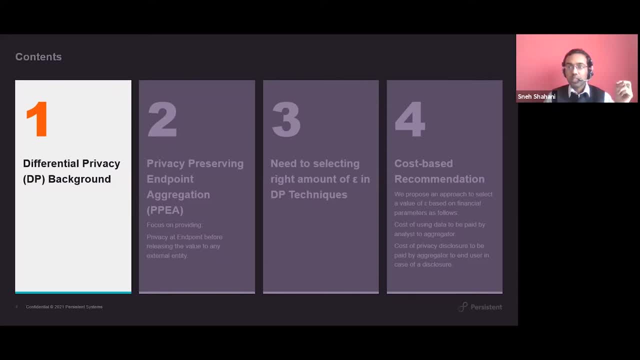 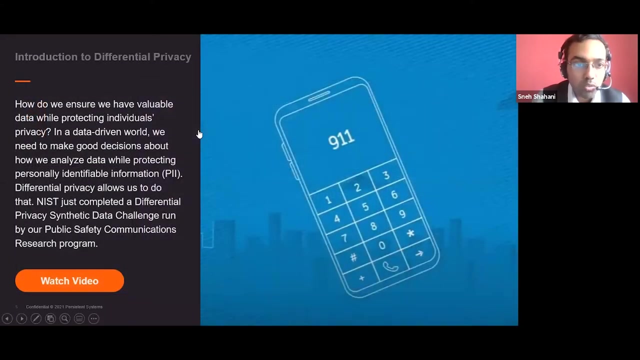 then that is a breach of privacy. so this is. these are some of the differences between security and privacy. so now, before we begin the presentation, so i wanted to show a small video. let me see, sound is shared, so now i will give a small introduction on differential privacy. 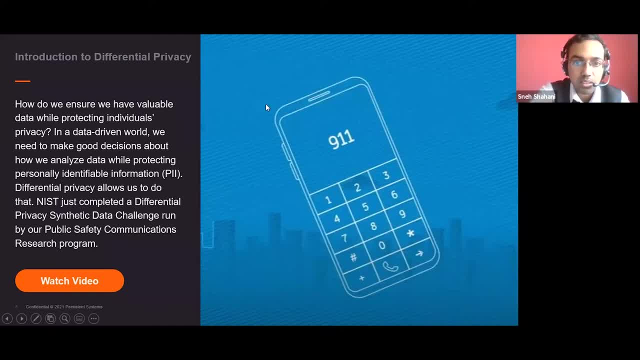 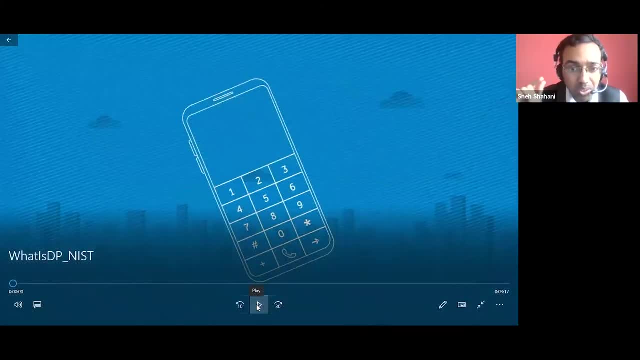 small video on differential privacy, and then we will start with small video on differential privacy, and then we will start with small video on differential privacy and then we will start with the definitions and some concepts. so please let me know if you are not able to hear the voice in the video. 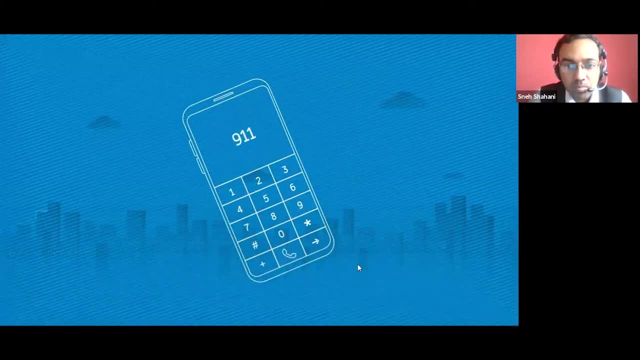 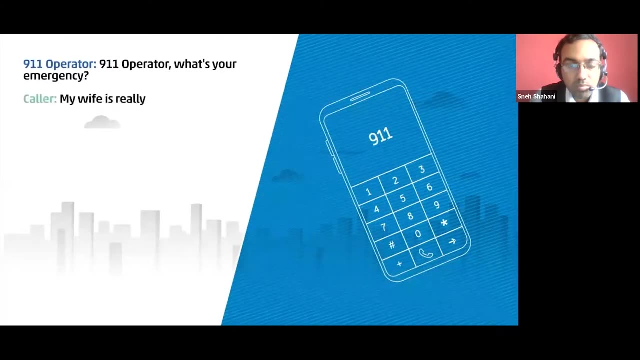 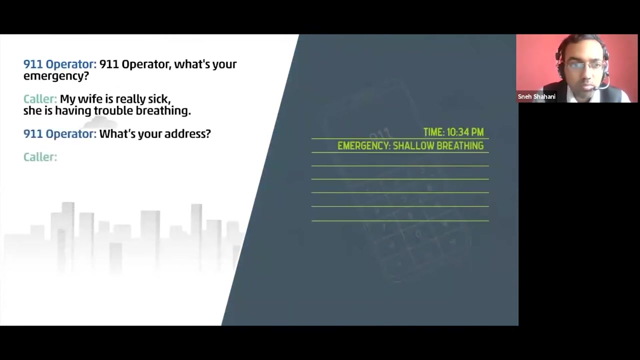 so i'll start the video now. so i'll start the video now. 9-1-1 operator. what's your emergency? my wife is really sick. 9-1-1 operator. what's your emergency? my wife is really sick. what's your address? 1235, 1235. 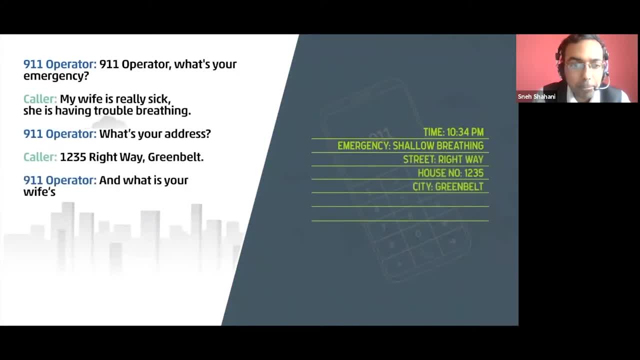 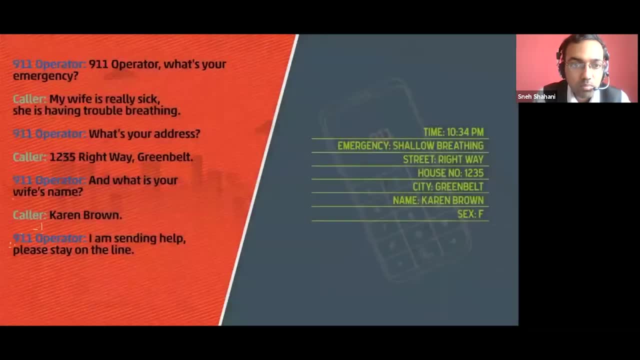 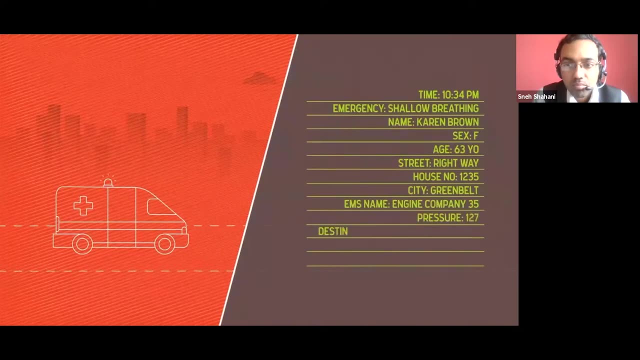 Right way, Greenbelt. And what is your wife's name? Karen Brown, I'm sending help. Please stay on the line, Okay? This is a typical call that 911 operators receive every single day. Each call provides a wealth of information about a person in need. 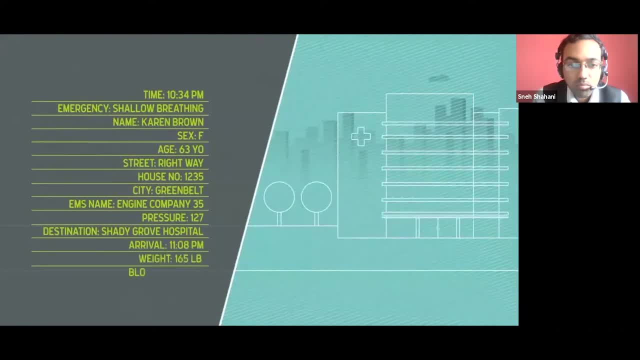 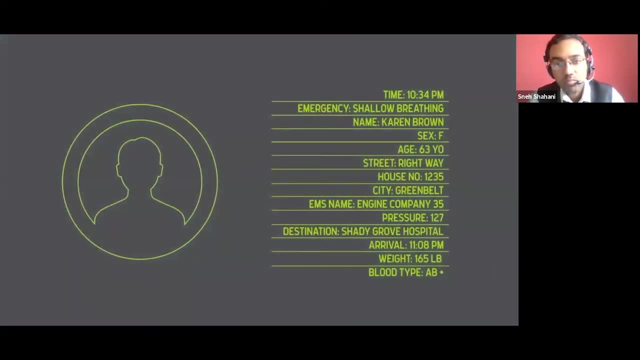 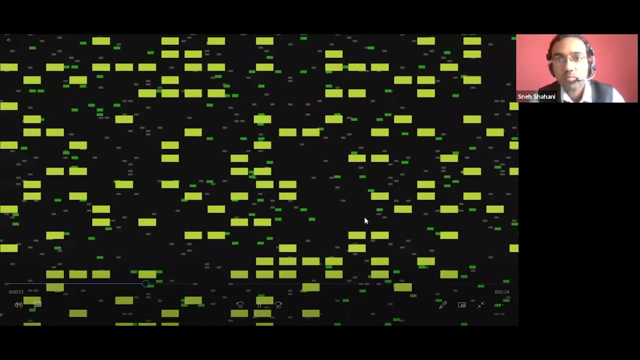 In addition to contact information, EMS and hospital staff add health information to Karen's medical record as they treat her. Most of this data is PII, or personally identifiable information, which is key to a person's identity. This information is stored in large databases all across the country. 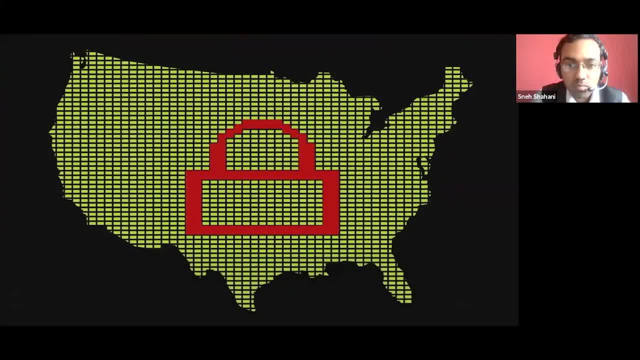 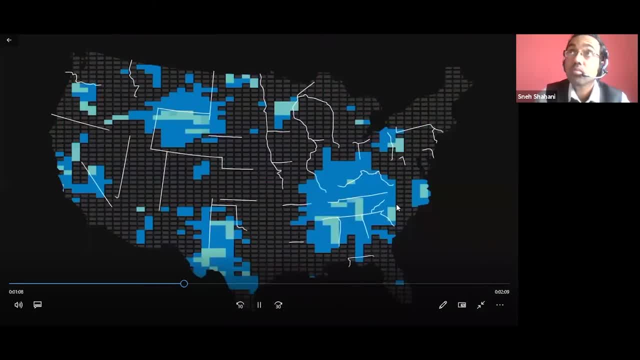 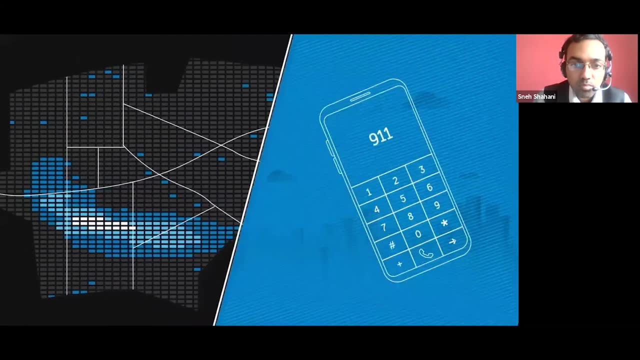 Use of this data is protected by law in order to preserve your privacy. But what if we could use this data without compromising your privacy? Imagine if we could aggregate data to see trends. What if access to Karen's and others' data show that 911 had received multiple calls about breathing problems around the same time? 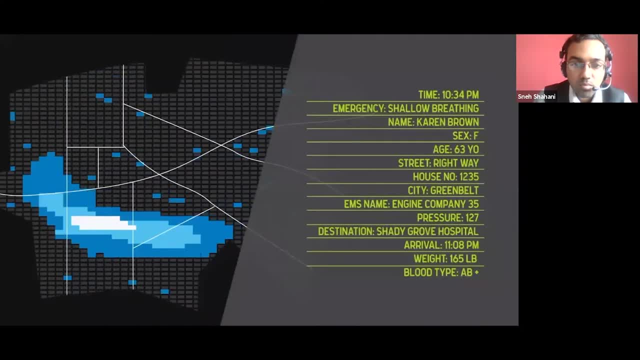 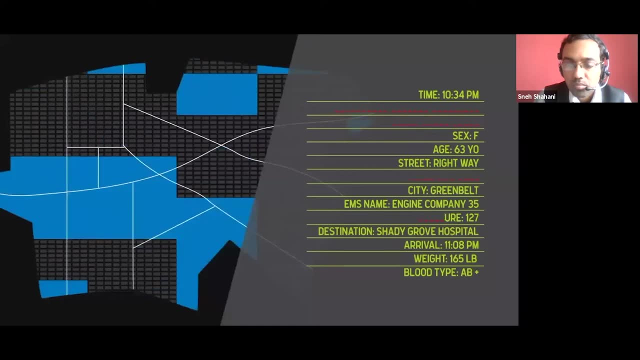 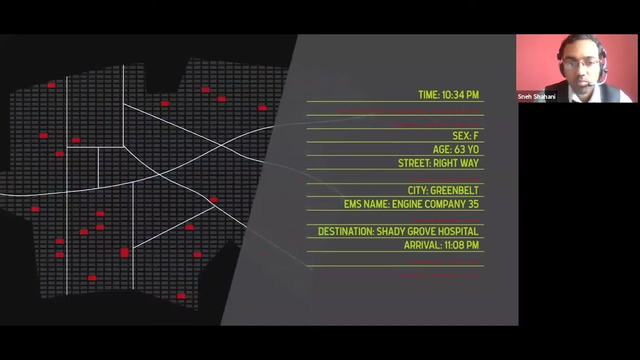 We might pinpoint the culprit. Right now, use of data in this way is allowed as long as we redact the personally identifiable information, But by removing PII we drastically limit the data's usefulness and we don't always protect identities. For example, if Karen lived on a small street, her identity could easily be revealed just by sharing her age and street name. 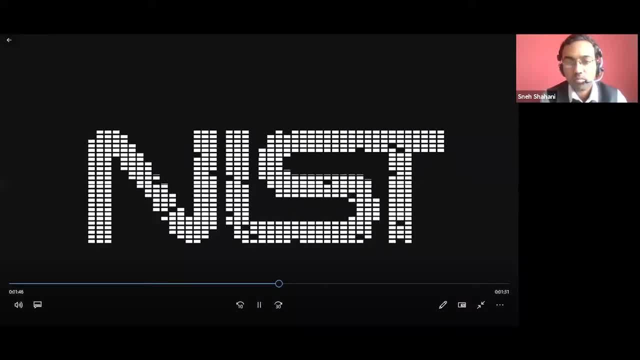 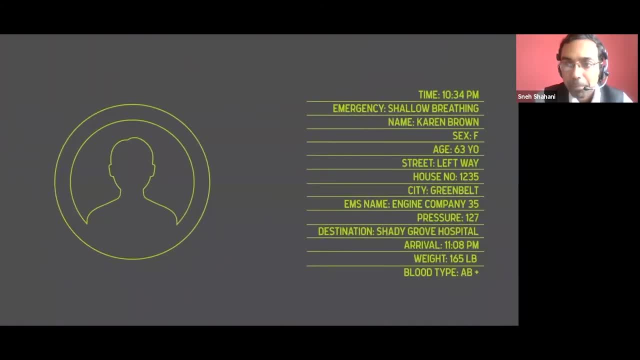 NIST scientists are seeking ways to improve the sharing of data while protecting individual identities through measurement and evaluation. By slightly altering the personal information, for example Karen's age or home address, we reduce the risk of compromising privacy while still allowing data to be shared. 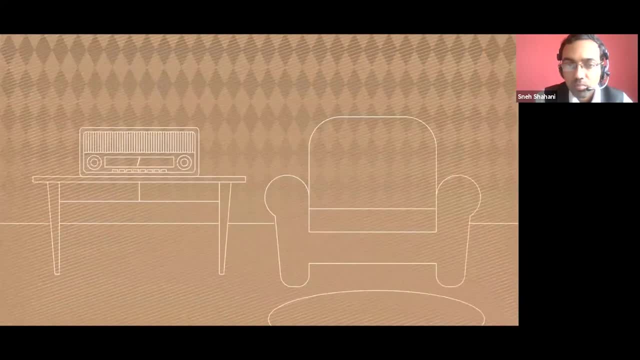 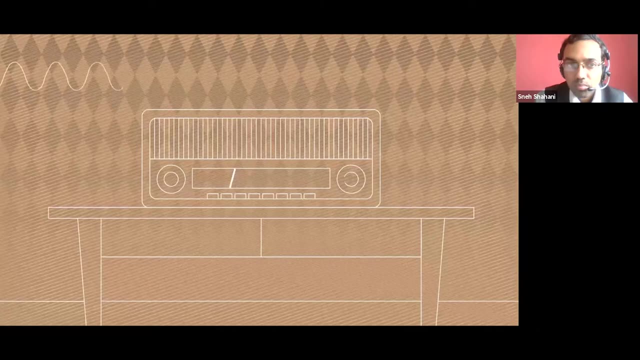 Altering the data is like adding a bit of static noise to a radio broadcast. When your radio is tuned in to the exact frequency of the station, you clearly hear what's being said. If you move the frequency a bit to the left or right, static noise muddies the sound but doesn't compromise the message. 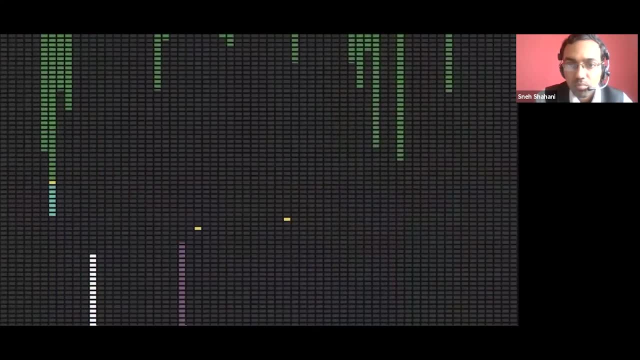 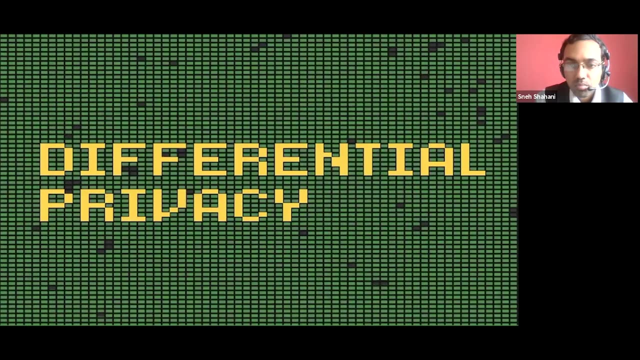 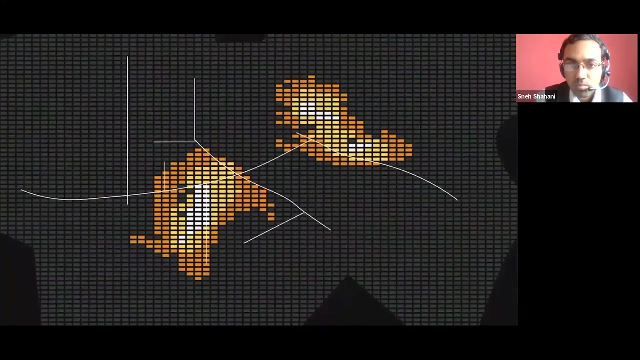 This process of adding carefully tailored noise and altering identifiable information within whole data sets is called differential privacy. When this process is applied to large amounts of data, it becomes a provable guarantee of privacy. Differential privacy allows all of the information to become useful and actionable data. 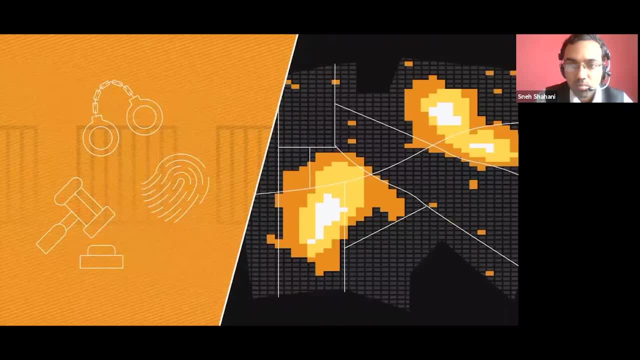 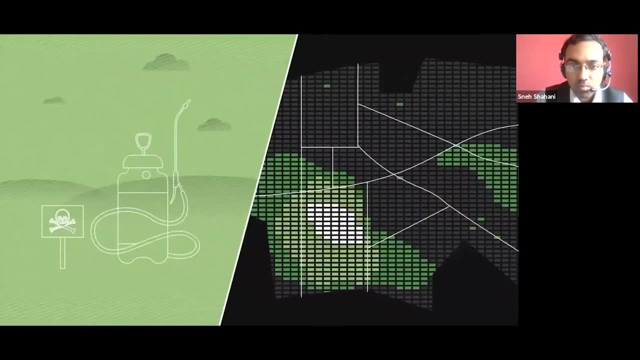 This can lead to identifying underlying problems or trends in neighborhoods, like reasons for spikes in crimes or a higher number of accidents due to poor road lighting. In Karen's case, access to data revealed that her community was experiencing breathing problems due to over-application of a new lawn pesticide. 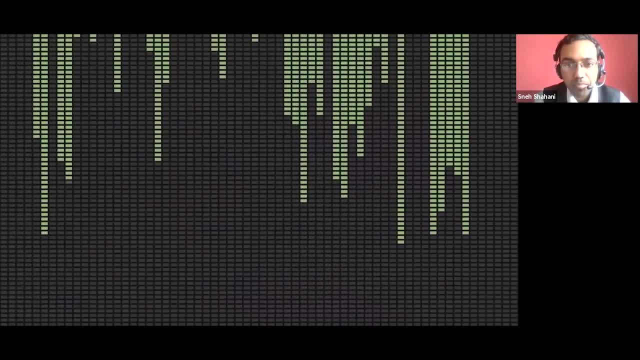 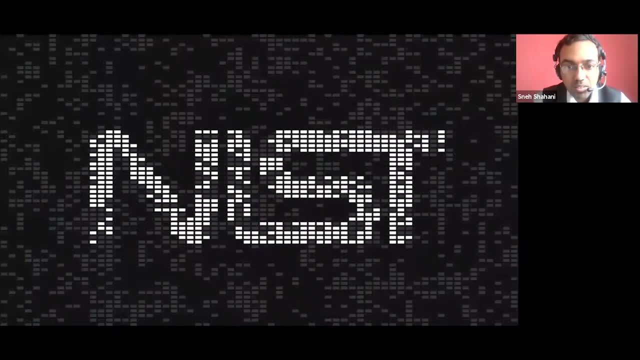 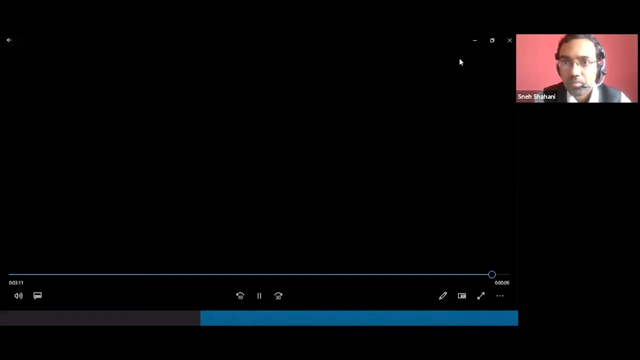 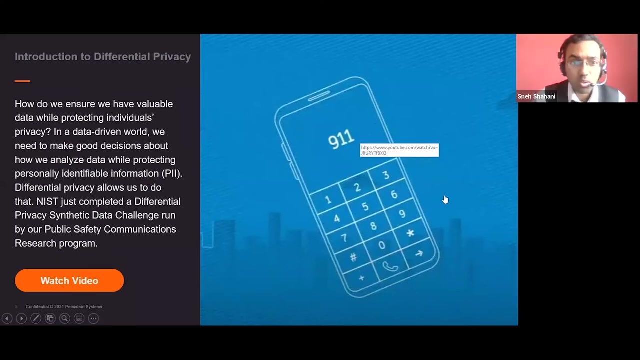 a problem that was quickly rectified. In today's data-driven world, differential privacy allows us to make more educated decisions that could improve the quality of our lives, Also in thiswo- Okay, Thank you. So in this video we saw that the Data 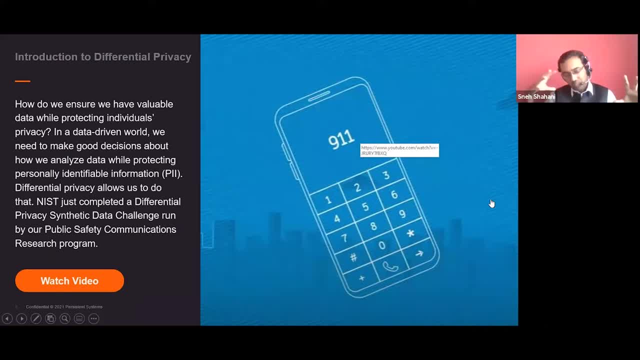 if it is analyzed to identify the trends of the entire group or the community. that is one aspect of using the data: To identify general behavior of the entire community or group of trends. In this case, at the very beginning, when we look at the data, we see that it is being analyzed. 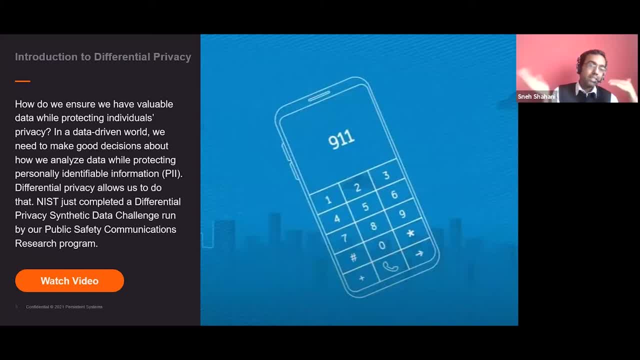 The nature of the data is a general mode. They are being used to identify general behavior of the entire community or group individuals, while it is other other aspect of using the data when we can identify, uh, some personally identifiable information about one particular individual. so our objective is to say 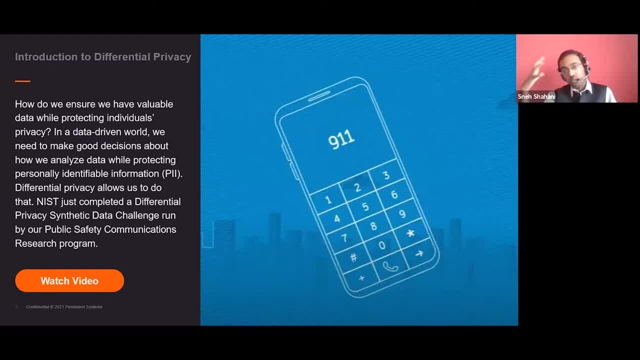 that data should be useful to analyze the trends of the entire group, but at the same time, if we try to analyze or identify traits of the individual, then it should not be, it should not allow that kind of a usage. so that is what we achieve by using differential privacy. 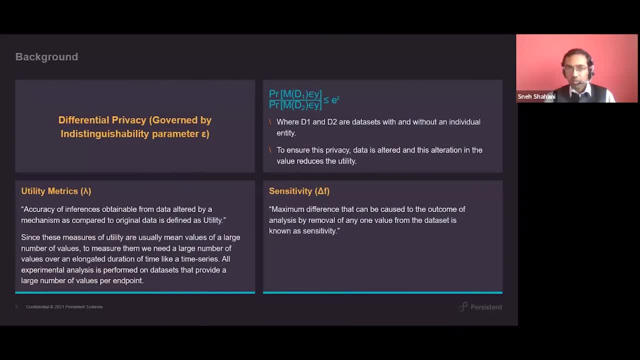 so now some concepts of differential privacy are. so now we understand the difference between privacy and security and our objective. so now let us come to the some of the basic definitions of differential privacy. so differential privacy is also known as epsilon differential privacy because it is measured by a parameter called epsilon. 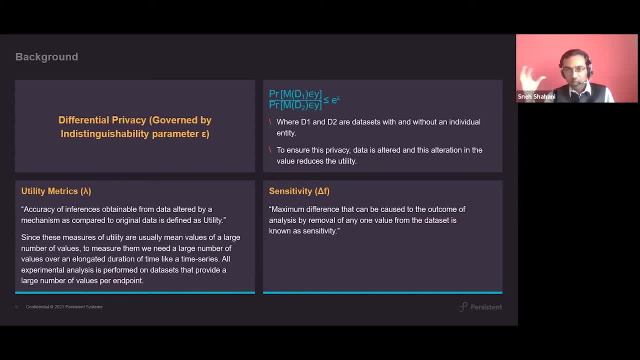 so to understand the interpretation of epsilon, let us take a data set d1 and from this data set we remove one record of one individual and we get a data set d2. now we have a data set d1 with all records and data set d2 with all records except one individual. so what differential privacy says that we the ability to 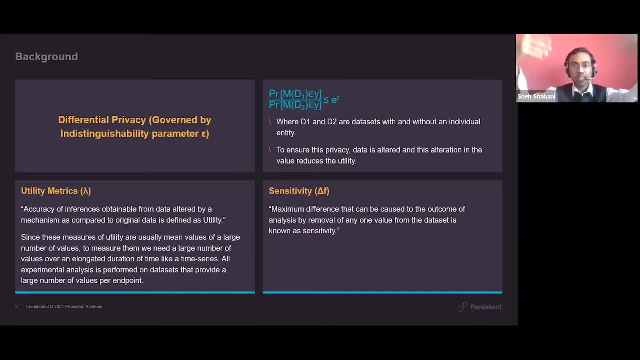 distinguish between these two data sets from the outcome of analysis. it has to be limited. say, for example, we are computing some of all these values or some we are computing a ml model using this data set. so just by looking at these two models you should not be able to the ability to distinguish. 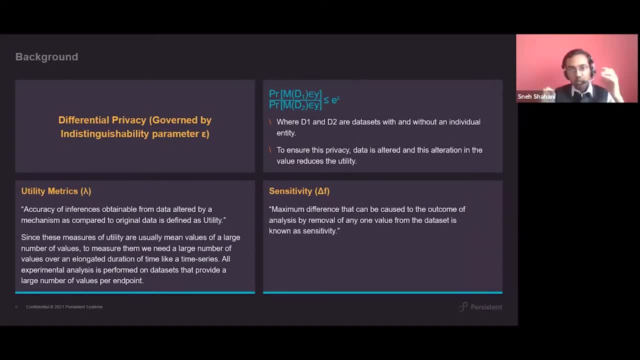 should be limited. so probability of getting an outcome y from data set d1 and probability of getting same outcome y from data set d2. the ratio of these two probabilities is bound by e raised to epsilon, so smaller the value of epsilon. e raised to epsilon equal to one. if, say, epsilon equal to zero, then 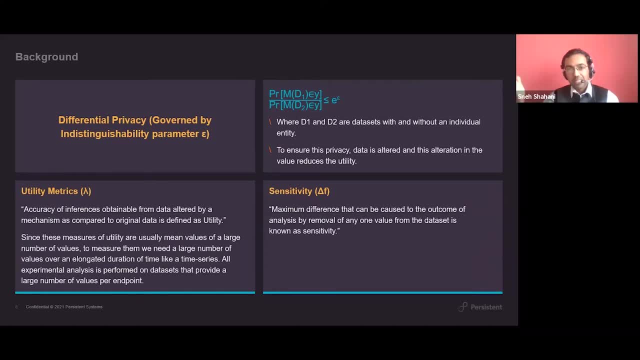 these two probabilities are indistinguishable. so epsilon is in a way a measure of indistinguishability of these two data sets. that's how we measure the differential privacy by using a parameter of indistinguishability. so to ensure this kind of a privacy, we alter the data in some particular way, say by adding random noise to. 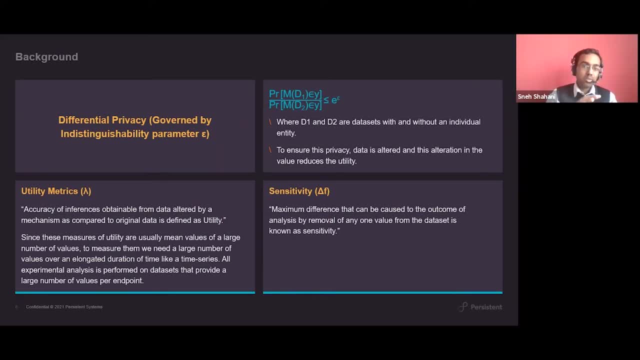 the data. so as we add random noise to the data, we add some randomization along with the data. the privacy improves but the usefulness of the data reduces. so by adding this random noise we provide some protection to the outlier and the data point. that can be noticed just by the outcomes. 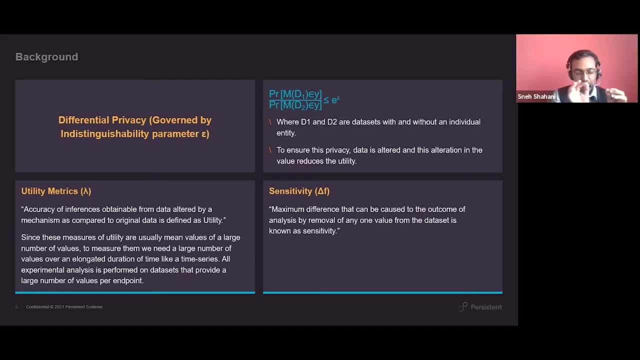 say for example: uh, from 100 values which are in the range 0 to 1 of the value is 100 or 1000 high value. so whether that value is present or not can be easily identified, even if we have only the sum of those values. the outliers and some kind of values can be out and 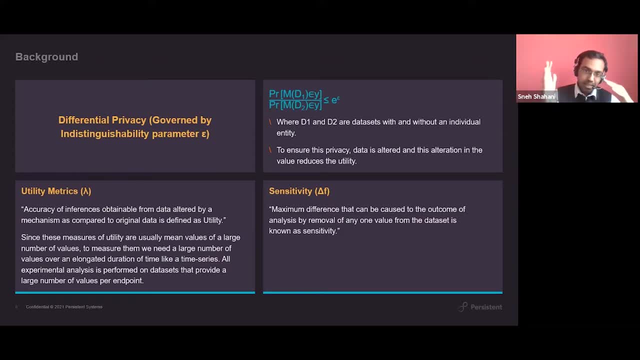 different only from the outcome of the analysis. so if we add random noise to all the values, we reduce the probability of identifying that outliers or, for the that matter, any individual in the data. but by adding those noise the usefulness is decreased. so we have to measure usefulness also. the accuracy of inference is. 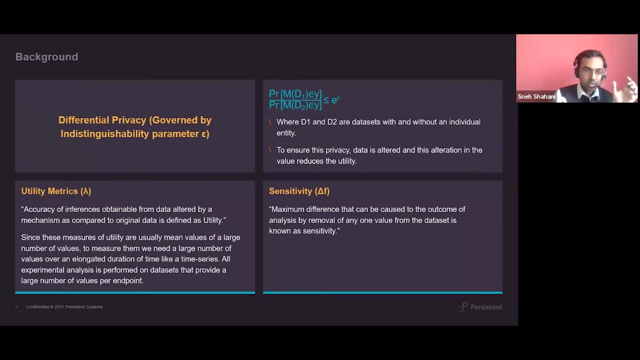 obtainable from data altered by a mechanism- in our case differential private mechanism- as compared to the original data. so we get some usefulness as come from the original data and some usefulness in the transformed data or the private, differentially private data. the difference between these two utilities is known as utility of the method of differential privacy. so these 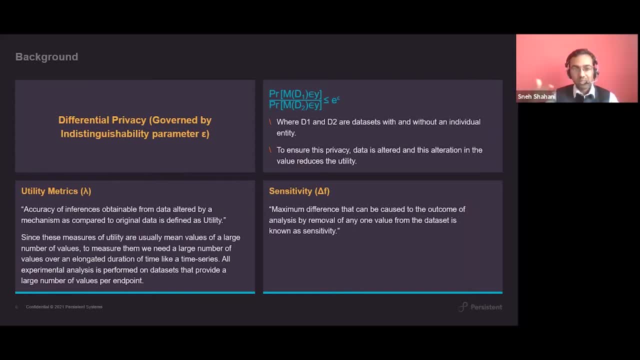 measures are usually computed as mean values of large values and we usually have time series data on which we do that. another very important definition is sensitivity. sensitivity is the maximum difference that can be caused to the outcome of analysis by removal of one value from the data set. 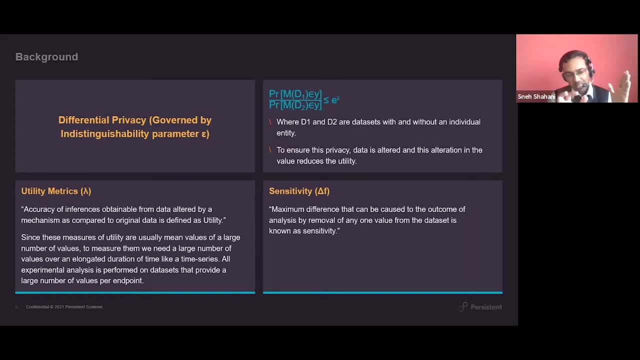 say, for example, we have a data set d1 and we are computing count. then by removal of one element, what is the maximum difference that can be count caused to the count? anyone would like to answer that in chat. maximum difference that can be caused to the statistic called count. so by removing one value from the 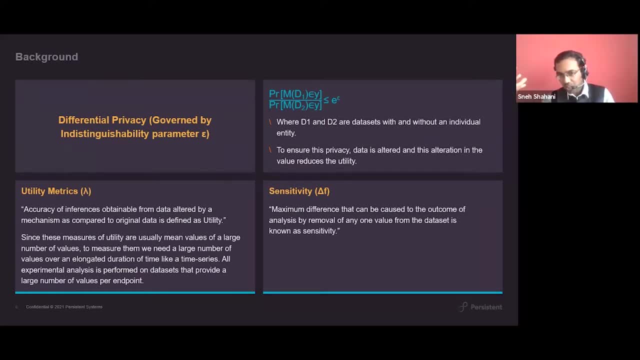 data set. what is the maximum difference that can be caused to the outcome? that is count. okay, so this time i will give the answer. the answer is one. so by removing one element, the count can change by one only. so, similarly, if you are computing a histogram, histogram is also a. 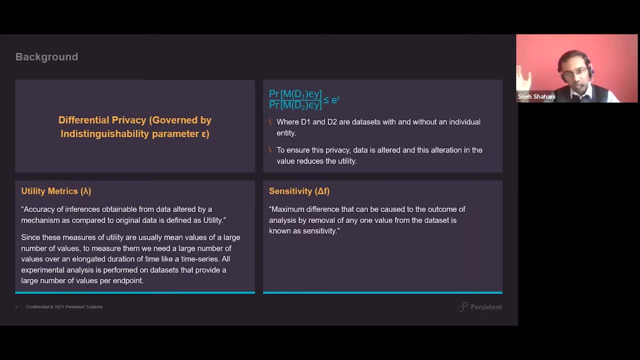 measure of counts, of intervals. still, in case of histogram also, the sensitivity is one. so for count and histogram the sensitivity is one. but now say, for example, we are calculating some of the data sets, some of the data set, then what is the maximum difference that can be caused to the outcome? 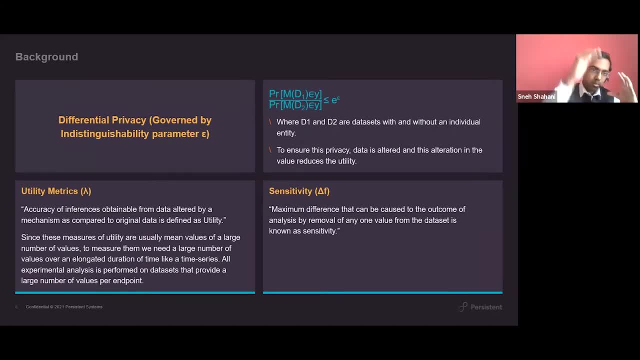 so maximum difference that can be caused from a data set is the max value in the data set. so in in this data set, say, max value is 100, then max maximum difference that can be caused by removal of any random value- we don't know which value is being removed- is the max value that can be. 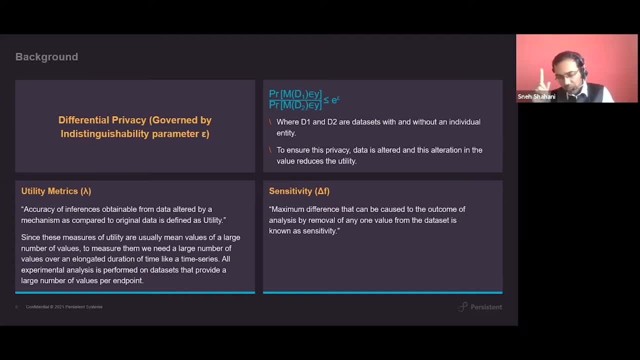 attained by the data set. the sensitivity of count histogram kind of query is one, while the sensitivity of some query is max. so we have understood three concepts. first one is differential privacy: the ability to indisting, measure of indistinguishability of two data sets, with or without an individual data set. 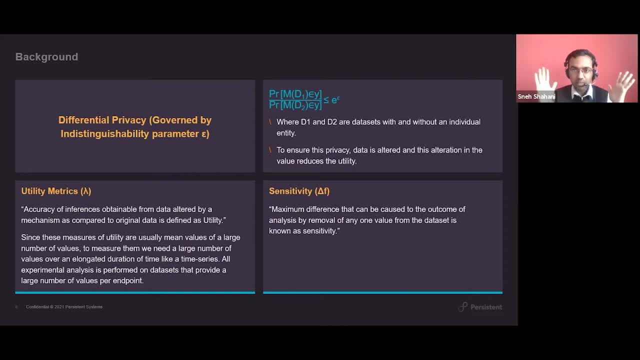 second one is utility matrix and third one is sensitivity. so please remember this concept. these are going to be used throughout the session. if you have any confusion, please ask now this. these are very important concepts that we are going to use throughout the session. thank you, so i'm moving ahead. 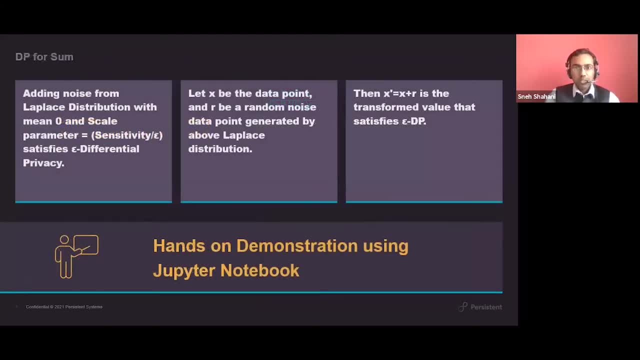 so differential privacy for some query. so we will. first we will understand how to provide differential privacy to some. so adding a noise that is this is a proven result. adding a noise from laplace distribution with mean zero and scale parameter as sensitivity by epsilon satisfies epsilon: differential privacy. 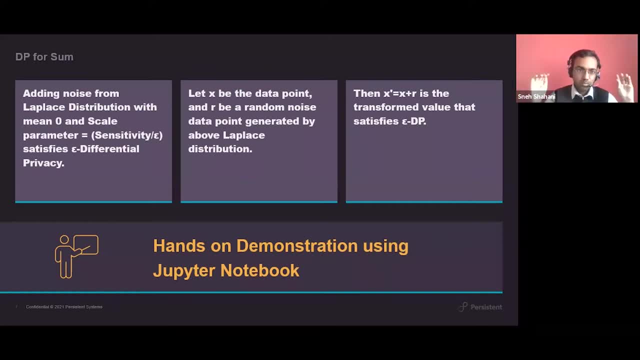 so this is a proven theorem. we are not going to the proof right now. so adding a noise from laplace distribution with mean 0 and scale parameter: scale of the distribution is like in gaussian distribution: scale is the standard deviation, while in this case it is known as scale parameter. 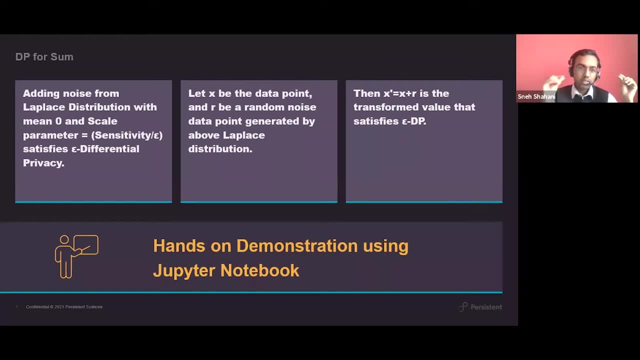 for laplace distribution. so adding a noise with mean 0 and scale parameter equal to sensitivity by epsilon satisfies epsilon differential privacy. let x be any data point in a series of data and r be a random noise generated from this laplace distribution, then x dash equal to. 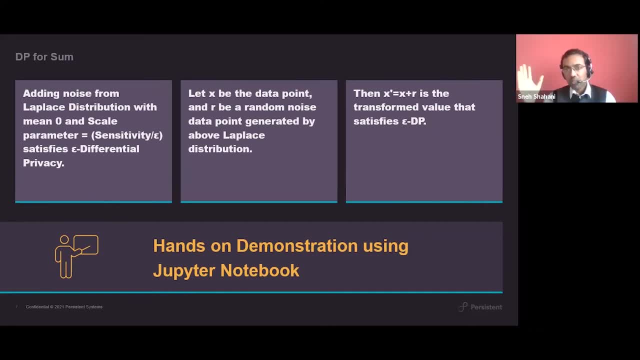 x plus r is the transformed value or the private value. that satisfies epsilon differential privacy. so we have a data set, d1- d and we add this random noise to all the data points. the transformed data satisfies epsilon differential privacy. so now, now i want to do a short hands-on demonstration using 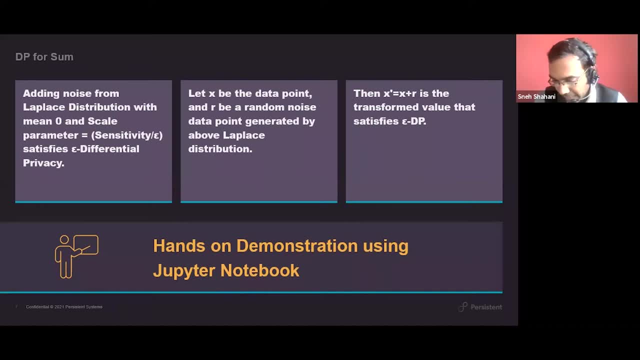 a jupiter notebook. so i hope everyone has started a blank jupiter notebook. so can you say yes in the chat so that i can understand that everybody is ready? sensitivity: yes, i will explain the meaning of sensitivity in in the hands-on demonstration and if after that also if there is confusion, we will. we will discuss that. 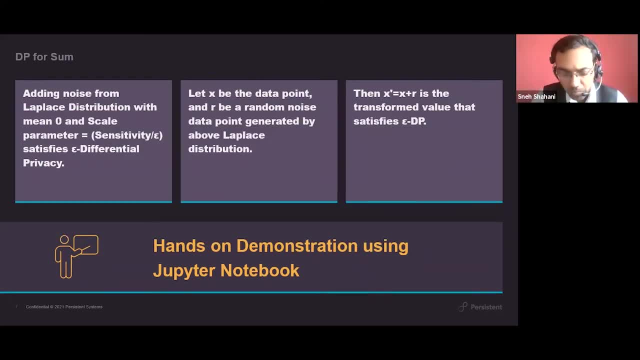 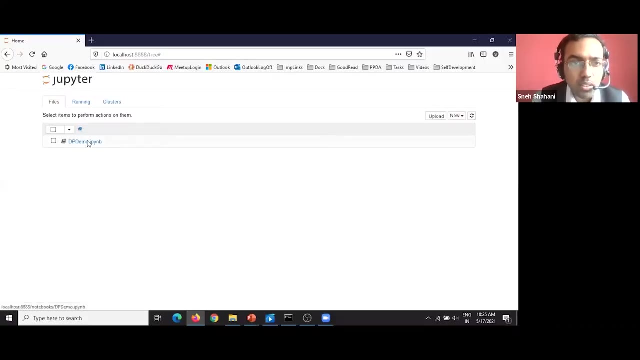 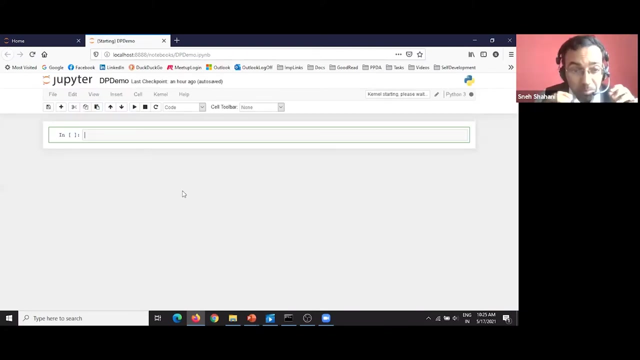 so if anyone is remaining to start the jupiter notebook, please let me know. we will start in next one minute. oh, we are running slightly late still, let me start right now. so can you see my screen blank jupiter notebook. okay, let me know if you are not able to see the screen, so we will start. 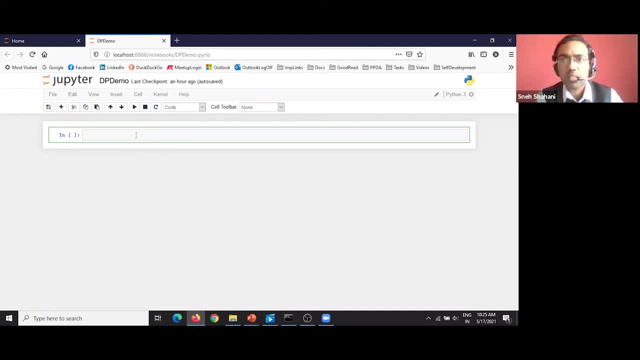 it's a very short demo. we will finish it quickly. i have not started using. i just need you to start a blank notebook. you need not know anything, we will learn right now- but i just want everyone to open a blank jupiter notebook. okay, okay, let us start. 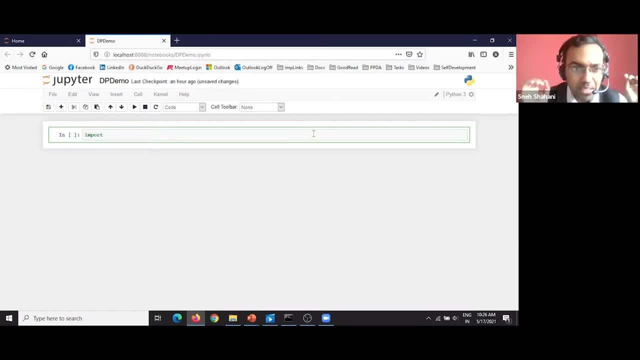 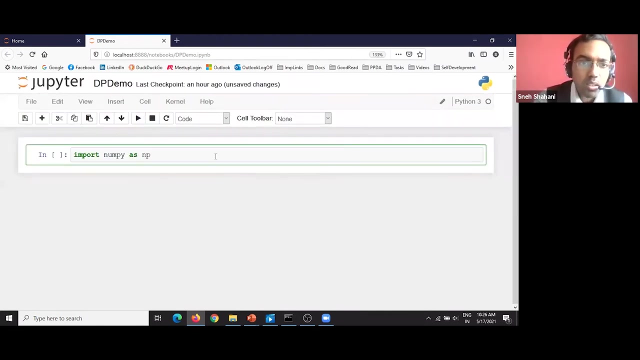 start right now. so please type with me import numpy as np. we are importing our lab numpy, library import numpy as np. let me see if i can expand my screen. so i'm executing this command, so i'm importing numpy as np and i will tell you um. so i will explore in later on so you know when we want. 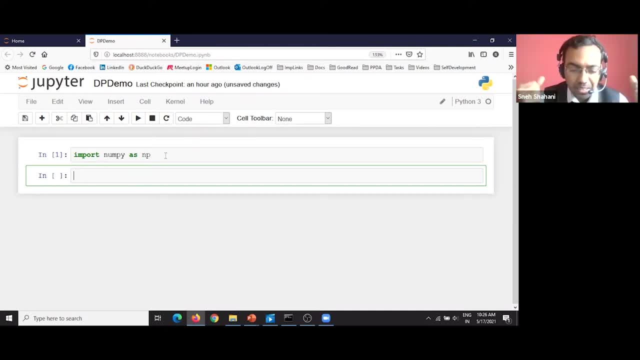 to install a alignment mechanism and we can use the enjoy and launch this problem. and i'm setting some parameters. first one is epsilon. epsilon equal to 0.5 and number: number of data points in the data set equal to say 5000. number of data points in the data set is equal to say 500. 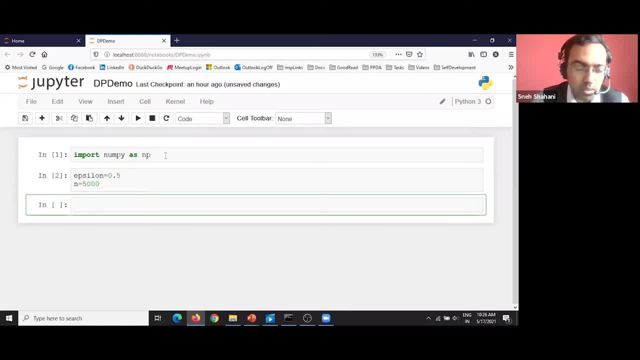 so i am storing these two variables. these we will use later on. so i am storing these two variables. these we will use later on. so i am storing these two variables. these we will use later on. so i hope you think this is helpful for you. so i hope you enjoyed watching this video. 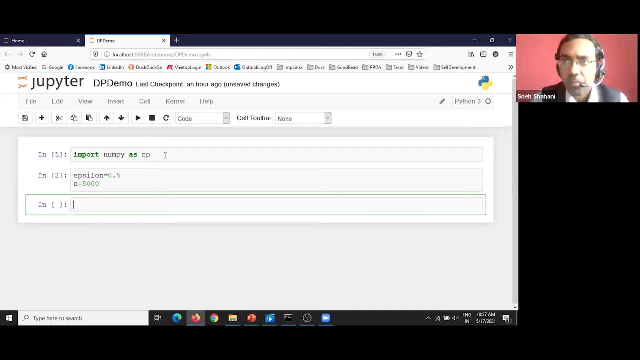 if you want to know further videos like this, leave comments or comment under the video. you all are with me. so now let us generate a data set of integers from 0 to 100. this we will call it as actual data set. actual data set equal to num, np, dot, random dot, randint, from 0 to 100. 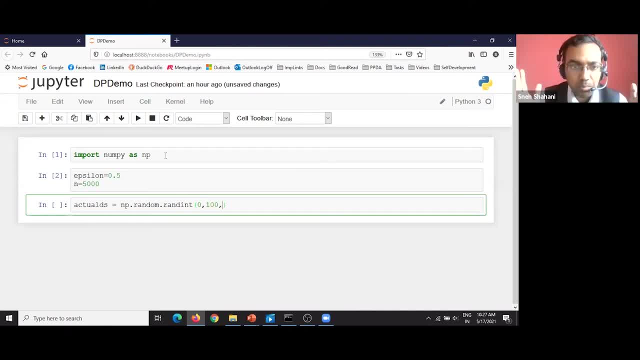 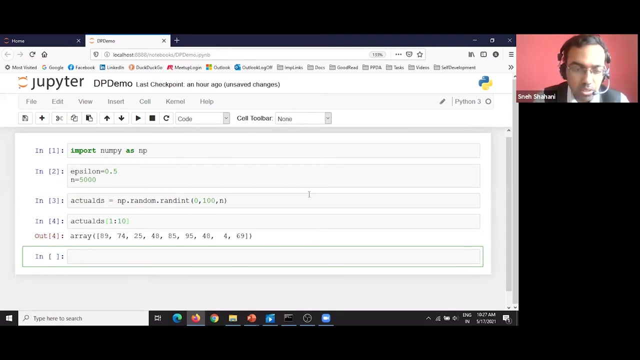 so we are generating a data set of random numbers from 0 to 100 n data points. let us check the first 10 data points. actual data set from first 10 data points. as you can see, this is the data set that we are generating: 89- 74. since this is random numbers, you will see some different values. 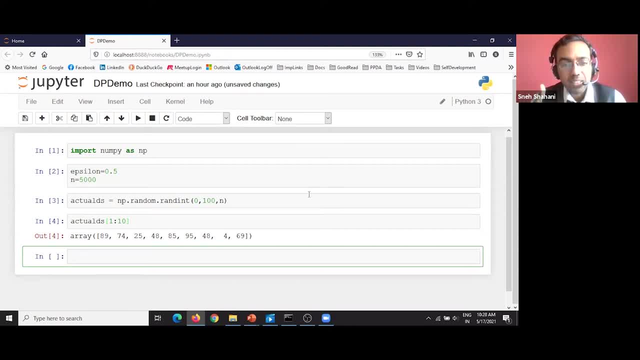 which are like this only in range 1 to 100. so now sensitivity: what will be the sensitivity of this data set, say in this data set, if we remove any one value? we don't know which one is removed. so what is the maximum difference that can be caused to the outcome? say outcome is sum of all these values. 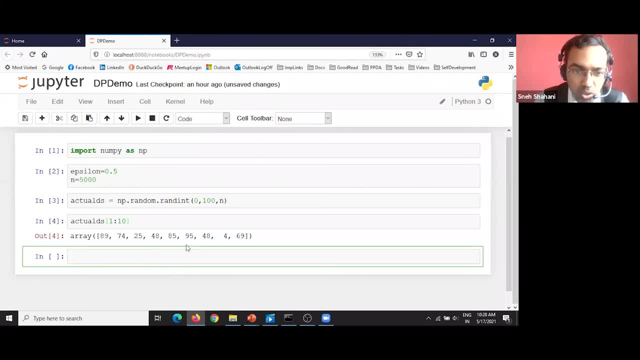 so max value here what we can see is 95, but in reality it can be anything between 0 to 100, usually then 99. so max value of this data set is the maximum difference that can be caused to the sum. so we will calculate sensitivity equal to np dot max. 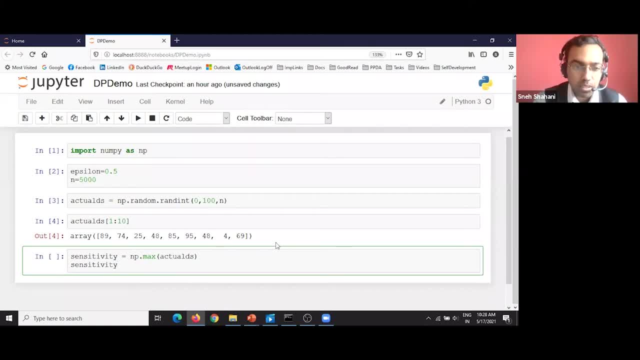 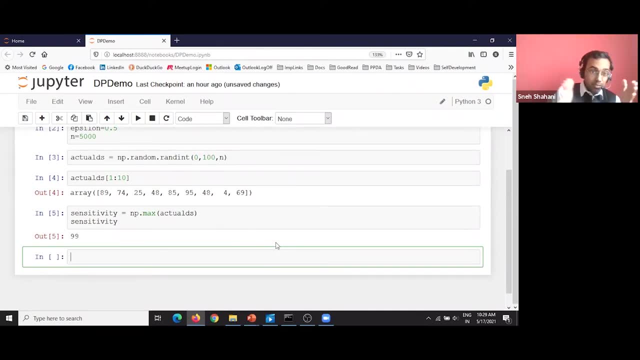 and then we will print the value to see what is the outcome. it is 99. so maximum difference from: for all the 5000 values, the maximum value is then 99, in this case the random values that we have generated. so max difference that can be caused to the outcome is: 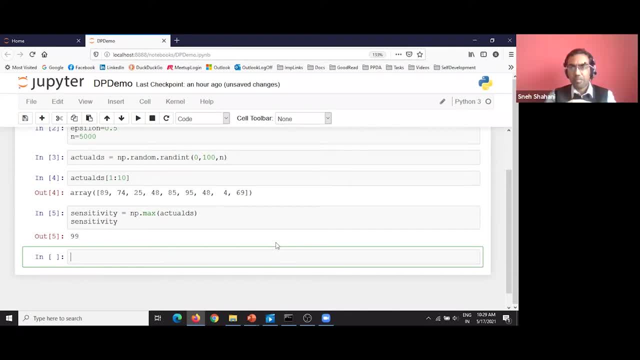 99 for our generated data set. so now we want to transform this data by adding laplace noise, so for. so we have studied a theorem just now that if we add laplace noise with mean 0 and scale parameter as sensitivity upon epsilon, then we get epsilon differential privacy. 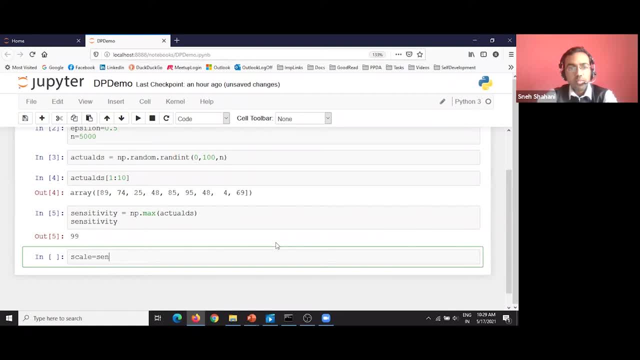 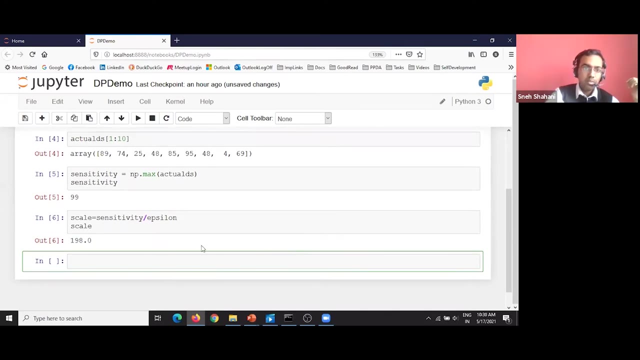 so scale parameter equal to sensitivity by epsilon. scale parameter is 190 in this case, because epsilon is 0.5 and sensitivity is 99.. so now we will compute that a transform data set that satisfies differential privacy perturb data set, we will call it as perturb data set. so we are adding noise perturbation to the 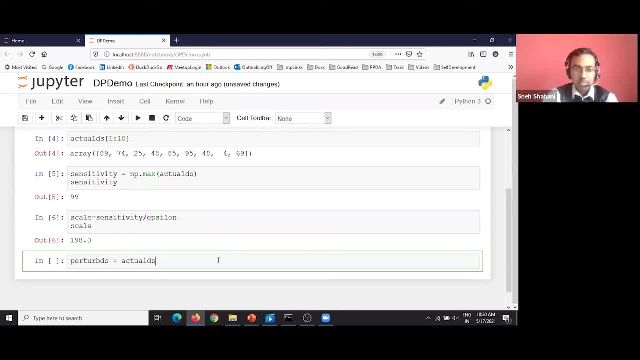 data set: perturb data set equal to actual data set plus numpy dot. random dot. laplace. so we are generating noise from laplace distribution with mean 0 scale parameter as scale that we have computed and n number of end points, n number of data points and we will print this data set. 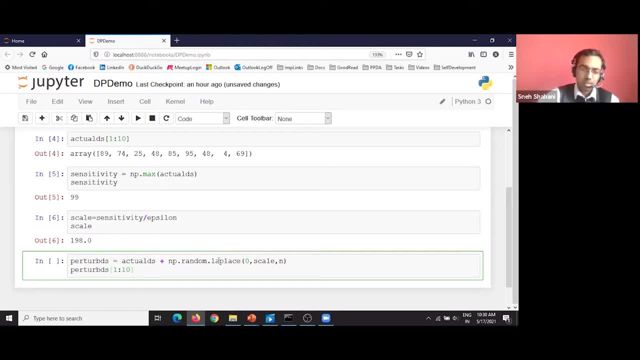 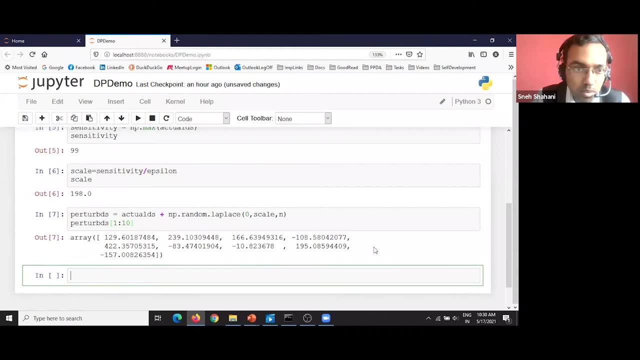 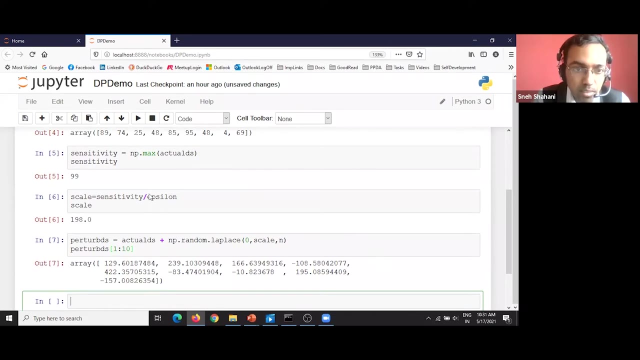 of 1, 200. first 10 values we will see. so this is the transformed value that we can see. so now we can see that first value here was 89, here it is 129.. second value, 74. in the actual data set when transform data set it is 239, like that it is say 166 minus 108. so looking at these values, we 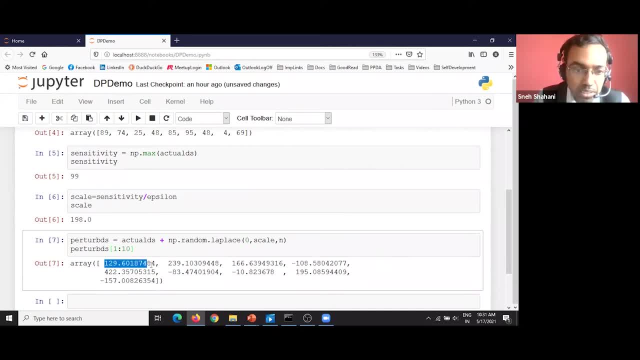 cannot identify that this value was actually 89, so we cannot identify the presence of value 95 just by looking at this transformed values. so now we can see that we can see that the value of the data set is 129.. So that's how we have protected the privacy of those individuals. 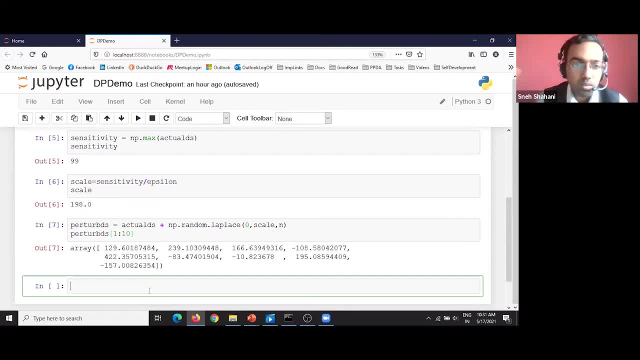 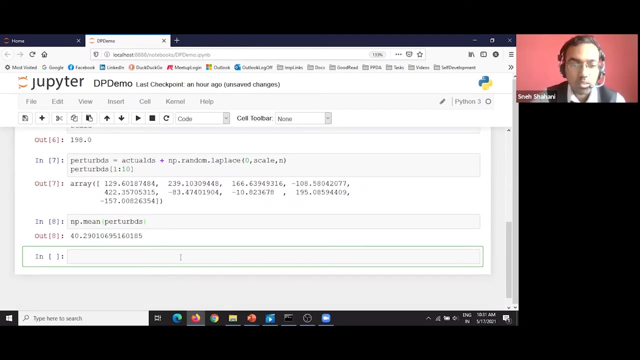 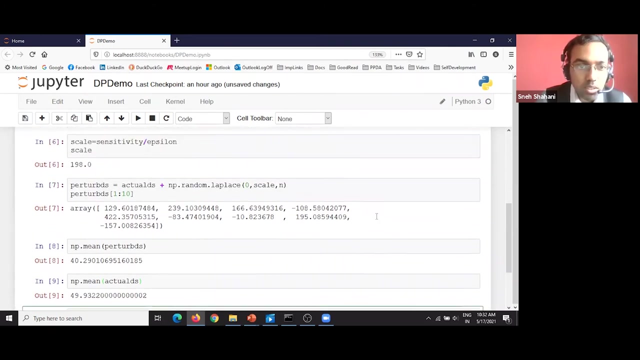 Now let us do some analysis on this data. We will compute mean of the data, numpymean of the transformed data set, that is 40. And mean of actual data set is 49. It is not that close to each other, but still it is useful for analysis. 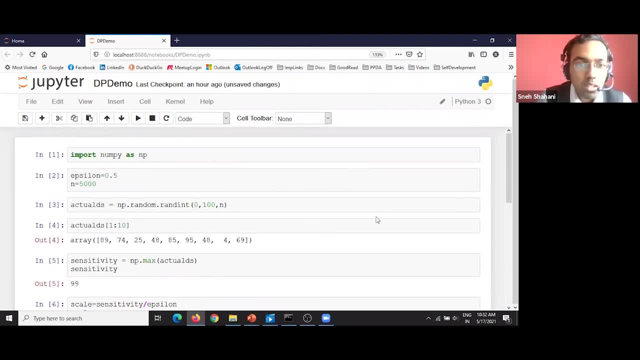 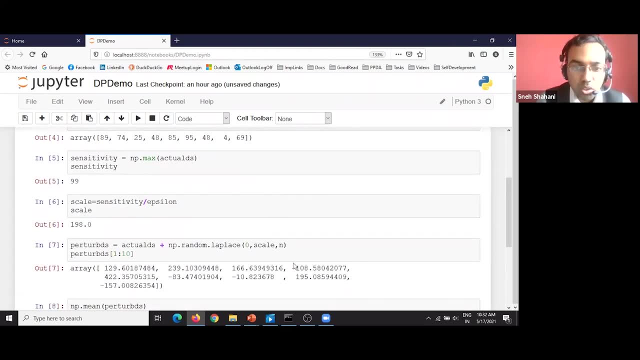 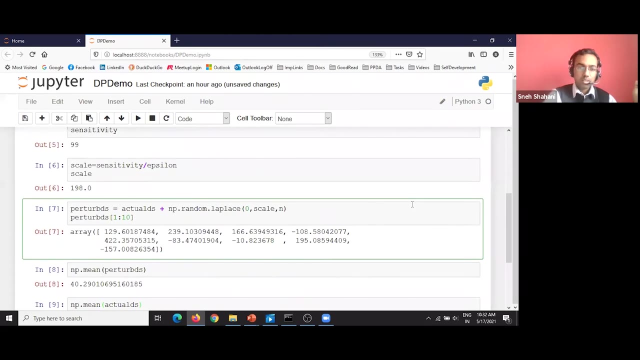 Let us see, let us generate this data set again. Many times, due to randomness, the randomness of the noise, the results are not very accurate. But when we have large number of data sets, the results are very accurate. So it is 43 and 49.. 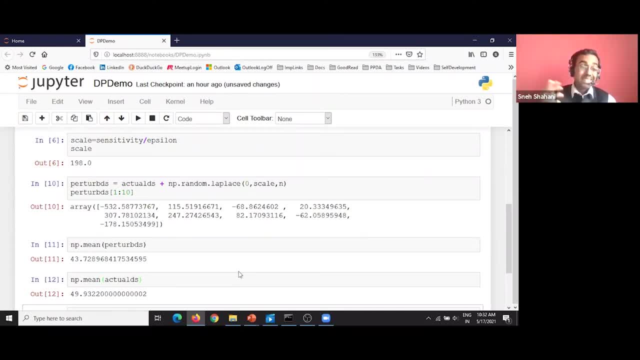 So like that you can check on your machine also. that mean computed from the transformed data, which protects the privacy of individual, is very close to the actual mean. So this shows that we can use the transformed data for our analysis and it will hurt the. 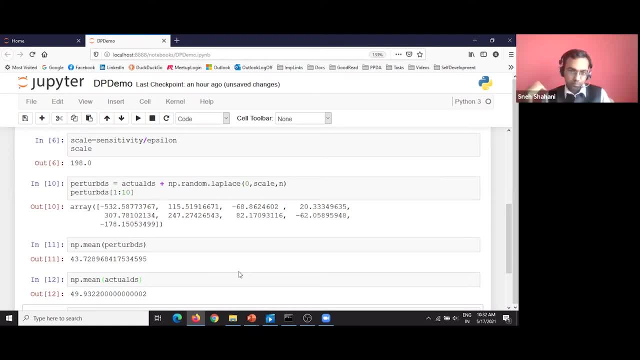 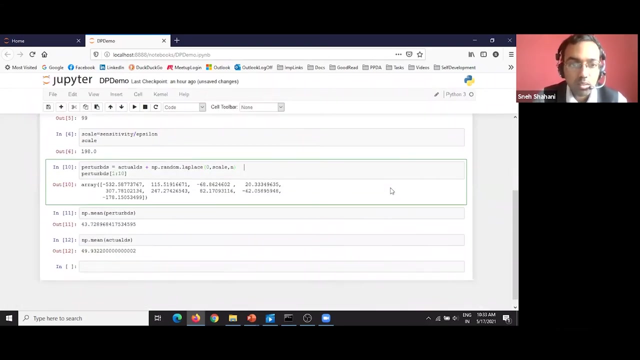 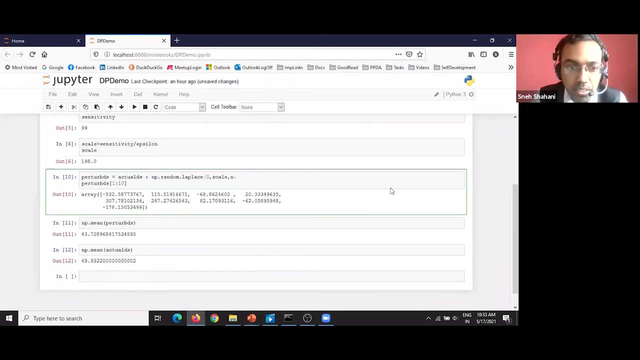 usefulness to some extent, But the privacy of individuals is protected. So there is a trade-off between usefulness and privacy, and we are ready to take some hit in usefulness while providing large amount of privacy to the individuals. So any doubt in this. were you able to follow this demonstration? 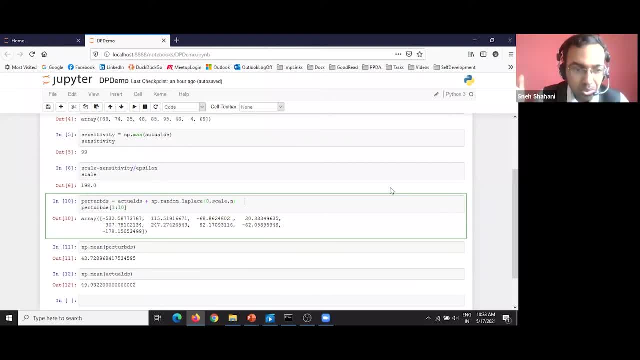 Did anybody get different values, very different values of mean, very much away from 49, the actual mean. So I would request everyone to share the mean of the perturbed data set, what you have computed. So let us see the kind of values that people are getting. 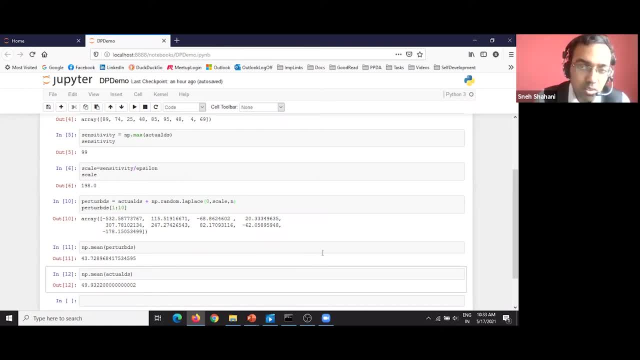 The actual mean is 49.9 or 50. So how different it is from 49.9?. That is what we want to see. So everyone who has done this experiment with us, please share the mean of the perturbed. 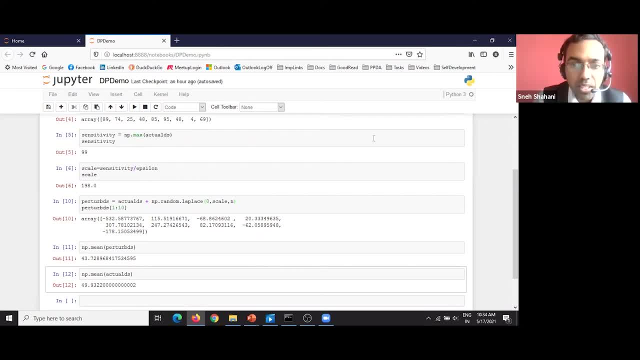 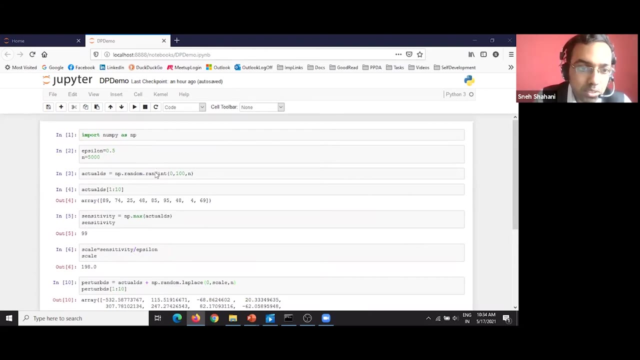 data set or transformed data set. Okay, So it is fairly close to 49 or 50, plus or minus 5, or plus or minus 7.. You can play with this data set. we are running out of time right now, but you can play with. 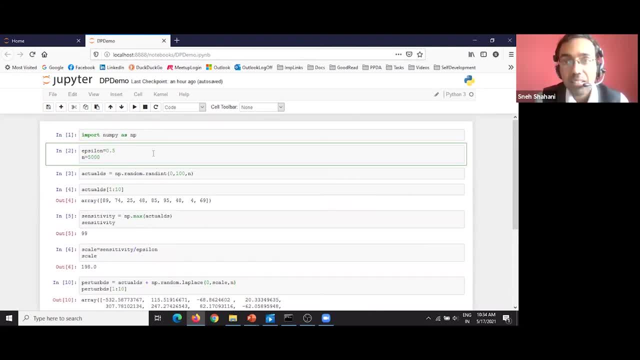 this data set by increasing the number of data points and see that. you will see that by increasing the number of data points, If you increase the number of data points, accuracy will improve. If you reduce the number of data points, accuracy will reduce, because what our objective is to 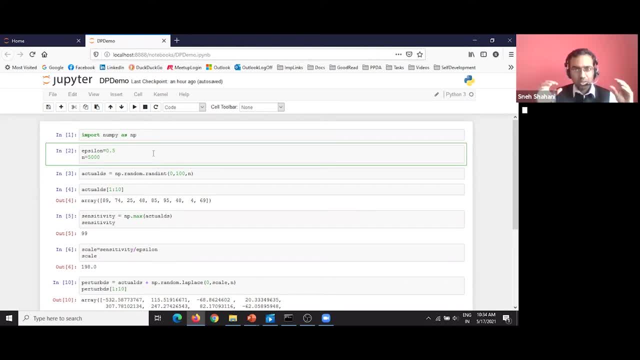 study the trends of the entire group and not of the individual. So if you have small group, then accuracy will take a hit, because we are providing more privacy to those individuals. Similarly, if the number of data points are more than, say, 10,000, then you will get high. 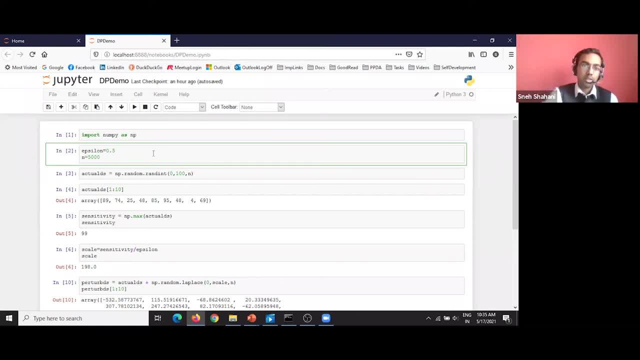 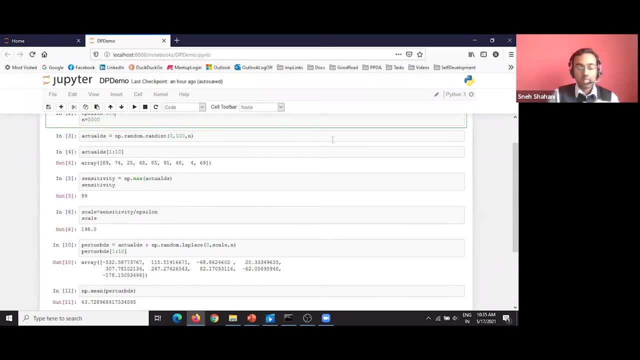 accuracy in that data set. And also you can vary the value of epsilon. Now that you have the notebook, chain the value of epsilon and play with the outcome and see, see. you can even say run a for loop and see by what happens to the graph as we change the value of epsilon from zero to. 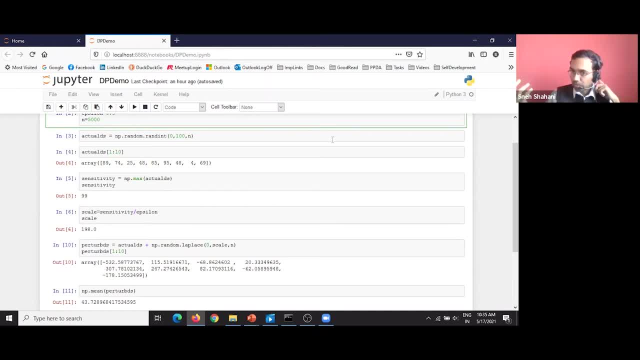 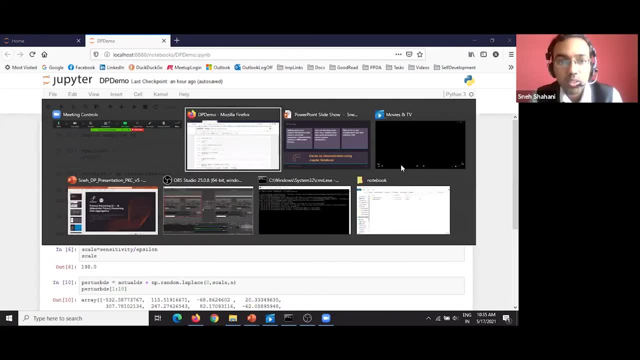 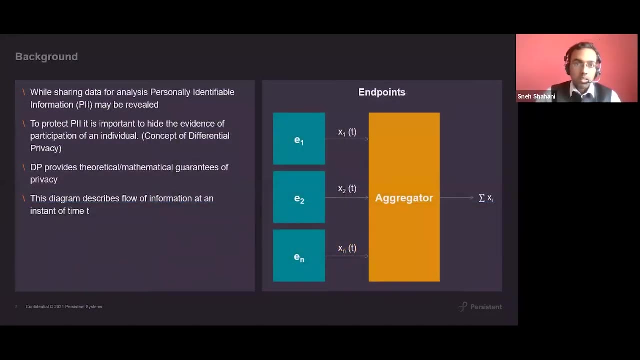 two with a jump of two: point one or point two. that kind of experiments you can do. so i hope you all enjoyed the demonstration. we'll come back to the presentation right now. so, while sharing data for analysis, personally identifiable in the information about individuals may be revealed, and to protect this pii, that is, to hide the evidence of participation. 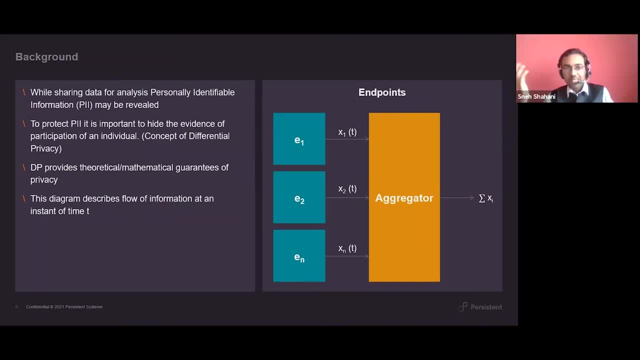 of an individual we provide. we use the concept of differential privacy. so there are various techniques of privacy, like k came sorry, i'm sorry. like histogram that hides the that groups everyone into the same set. we release the counts 0 to 10, 11 to 20, that kind of counts, and we release only. 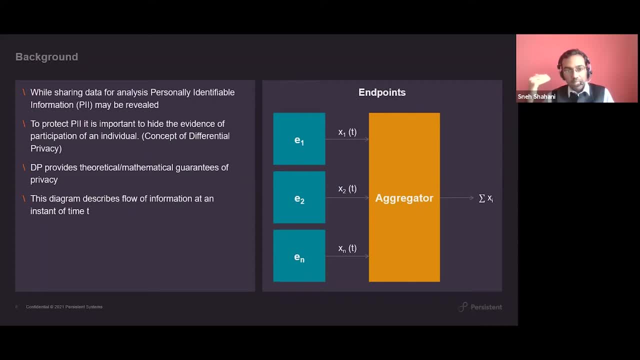 only the average of those values. and there are various other techniques where we release, say, only the limited amount of data, but differential privacy is very much different from them, because it provides mathematical and theoretical guarantees of privacy. you can calculate the probability of disclosure of that individual, which is not possible in other techniques of 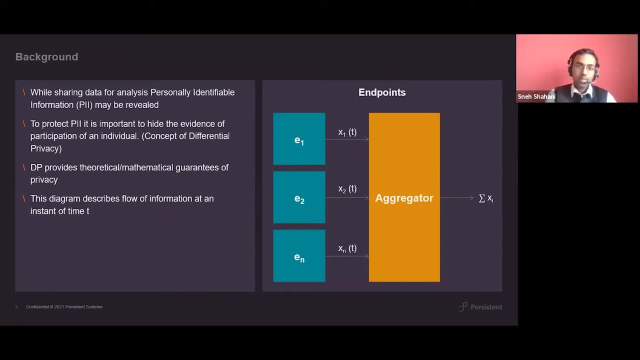 privacy. so let us have a look at this diagram. this is the block diagram that we will use throughout our study. are n, number of endpoints, e1 to en, and each endpoint has a value- x, xi at a time, instant t- and then there is an aggregator which wants to compute the sum of all those data points. 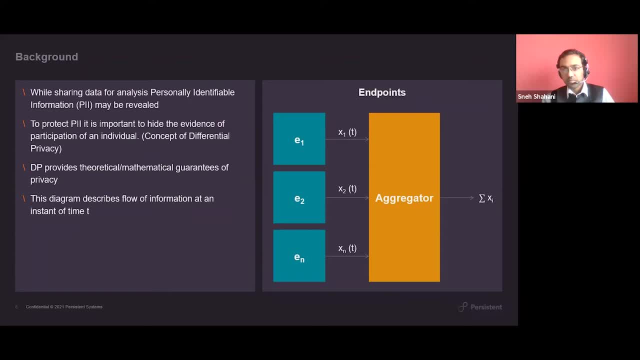 at a time, instant t. So aggregator should be able to compute the aggregate but not come to know about the individual values. That is what we want to achieve. Another example, for this is other than sum- is we are doing some federated learning In federated learning aggregator. 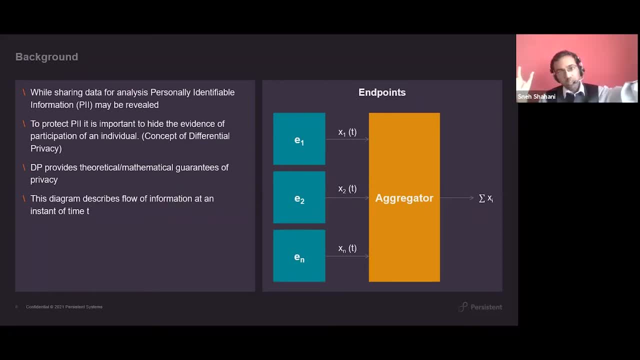 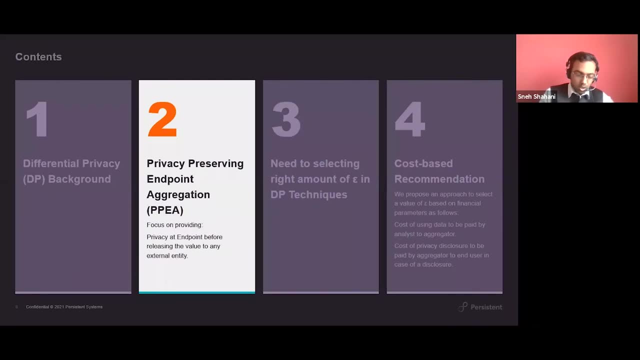 should be able to compute the final model but not come to know about the individual values of the endpoints. So we will understand this with an example of privacy preserving: endpoint e1 to en and each endpoint has a value x, xi at a time, instant t, So aggregator should be able to. 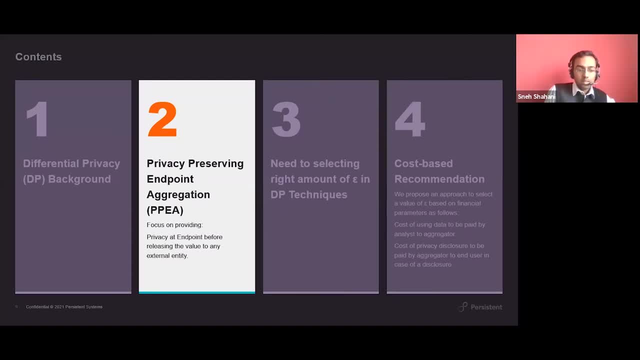 aggregation. So we have done a study of for some and we have designed a technique to satisfy some of the drawbacks of the existing techniques in the literature. So first part is privacy preserving, endpoint aggregation. So our objective is to protect the privacy at the endpoint itself before 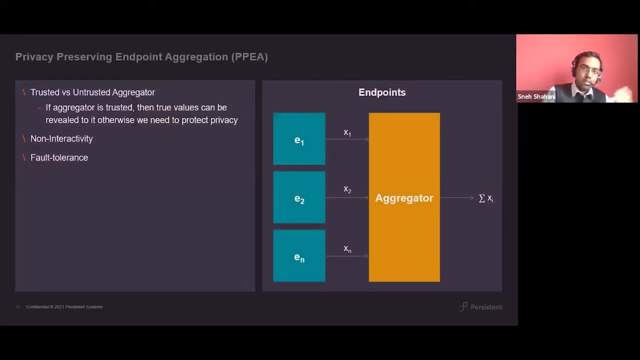 relating it to any external entity. So here in this block diagram you can see that there are, say, n endpoints. Each endpoint has a value x, and aggregator wants to compute the sum. The sum will be released for the analysis. The outcome of the analysis is sum only. So if aggregator is trusted, then we can. 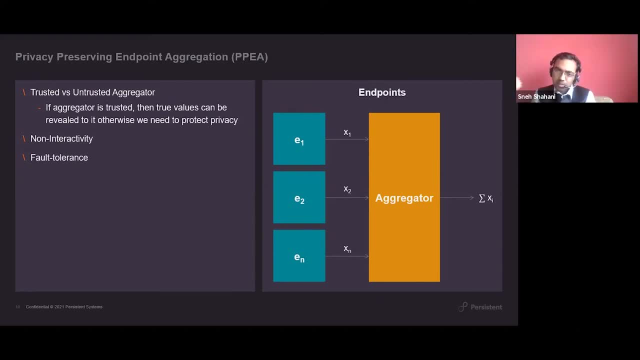 reveal the actual value to the aggregator, and aggregator will compute the sum and release only the sum. But what if aggregator is untrusted? Then we cannot reveal actual values to the aggregator. We have to do some, protect the privacy at the endpoint itself, And then there are other two limitations. So there are various techniques. 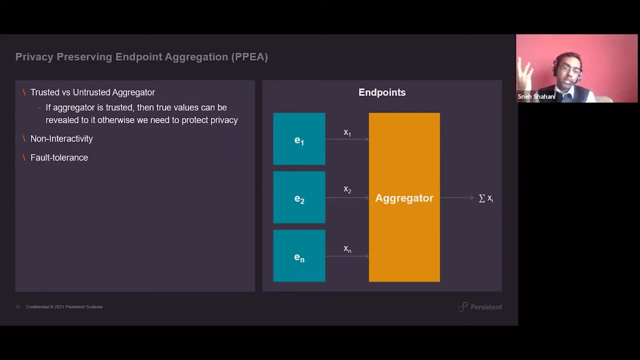 in literature that use this concept of symmetric multi-party or secure multi-party computation. Since secure multi-party computation there is a lot of to and fro communication but that ensures that aggregate is computed without a back up of knowing their individual values. But this requires a lot of. 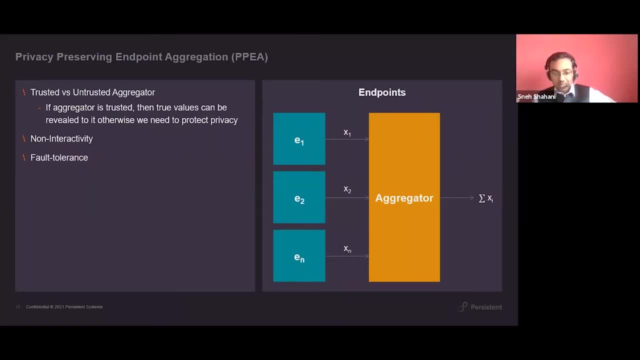 interactive communication, which may not be possible in various real life scenarios. Say, there is a mobile device that is revealing some data point, emitting some value to the server. In that case it may not be possible to set up a full network of devices that communicate with each other and then they transfer to some value. 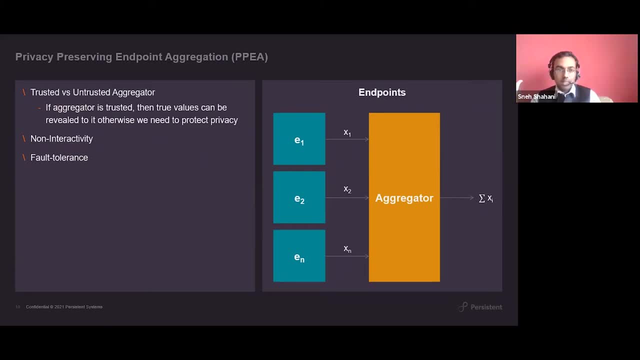 each other and then we'll come to know only the aggregate. so in this case we need non-interactive communication where the endpoint will reveal a value. endpoint can only emit the value and aggregator can only receive the value. other concept is there are some class of techniques. 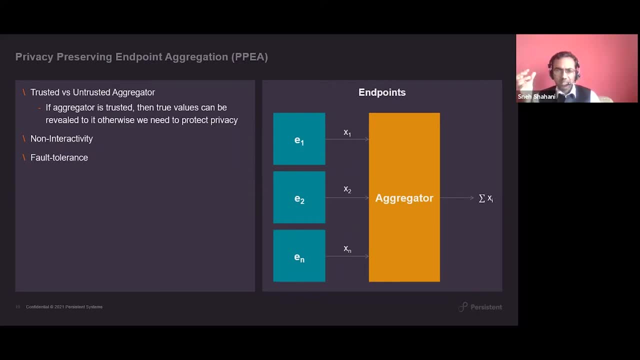 where they generate large random keys for each endpoint, and it is. they know that we are going to compute sum of only this 100 endpoints. so they will generate large keys for each endpoint in such a way that the sum of all those random keys is zero. so if each endpoint adds that large 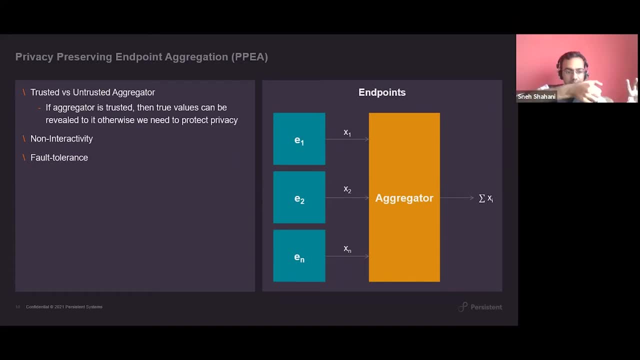 random value to the individual value xi and reveals that large value. we cannot identi identify the actual value from that large random value because what we see is a large random value only because actual data point is very small as compared to the large value. but when we compute the sum we get the actual. 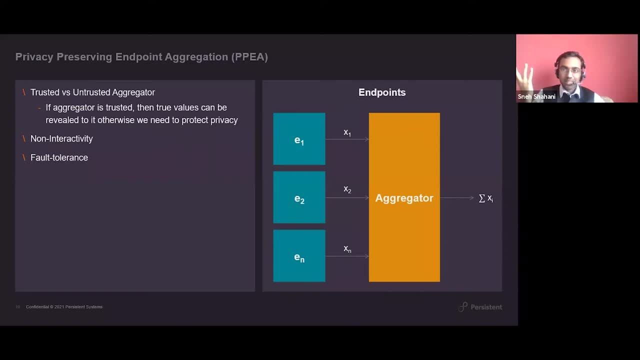 sum. however, there is a serious drawback in this case. say, if one particular endpoint fails to send the value, then we cannot compute the aggregate itself, because that large noise doesn't get cancelled. so just by a fault of one endpoint, aggregator was not able to compute the entire. 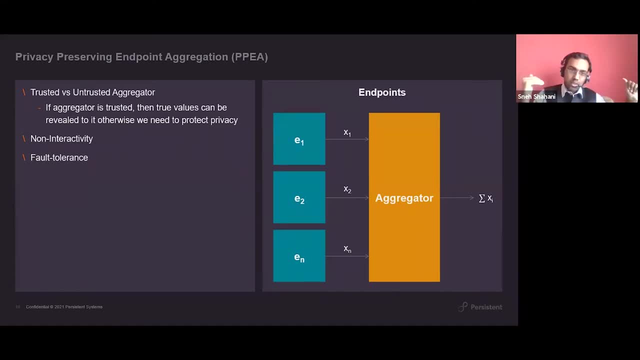 aggregate. so we need to design techniques that are fault tolerant say. fault tolerant in this case is when one data point falters to send the value. aggregator should be able to compute the aggregate of rest of the endpoints. if there are thousands of endpoints sending the value but at one iot device. 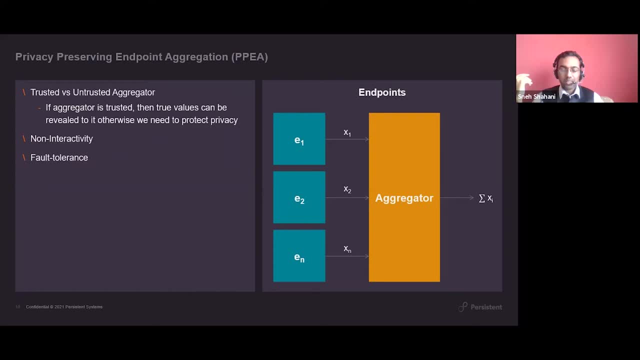 the power went off, the battery was faulty, so still we should be able to compute the aggregate for rest of the values. so this is known as fault tolerance. so we want to design a technique that works with untrusted aggregator, provides non-interactivity and is also fault tolerant. 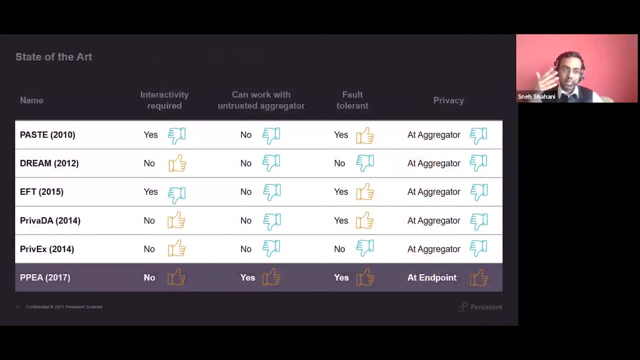 so we did a literature survey of some of the existing techniques in last decade and we identified that none of those techniques in literature- like pay stream, this enhanced fault, tolerant technique, priwada, privex- none of them just satisfy all these requirements: interactivity, ability to work. 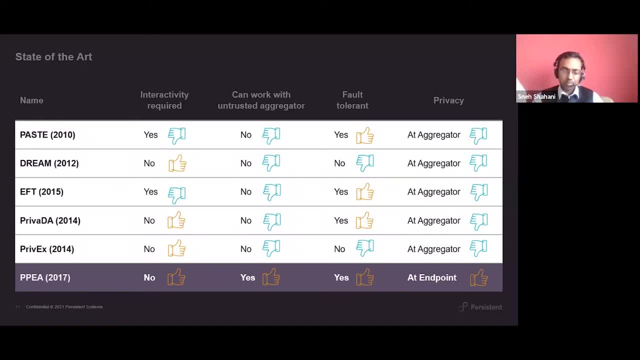 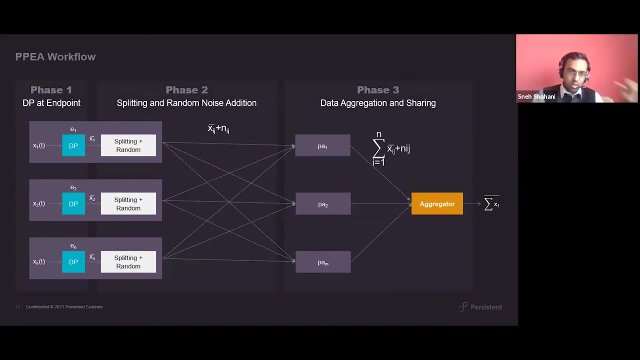 with untrusted aggregator and fault tolerance at the same time. so we designed a technique called ppea, that is, privacy preserving endpoint aggregation that satisfies all these requirements at the same time. so this is how we have done the design. sorry, so at any time, instant t, the endpoint device has a value x, x, i, and then it performs. 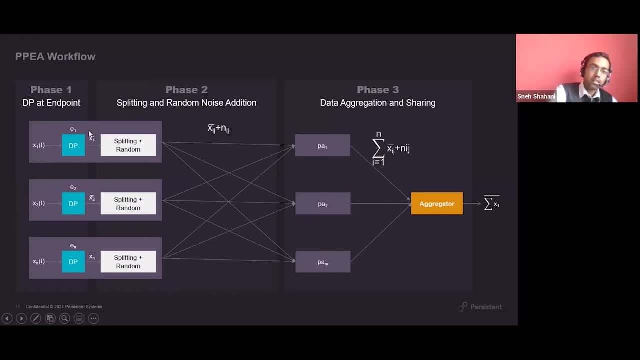 differentially private transformation on that value to get x i bar. so this ensures that that privacy is protected. now we will do some more steps to ensure security. so first we split the value into m, equal m parts, unequal parts- i'm sorry, i said equal parts, so each endpoint will split the. 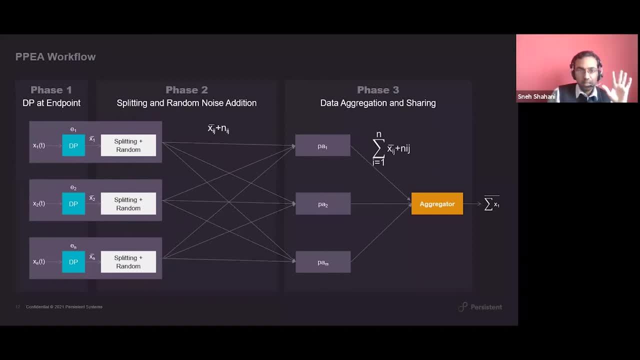 differentially paired value into m unequal parts randomly. and then okay, sorry, and then we add large random noise to this unequal part in such a way that these noises get many. noise is zero, so x1 is split into, say a case�도 and irgendwo involved members. 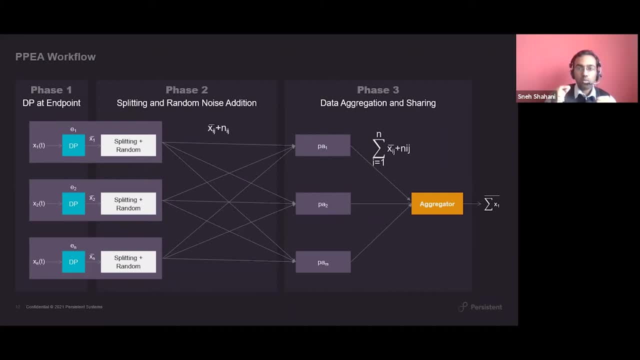 one is split into, say y one x one one x one, two to x one m, and then we add random noise, n one m n one one, n one two to n one m, such a way that sum of this n one m is zero, while sum of this x. 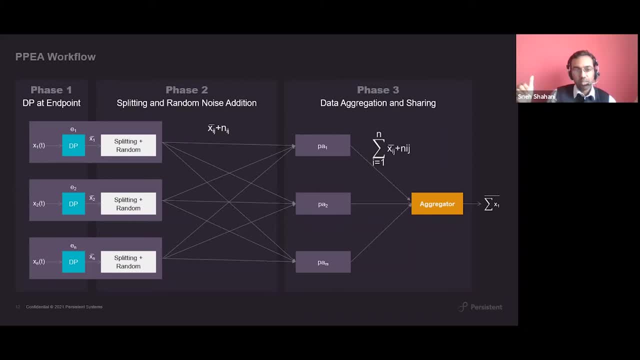 one, j is x one and these values are sent to this partial aggregator. so each data point will end point, will transfer, do this kind of transformation and send the value to the partial aggregator. partial aggregator will complete the partial aggregate and then send the partial aggregates. all the partial aggregators will send partial aggregate to. 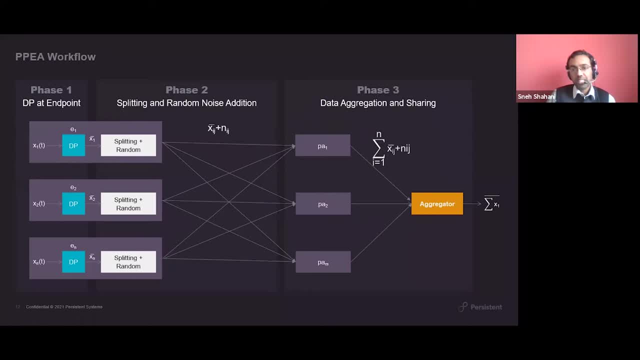 the aggregator and then aggregator will be able to compute the final aggregate using this, all these partial aggregates. sam, your quick question. maybe you can answer yes, yes, whenever you you get a chance. yeah, by splitting the value into uh, the same x into n values have. now will the uh. 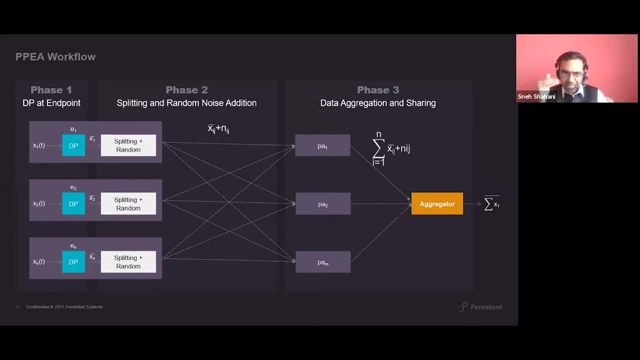 error be, uh, very different. this splitting does not affect the error at all. this is just to ensure that there is a concept called aggregator obliviousness. aggregator obliviousness means aggregator should be able to compute only the aggregate and not the individual value. so by splitting this and then combining this at the aggregator, we ensure that the 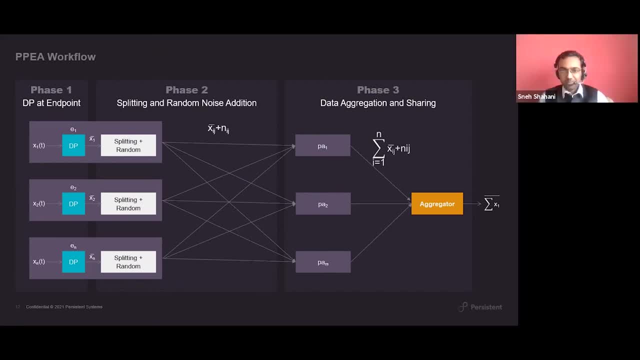 aggregate is same but, uh, individual values are not known to the aggregator. this step of splitting and random know that addition does not affect the usefulness, only there's differential privacy, the small noise that we are adding to the before splitting and random noise addition. that is what affects the usefulness. 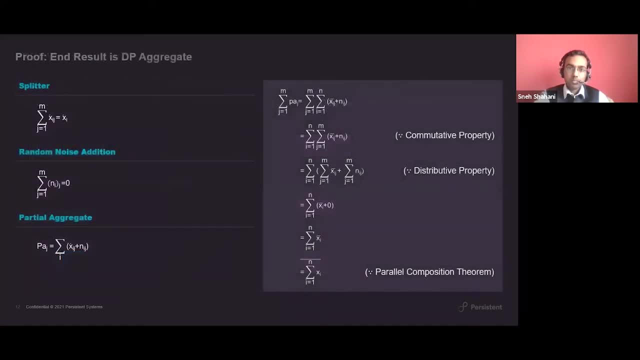 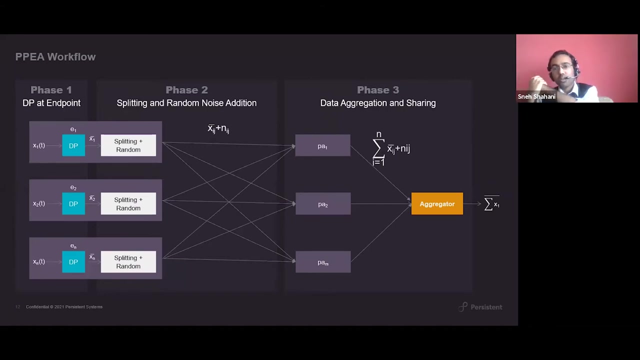 yeah, thank you. okay, thank you, thank you for asking this question actually. so this brings me to another point, another concept called aggregator obliviousness. so the aggregator obliviousness is also a way to protect the privacy of individuals in federated learning. what we do is we provide aggregator obliviousness. 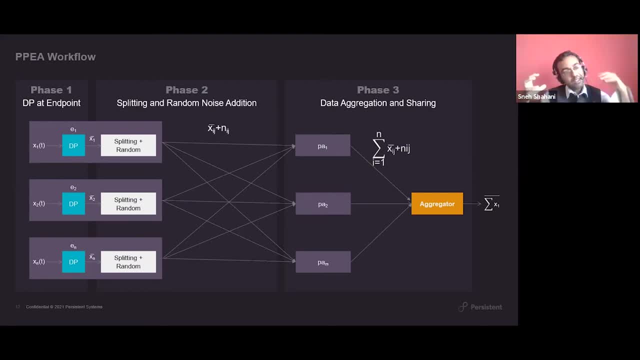 means the aggregator or the final model. uh is computed without knowing the individual values, but it does not protect the privacy of the individual theoretically. so it is very difficult to identify individuals from that individual federated models. but still theoretically it is possible. and there are some attacks like model inversion attacks or mi attacks. that can be employed to predict the presence of individuals of a certain scale when the model is試ed didn't work for them. that can be employed to predict the presence of individuals of a certain scale when the model is試ed didn't work for them. 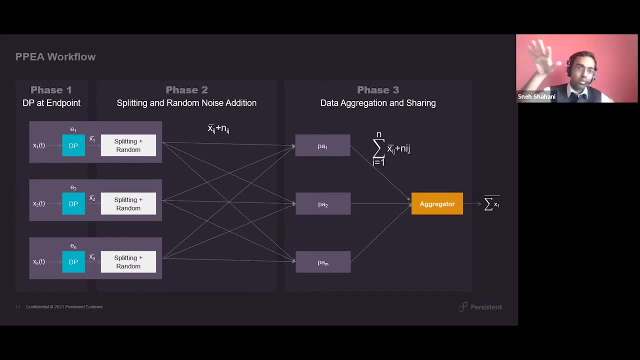 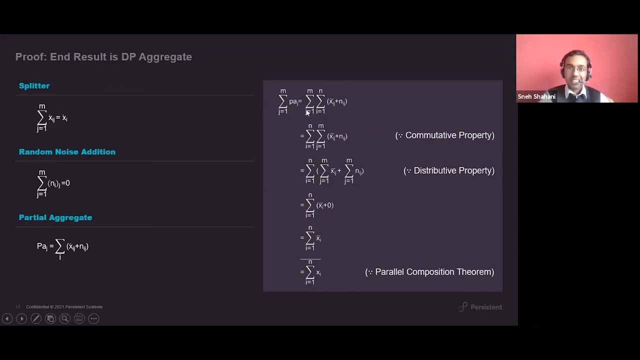 usual in that data set. so in order to protect that kind, in that kind of scenario, we, in addition to aggregator obliviousness, we also use differential privacy, and so in predated learning also, differential privacy is very useful. so we will come to that. okay, so in this work on ppea we have proved- we will first prove- that some of this partial 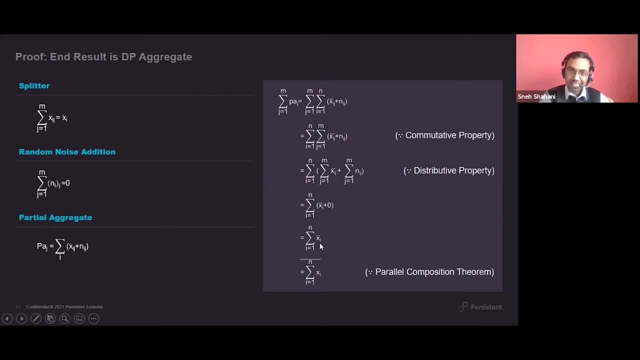 aggregate is actually the aggregate of the uh differentially private value. so it is all. it can also be considered as differentially private aggregate. this is proved in our paper and i will encourage everyone to have a look at the detailed proof in the paper in. In addition, we have also proved that in case of a fault, say one value is missing and still we can compute the sum of the rest of the values, n-1 values. 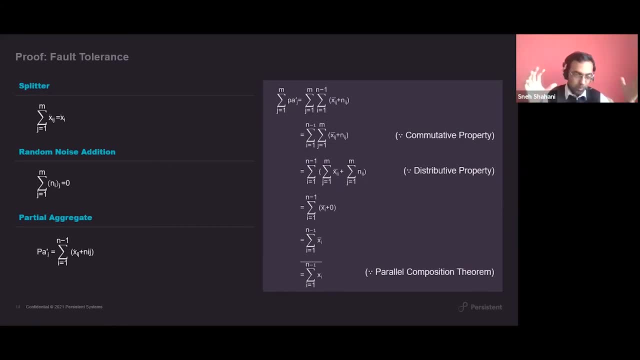 So we have proved that aggregate computed using PPA is differentially private as well as fault tolerant. These two things we have shown mathematically. So now we are happy that we have provided privacy, But still now the question is about the usefulness of the data. 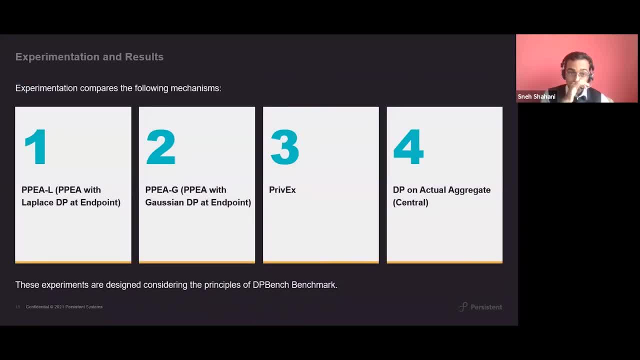 Now we will measure the usefulness experimentally. So we have designed two variants of PPA, that is PPA-L, that is PPA with Laplace noise, and PPA-G, that is PPA with Gaussian noise. And then we have compared these two techniques with Prevex, one of the existing techniques in literature. 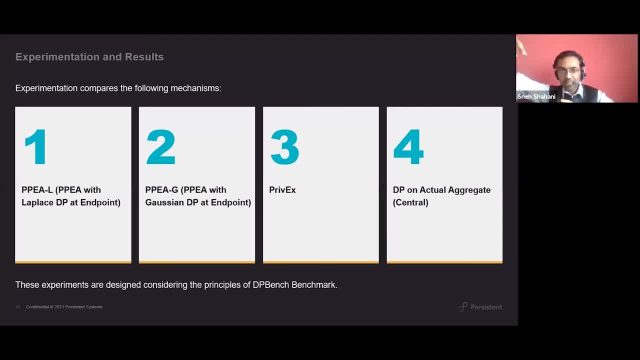 And also we have compared this. So we have compared the two variants of PPA, with differential privacy on the actual aggregate. So instead of providing protection at the endpoint, we use trusted aggregator and we add noise to the aggregate only. This is the least amount of noise that we can add. 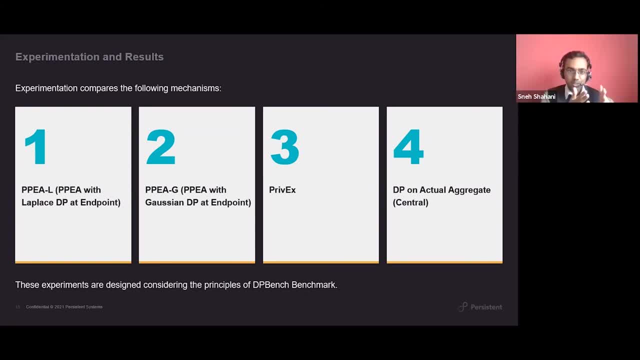 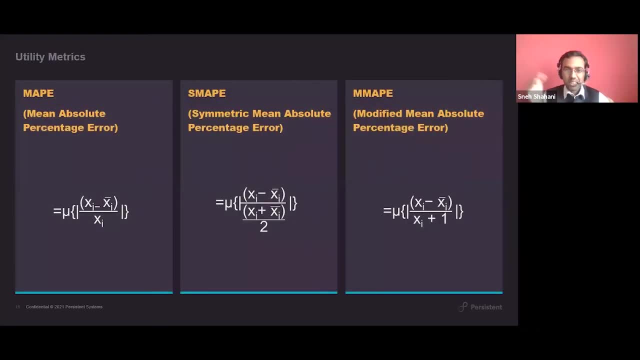 And we get very high utility in this case. but we do not protect the privacy. But still, for the sake of experimentation, we are comparing this with the ideal use case. also, We are using three measures of utility. First one is MAPE. 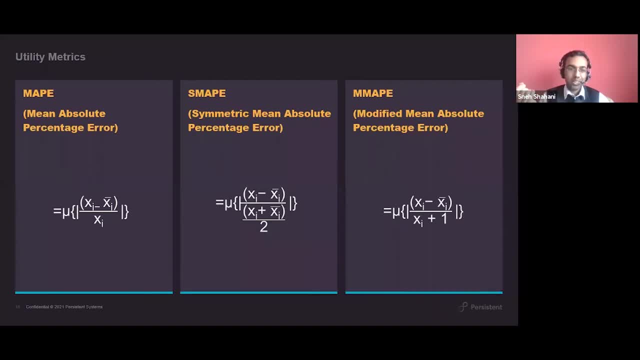 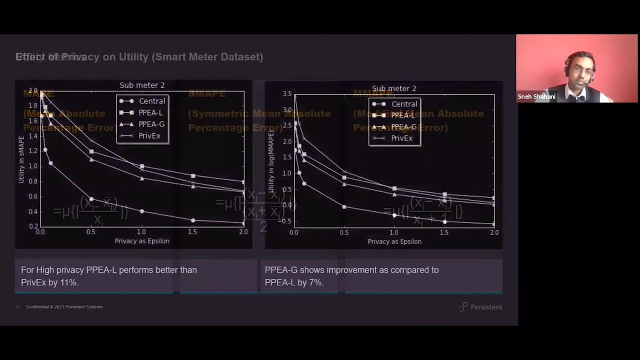 The mean absolute percentage error. It has some problems that for zero value data data points with zero value, we cannot measure MAPE. So we use two variants: symmetric mean absolute percentage error and a modified mean value percentage error where we add some constant value to the denominator. 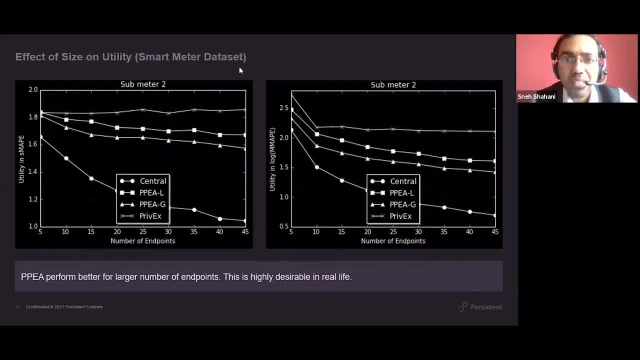 Are you able to see the title? Hide this? OK, So first we study the effect Of size or number of endpoints on the usefulness. So what? we observe? that as we increase the number of data points or number of endpoints, the usefulness improves. for all the techniques. 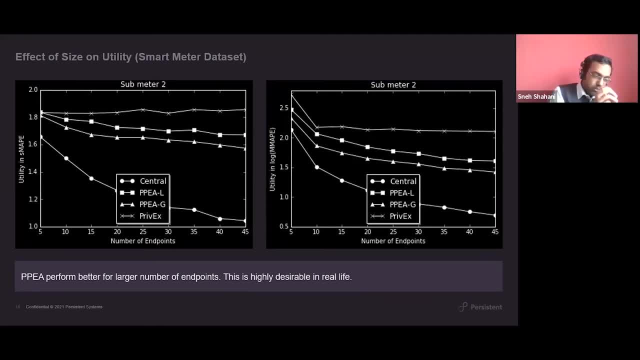 So there is a benchmark paper called DP Bench, where they have designed, described the set of experiments to be performed for any new differentially private technique. So first they are advised to study the effect of size or the impact of varying the number of data points. 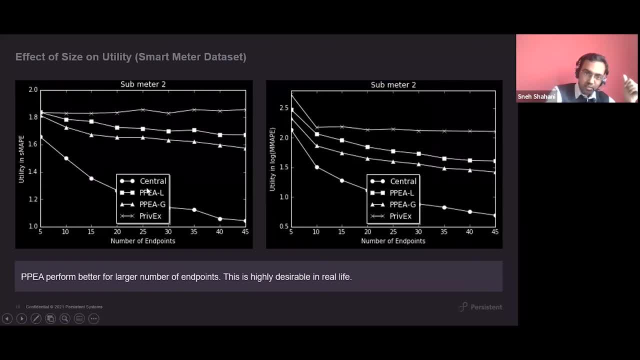 So as we increase the number of data point, the express error reduces on usefulness into it. So what you are- this is the bottom most line- is the central privacy or the ideal use case and our all of the techniques that works in the ideal use case. 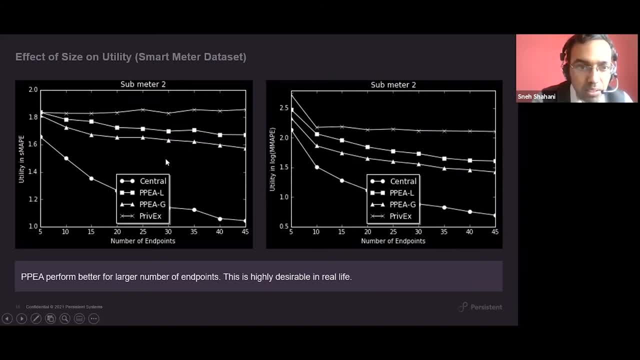 So what we absorbed from our experiments is that PPA performs better For large number of data points, Other numbers of earthquakes, For large number of data points, Other numbers of maiden conditions. If we see this, then the virus may Chinese of recent data, occur. cases or even all the population could be injured, as ETS. 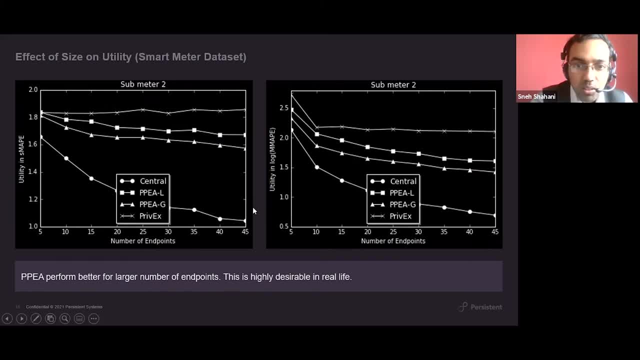 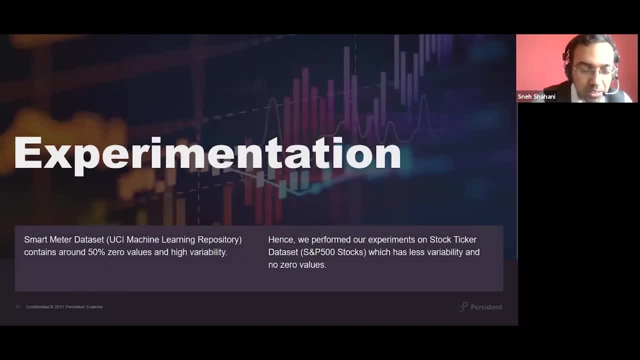 points. the number of endpoints are very large, which is ideal use case, and we have performed our experiments on this uh uci machine learning data set, that is, smart meter data set. and then there is another data set called stock ticker data set. stock ticker data set we have selected 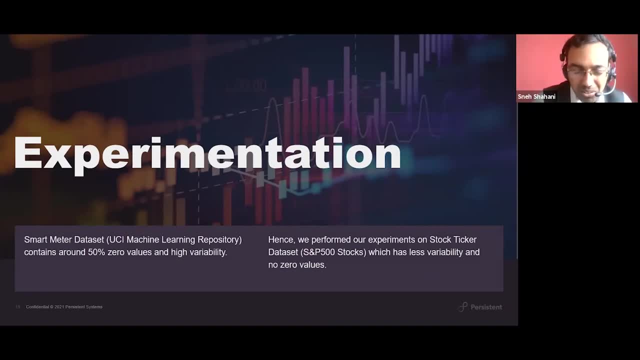 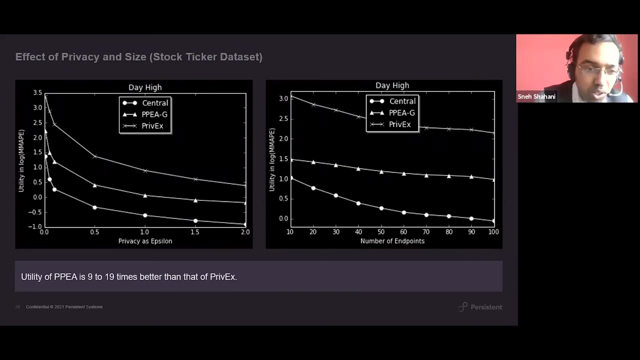 because it has no zero values and it has less variability. so to study it doesn't need any kind of privacy. but to study the impact on that kind of data we have used tactical data set. the second effect that we study is the effect of varying the epsilon. so as we increase the epsilon, 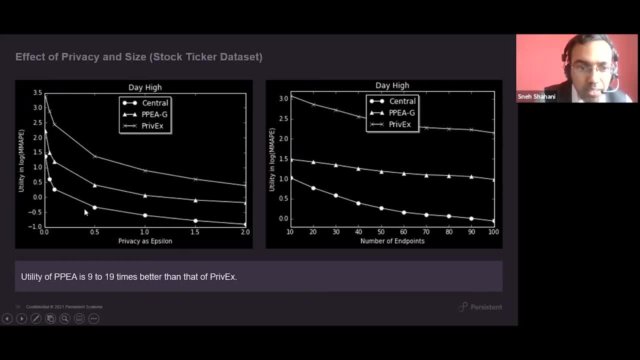 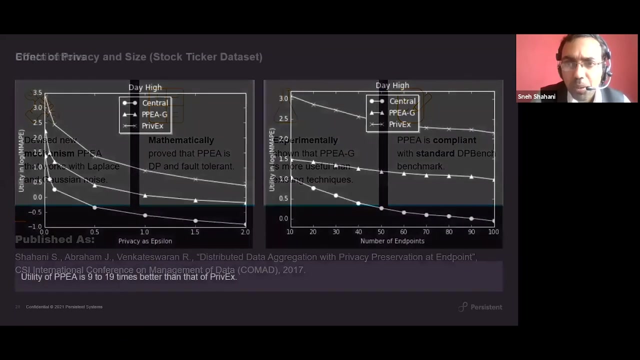 that is, we are reducing the privacy. the impact on the usefulness is also improved and what we have observed is our technique ppa is better than existing technique privets. it is around 9 to 19 times better than px. and another observation that is not seen in this experiment is that 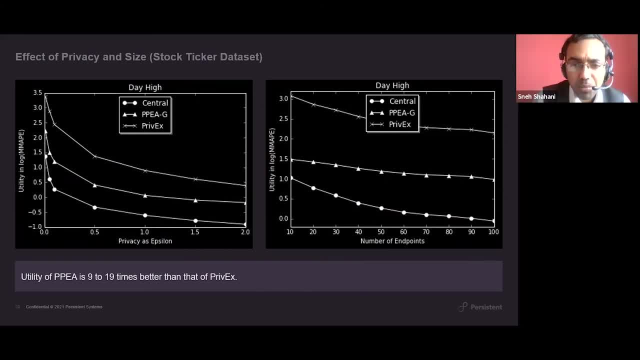 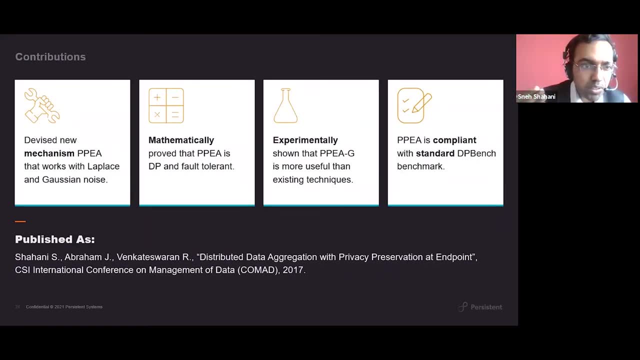 ppa with gaussian is better than ppa with laplace. so what is the outcome of this research is we have designed a new mechanism, ppa, that works with laplace and gaussian noise. we have mathematically proved that ppa is differentially private and fault tolerant, and we have shown that ppa is more than the 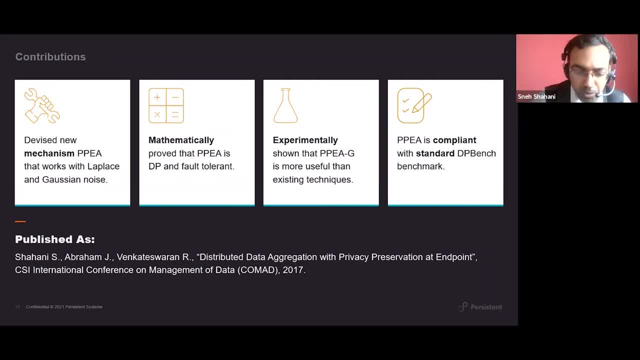 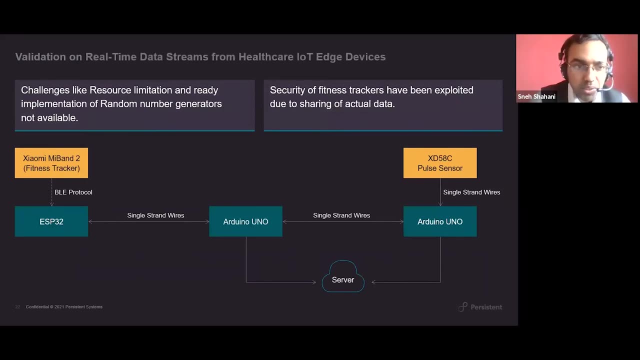 existing techniques and it is compliant with dpbench benchmark. okay, we have to go quickly now. we have a lot more to cover. so, in addition to this, we have also validated this technique on a real-time scenario on xiaomi's fitness tracker, and there is another pulse sensor called ocup98c. so both of them. 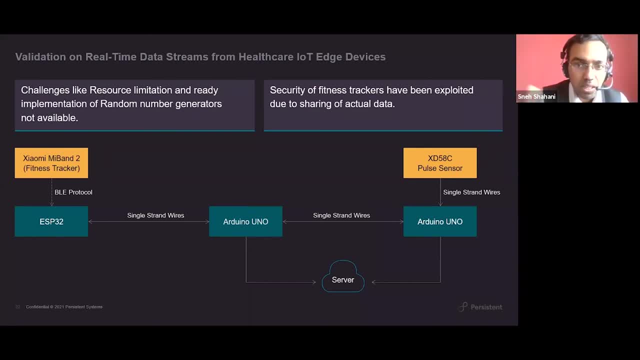 measure pulse rate or heart rate. so heart rate and pulse rate are very similar and I am talking about 10 million data cell powered sound environment data structure, as you can how this comes from. this real-time zienario on XAOMI fitness tracker is Veri, northern federsey, and there are process ofр. 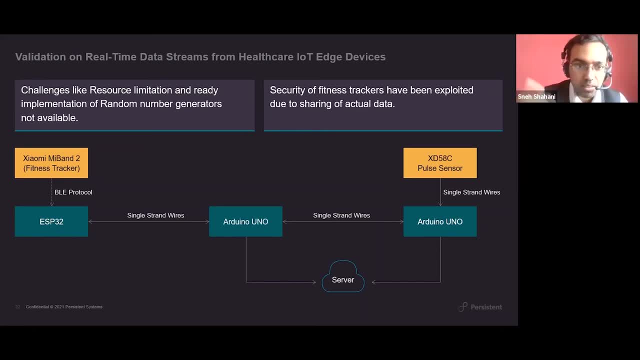 are same things measured using different techniques, through pulse and through other techniques. so in order to implement this technique on this low-end devices like arduino board- there are some challenges on these devices that ready-made implementation of this random number generators is not available. so we, in order to implement, we had to first design those random number. 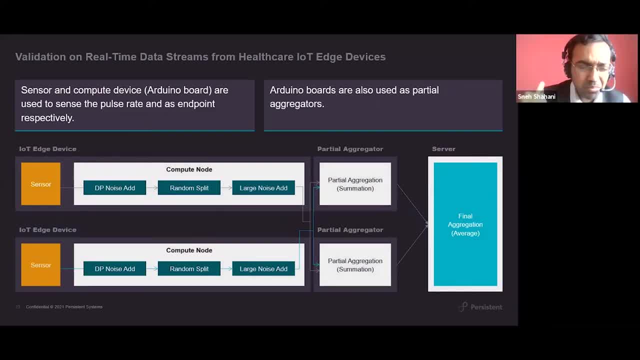 generators by using this box miller transformation, and then we have implemented our partial aggregators as well as this dp noise addition, random splitting and large noise addition on the arduino board itself. when arduino board was, it's also used as a partial aggregator also, and final aggregate that we computed was average. 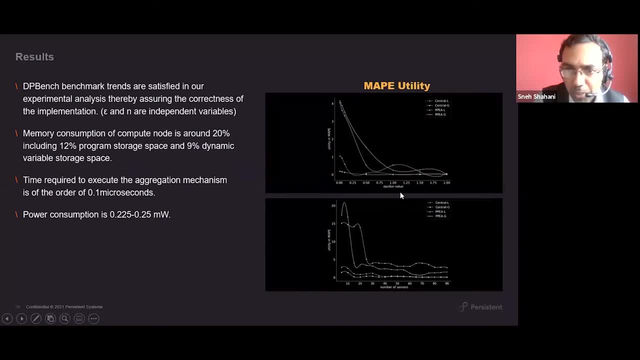 so first we validated the impact of epsilon and number of sensors and we found that they follow the dp bench trends, that we have observed the theoretical trends. this ensures that our implementation is correct. so, after ensuring that our implementation is correct, now we validate whether it is actually useful or not, the memory consumption, time required and power consumption. 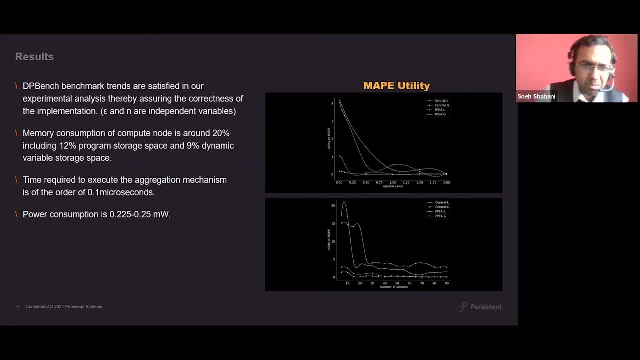 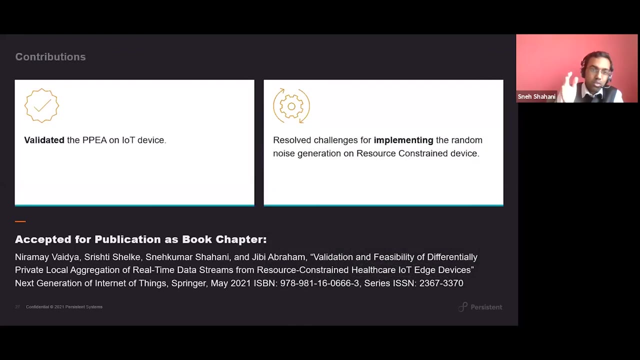 these are some some of the parameters that we have measured. so memory consumption is less than 20 percent and time required to execute is also 0.1 microseconds. so these are some of the numbers that show that it is actually implementable and practically useful on this kind of iot devices. so what we have done, we have basically validated ppa on iot device. 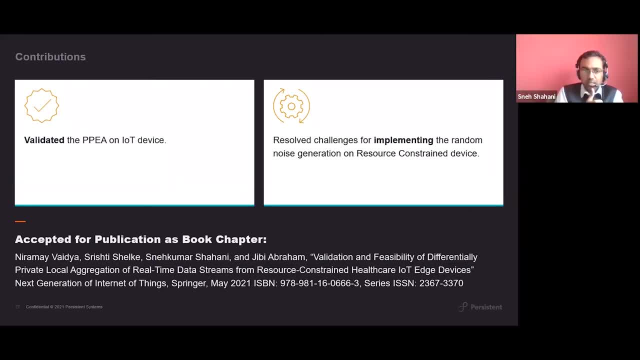 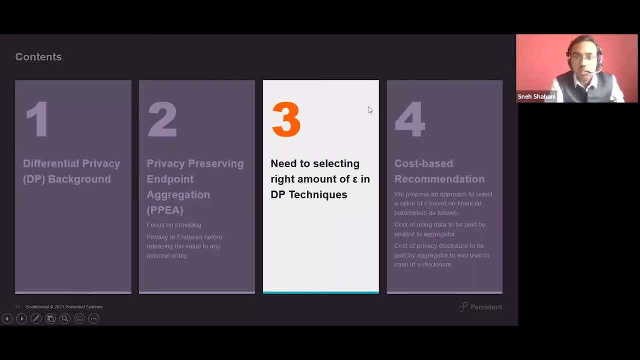 and resolved some of the challenges of implementing random noise generation, so this has been accepted as a book chapter in next generation iot. okay, let me start with the session now. so now we come to a very important aspect of this differentially private technique. so till now we described one of the techniques of differential 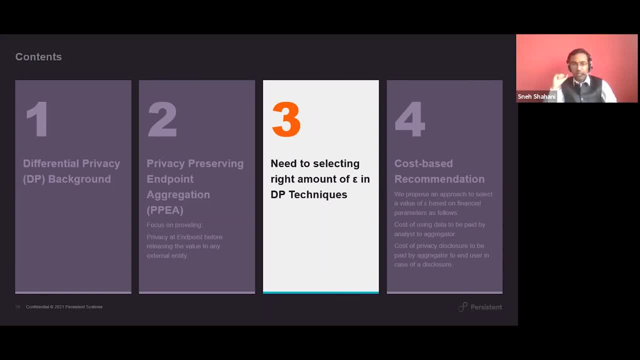 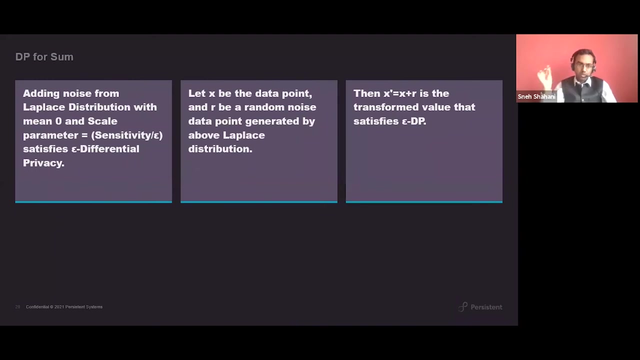 privacy. we understood some of the concepts of differential privacy. now we are going to discuss a serious limitation in the existing literature about. in order to practically implement this differentially private technique is the limitation is to select the right value of epsilon. so we know that adding noise from laplace distribution with mean 0 and scale parameter sensitivity by epsilon. 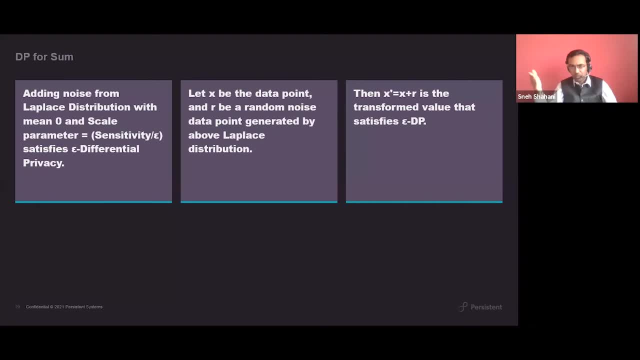 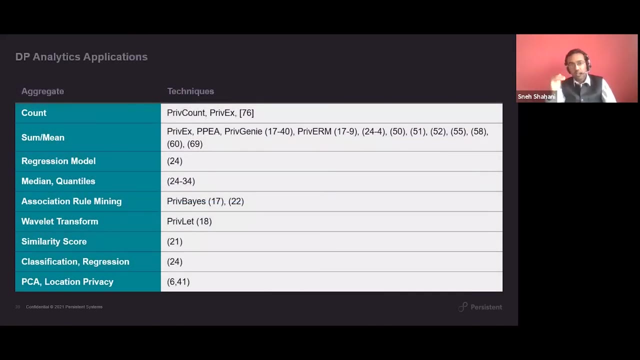 satisfies epsilon differential privacy and we even saw hands-on demonstration of how the transform data set can be used for computing sum and mean like this. there are other differentially private techniques for count, sum mean, even for regression model, medians and other quantiles: association rule, mining, wavelength, transform, similarity score. 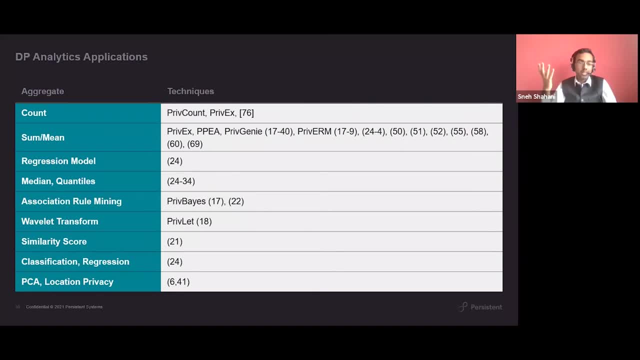 classification and regression, principal component analysis and there are other techniques for location privacy. this is a literature survey of last decade. but one common issue in all these research papers is that none of them they provide a way to select the right value of epsilon. they do not recommend a value of epsilon that should be used. 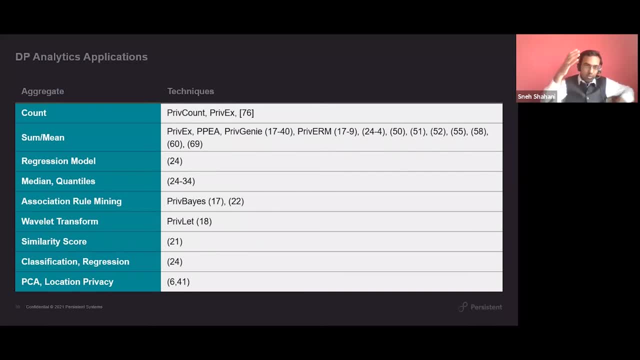 they all follow this tp bench trends, like by varying a value of epsilon, what happens by varying the number of endpoint? for what is the impact on the outcome, and then for the purpose of experiment, some of them, they select value as 0.1. epsilon equal to 0.1. epsilon equal to 0.01. 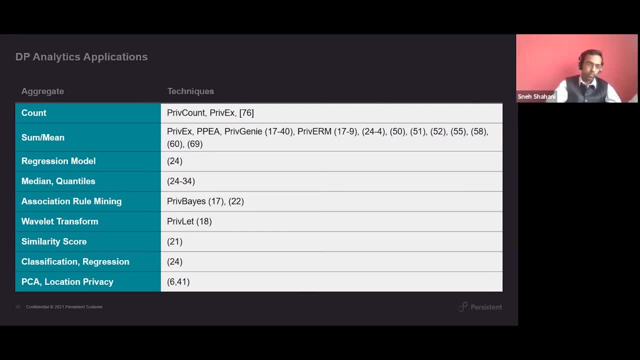 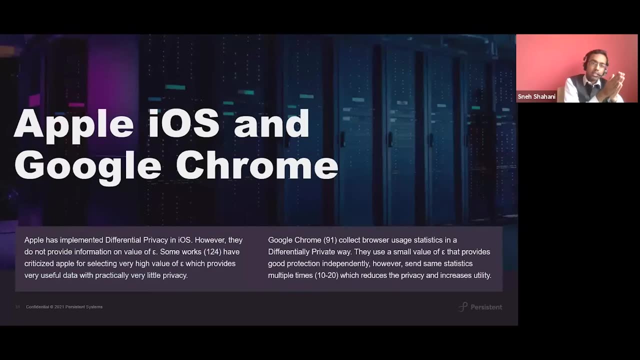 and then they study the outcome for a fixed value. but not selecting a value of epsilon has some problems. let me give you an example that in last two years- back around two, three years back- apple did a lot of publicity that they have implemented differential privacy in ios. 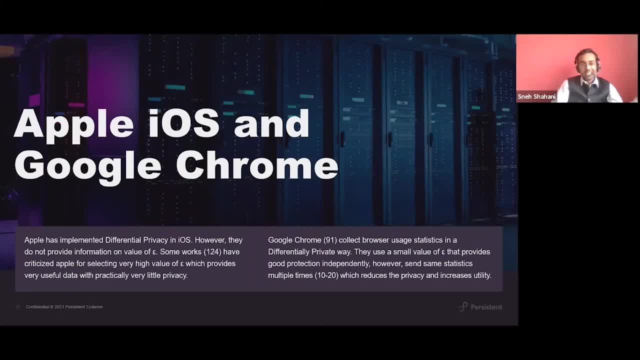 however, they have not provided the value of epsilon that they select. and then there is a research paper which has criticized it and they have not provided the value of epsilon. and then there is a research paper which has criticized it and they have not provided the value of. 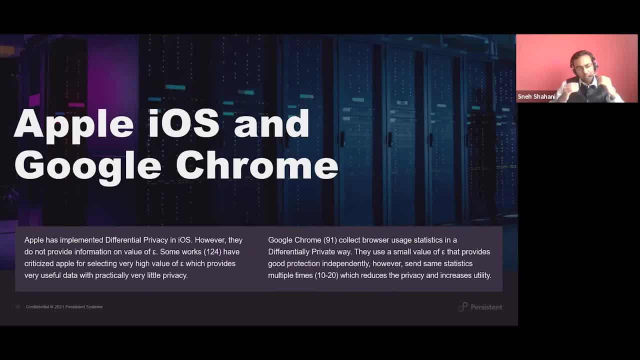 apple for selecting a very high value of epsilon. that provides very useful data and practically very little privacy. similarly, google chrome also has a technique called rapport that they have implemented to collect this browser statistics in a differential priority. they have used a good small value of epsilon, but they use some other techniques like this: send the same value 10 to 20. 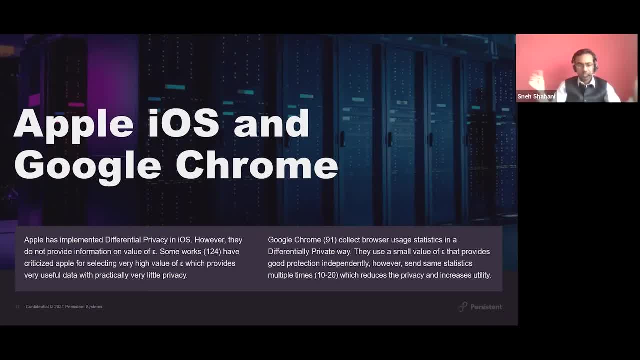 times. you know, in some different way of measurement. say somebody, something is kilogram, they send the same value in grams and then they will change the name and, like that, they send that same value 20, 30 times. this also reduces the privacy and increases the utility. 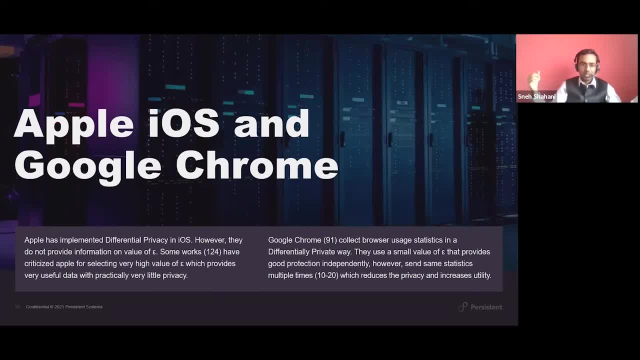 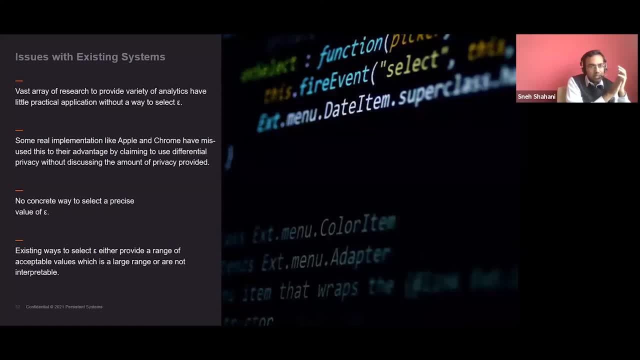 so these are the side tricks that they have used in apple and google chrome. so what we saw till now is that there are- there is a vast area of research done to design differentially private techniques for variety of outcomes, like some count, mean, quantiles, etc. but but there is no. these techniques have very little practical application without having a way. 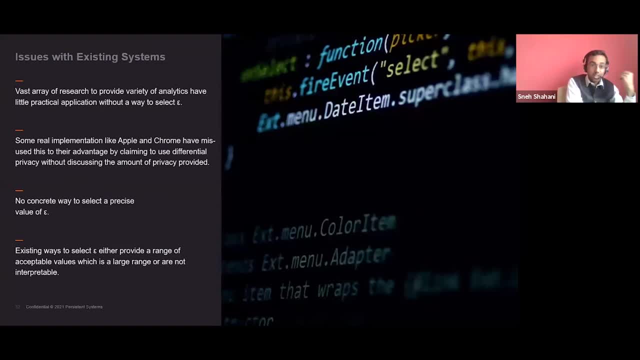 to select epsilon, and some real implementers of dp, like apple and chrome, have misused this to their advantage. all this is due to the same reason that there is no concrete way to select a precise value of epsilon. there are some existing works that select epsilon. they provide range of acceptable values, but sometimes 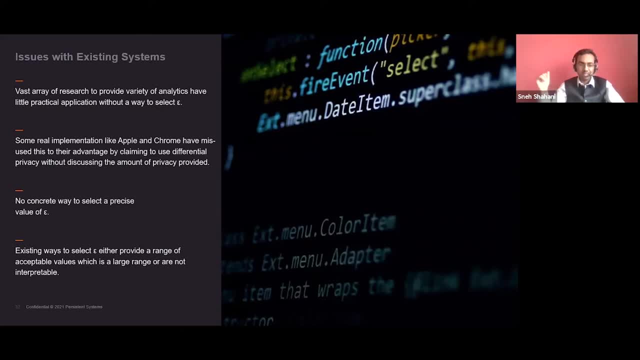 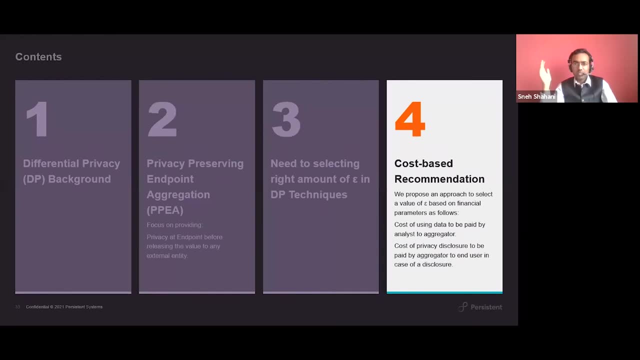 many times these ranges are very large and they are not practically interpretable. so what we have come up with is a cost-based technique to select, recommend a value of epsilon. so we consider two costs: cost to be paid, cost of using the data, to be paid by analyst to the 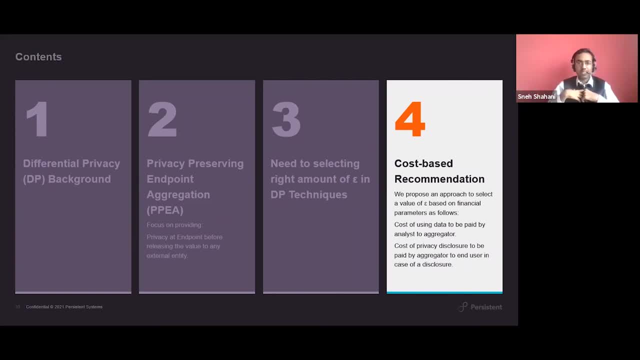 aggregator say we are the aggregator and somebody is going to use the data. so cost of using the data needs to be paid to us and we have to acquire the data from individual people. so by acquiring the data using any value of epsilon some, there is some cost to be paid to us. 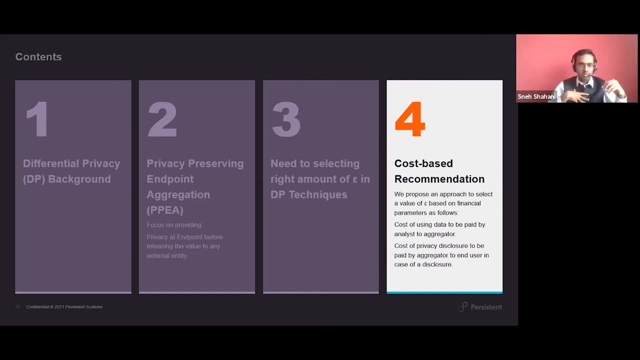 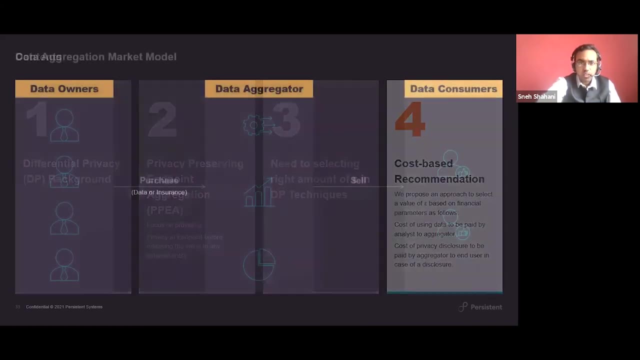 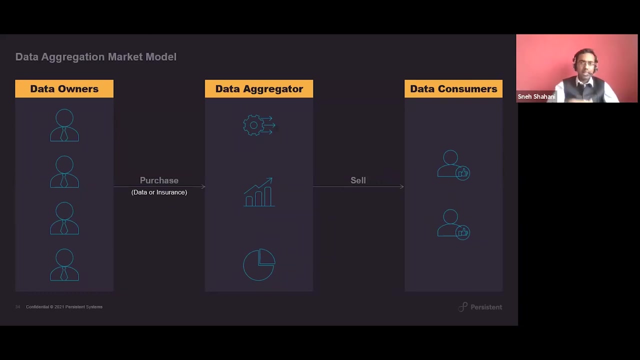 probability of disclosure. so, based on the probability of disclosure, we have to pay some money to those people. so that is cost of privacy loss to those individuals. so using these two costs, we will try to recommend or select the value of epsilon. so consider a data aggregation market model. so there are data owners and there are data consumers. 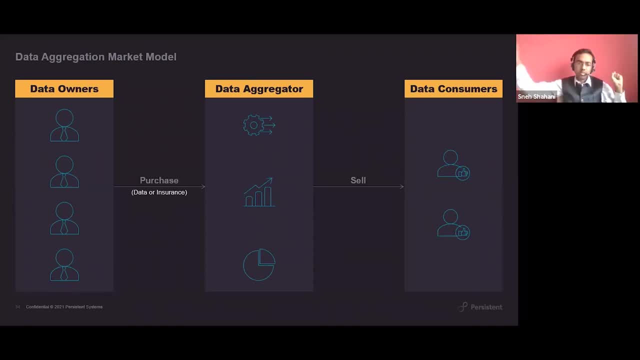 so we acquire the data from these individuals and sell the data to the consumers. so we acquire the data from these individuals and sell the data to the consumers. so we acquire the data from these individuals and sell the data to the consumers. so we can either make some upfront payment to those individuals, that in 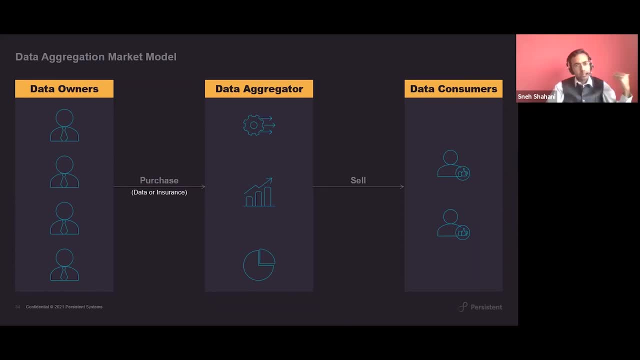 you give the data will pay you some money, or we can provide them assurance or insurance that in case of a data disclosure, you will get this kind of lump sum money. for that we have to pay some money to the insurance provider. so we are paying some money. to put thought or say: 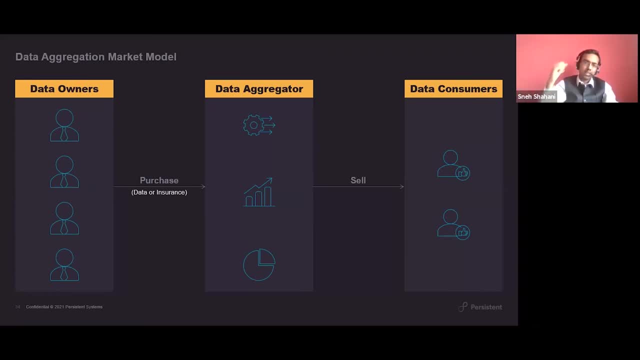 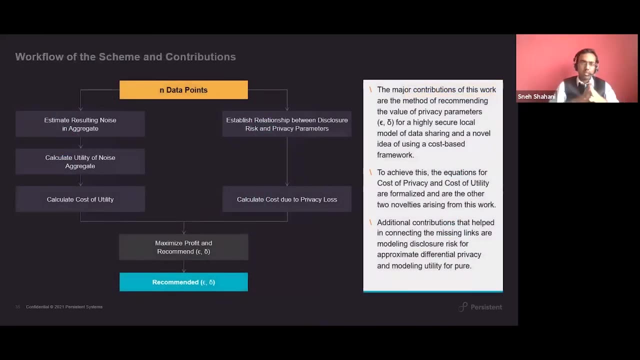 cover the cost of privacy loss, and then we are gaining some money by selling the data to the consumers. so in order to identify a value of epsilon by point at which the profit, this profit, is maximized, we have to- we we did some work on that. so first we have to estimate the resultant noise in the aggregate, and then we 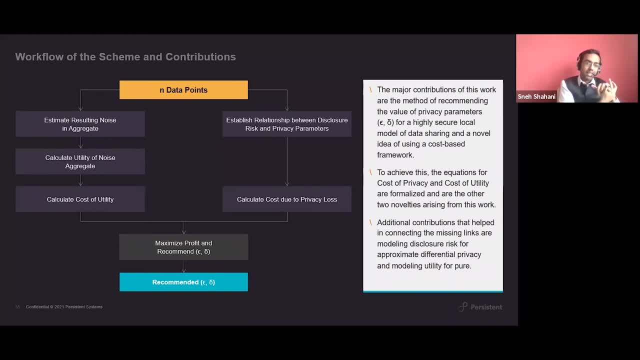 calculate the utility cost of the data. so we have to estimate the resultant noise in the aggregate and then we calculate the utility of noise in the aggregate and then we calculate the cost of this utility. similarly, we have to establish a relationship between disclosure risk and the privacy parameter. 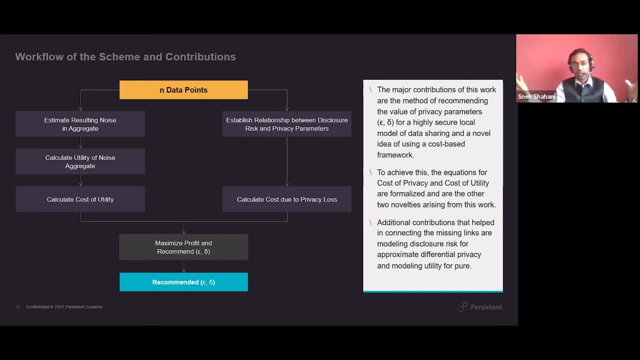 epsilon and then we calculate cost due to this privacy loss and difference of this cost is profit and this point at which the profit is maximized is recommended value of epsilon. the major contribution of our work are first two technique: cost-based technique to recommend value of epsilon. 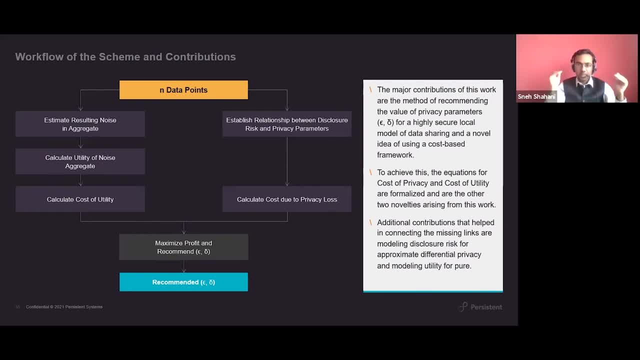 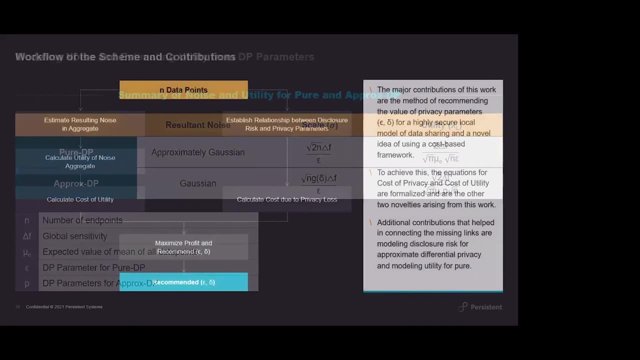 and in order to do that, we have mathematically modeled this cost of price and cost of utility, as well as we have mathematical model estimates for usefulness and probability of distress. what's the second parameter there? sorry, previous one, epsilon comma. what is the next one? actually it. 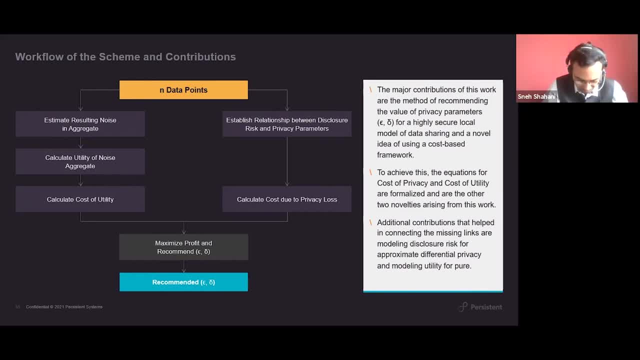 is error value, delta, the allowable error in this epsilon dp. so for this current presentation, current presentation, we are not going to cover that, but it is- there is a separate technique, technique called approximate differential privacy. so in this research paper we have covered that also, both approximate and pure differential privacy. thanks, 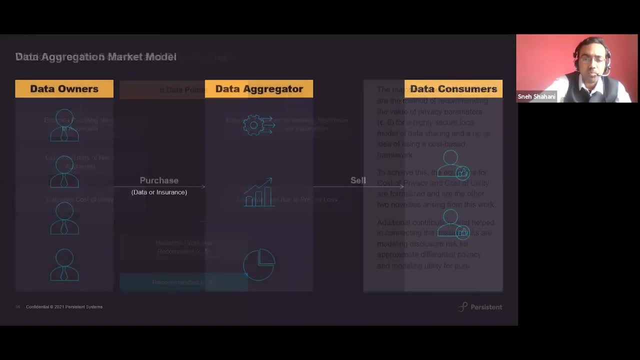 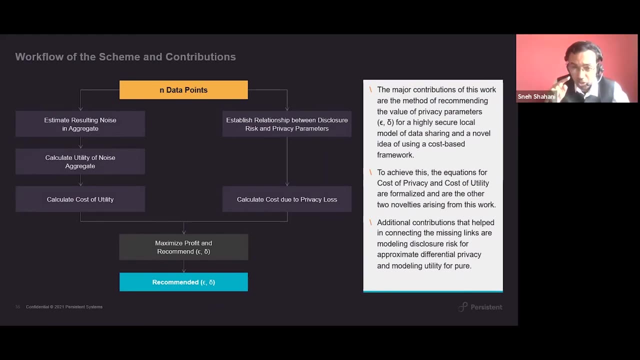 so in the definition of differential privacy that we saw, ratio of those two probabilities, probability on d1 and d2 is bound by e raised to epsilon. there we can add plus or minus delta so that allowable error is allowable approximation in that differential privacy. so this delta has to. 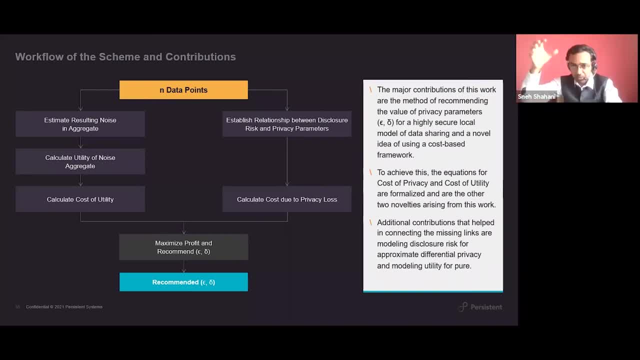 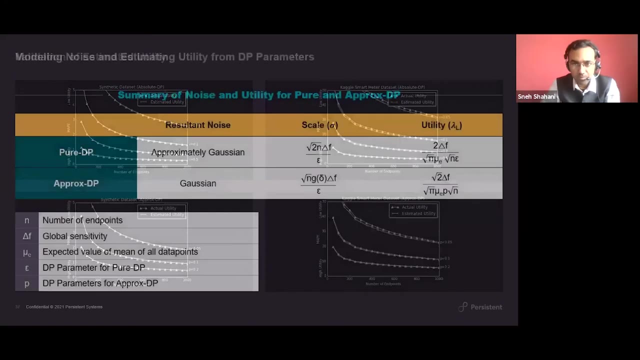 be very small. so there is a separate paper where they have described the maximum value of delta that can be used. so this always thing, all these things are covered in our paper, so i would encourage everyone to read our paper. oops, so for this we have mathematically derived these equations for pure dp and also for approximately 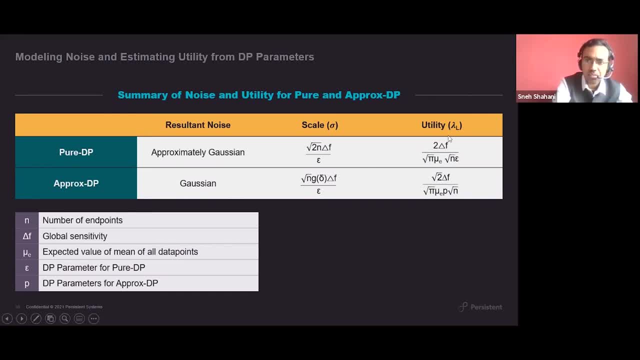 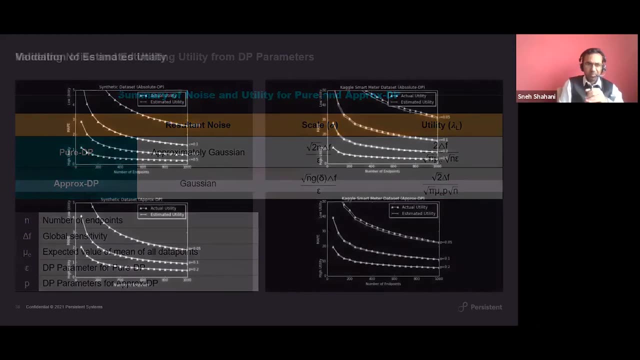 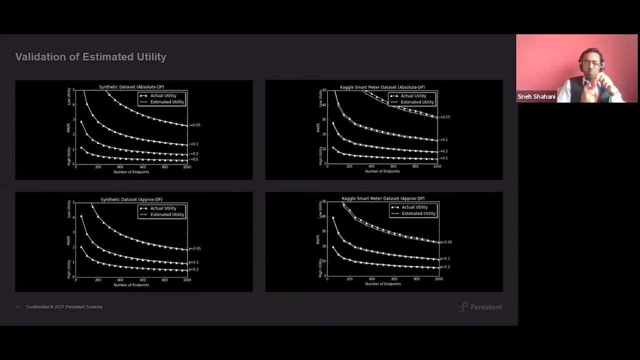 the usefulness is estimated as 2 into delta f, the sensitivity upon root pi. mu is the mean of the data, n is the number of endpoints and epsilon. so this is the mathematical estimate of the usefulness, and this mathematical estimates have been validated experimentally. for that purpose we have taken kegel's smart meter data set. 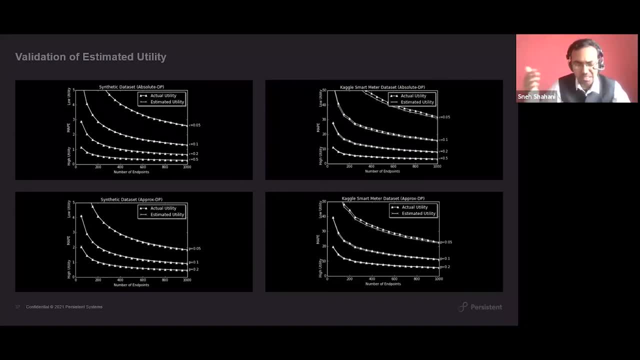 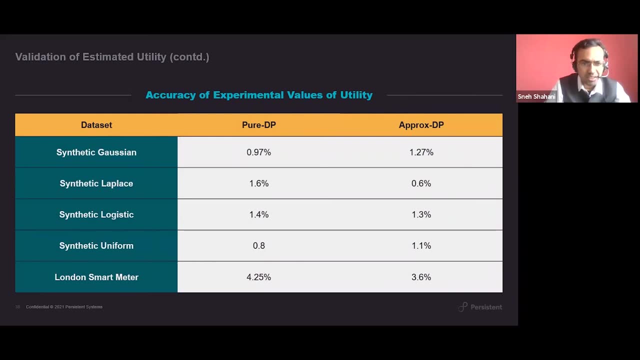 and this and a synthetic dataset that we have generated for various distributions and we have identified that for synthetically generated gaussian data, laplace data, logistic data, uniform data means the data generated from this distribution And the noise. after adding noise, we get the usefulness that is obtained experimentally. 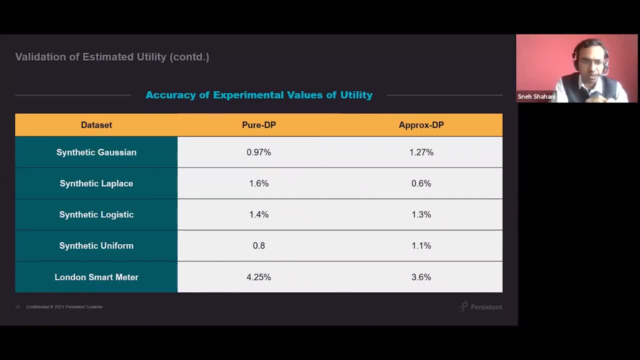 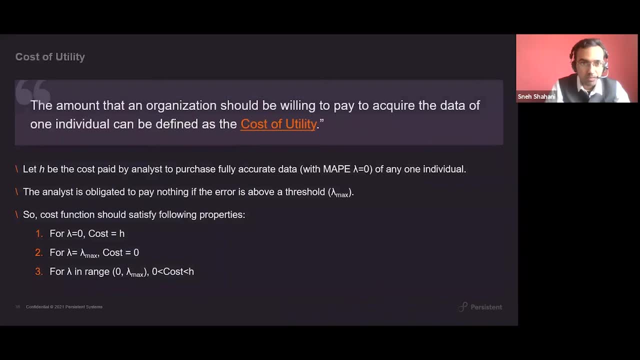 and the usefulness obtained using our formula are fairly close to each other, So we can use these mathematical estimates for calculating the cost. Now we come to the cost of utility, The amount that an organization should be willing to pay to acquire the data of one individual. 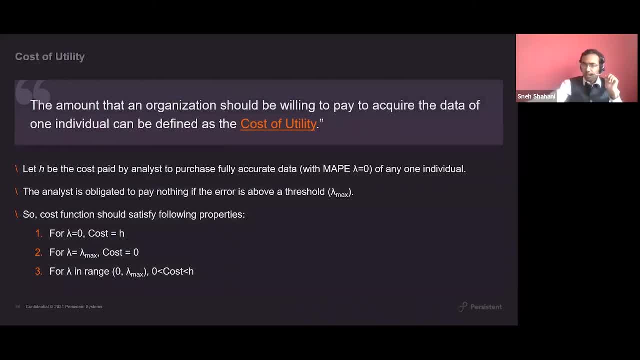 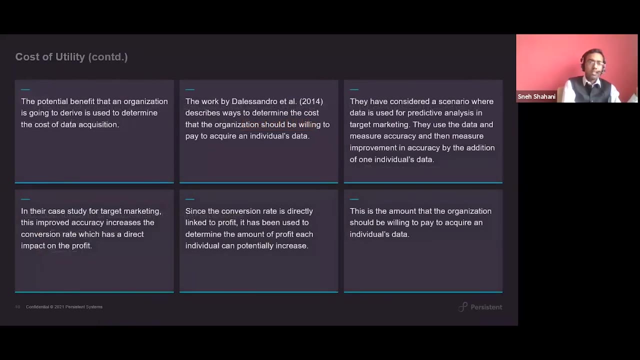 is defined as cost of utility. So we can go deep into this cost of utility. actually We have some time. The potential benefit that an organization is going to derive by using the data of one individual is cost of data acquisition of one individual. 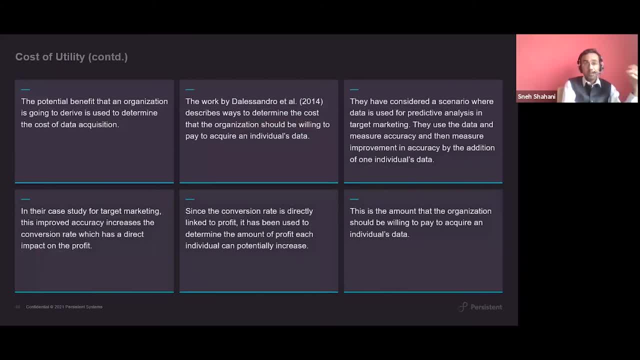 There is a research paper by D'Alessandro et al that describes ways to determine this cost, The cost that one organization, The cost that one organization should be willing to pay. I'll give you one example. We are doing some predictive analysis in target marketing. 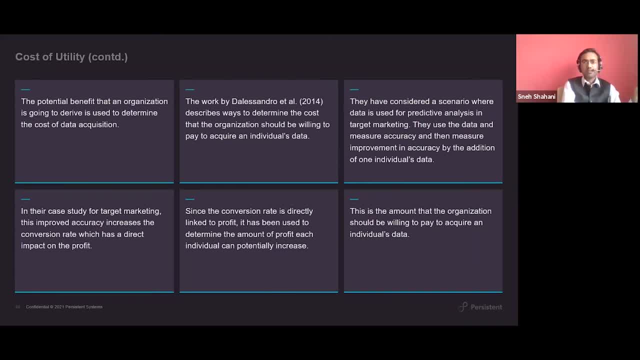 And then we know that our heat ratio is 0.1. And by selling our services to one individual we earn $100. Then acquiring data of one individual gives us 0.1 into 100. That is $10. So $10 is what we get by acquiring one individual's data. 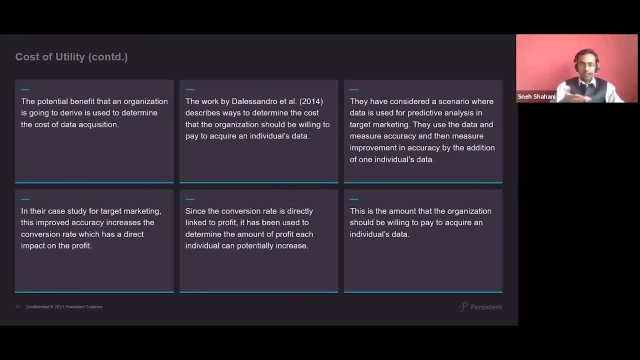 So we should be willing to pay some part from the profit of that data of our earnings, So like that we can calculate the cost of data acquisition, The cost that we gain from acquiring one individual's data. This is the amount that our organization should be willing to pay. 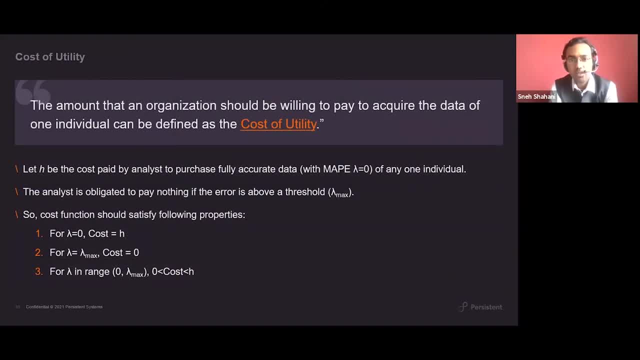 So let H be the cost paid by analysts to acquire fully accurate data, That is MAP or the mean absolute percentage error lambda equal to 0.. And then we decide a threshold, say maximum error, beyond which we will not pay anything. 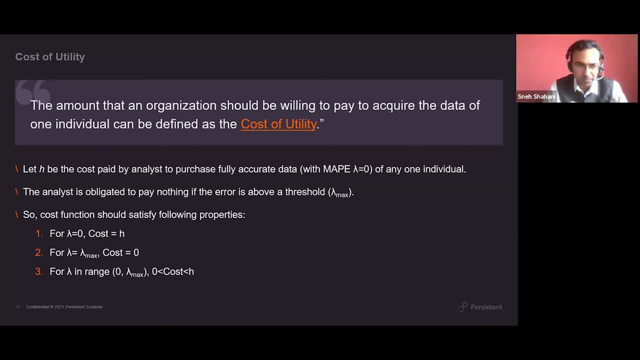 If the error crosses a threshold- lambda max- we don't pay anything. So the cost function that we are targeting should satisfy some properties. At error equal to 0, cost is H. When error is lambda max or more, cost is 0. 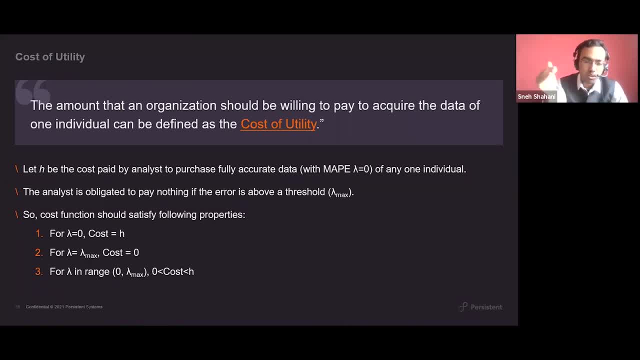 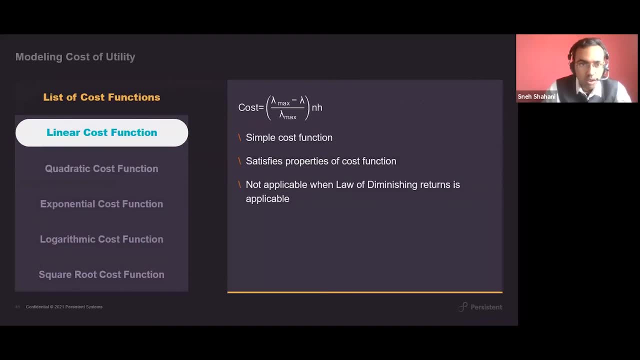 And in this range 0 to lambda max, the cost is 0 to H. So this can be given by some cost functions like linear cost function. The linear cost function is lambda max minus lambda by lambda max into N, into H. 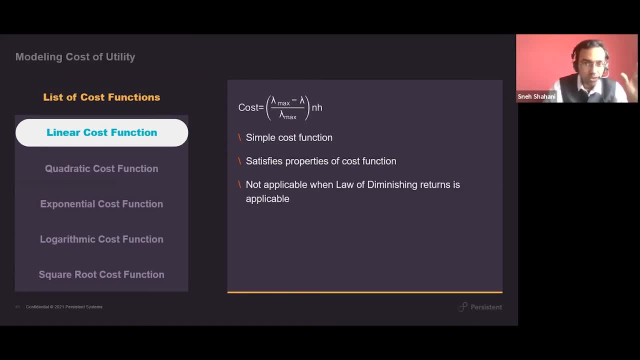 So, as we are acquiring data of N individuals, N into H is the cost And, based on the accuracy, we are paying lambda max minus lambda by lambda max into N H. This is a simple cost function. It satisfies all the properties, but it is not applicable when diminishing returns is applicable. 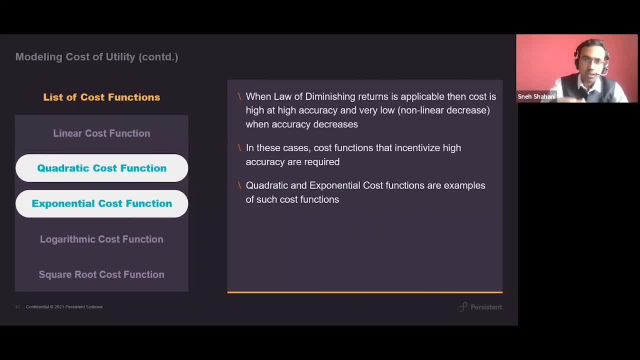 So when the law of diminishing returns is applicable, then cost is high for high accuracy, but very low. It diminishes very fast as the usefulness reduces. So in this case we have to incentivize high accuracy but then penalize even slight reduction in the accuracy. 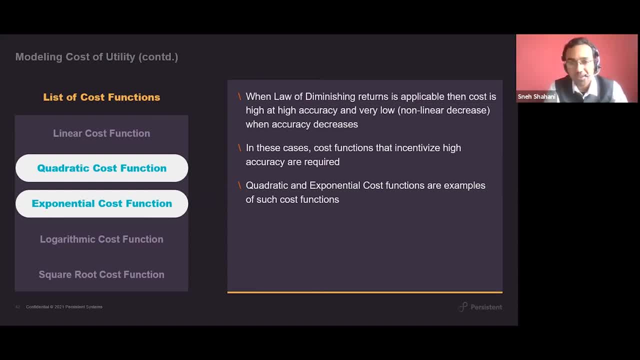 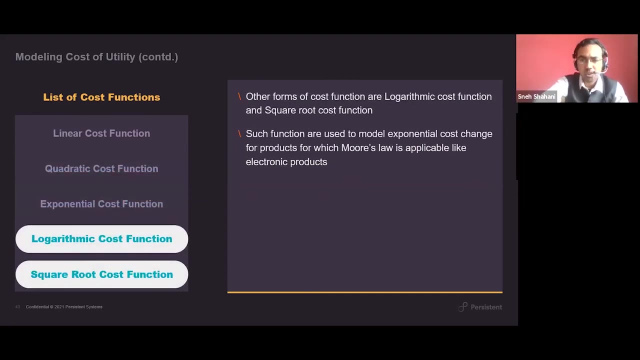 So quadratic function and exponential function are examples of such functions. So we use quadratic and exponential cost function in this case, And there are some other cost functions like logarithmic and quadratic, And there are some other square root cost functions that are used for electronic items when Moore's law is applicable. 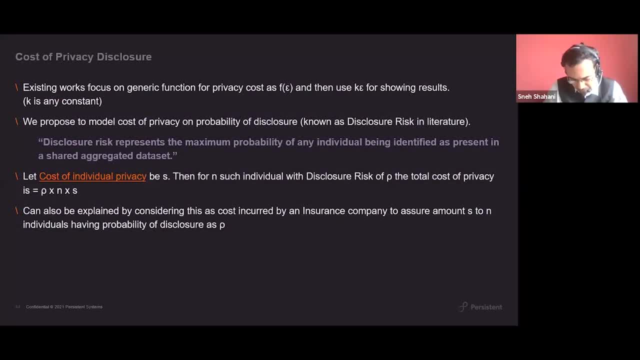 So all these cost functions have been described in our paper And also we described data-driven modeling of cost function. So next comes the cost of privacy disclosure. So we have done a literature survey of existing papers where they tried to estimate the cost of privacy loss. 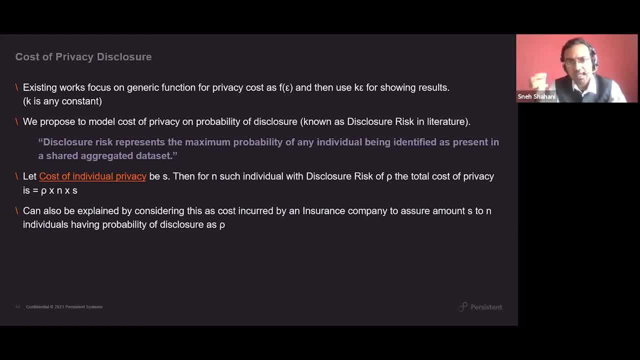 And most of the research papers they have shown. they use a generic cost function, f, of epsilon, And then for experiments they use a constant multiple of epsilon, say k epsilon, as cost function. But we propose to model cost of privacy based on probability of disclosure, also known as disclosure risk in literature. 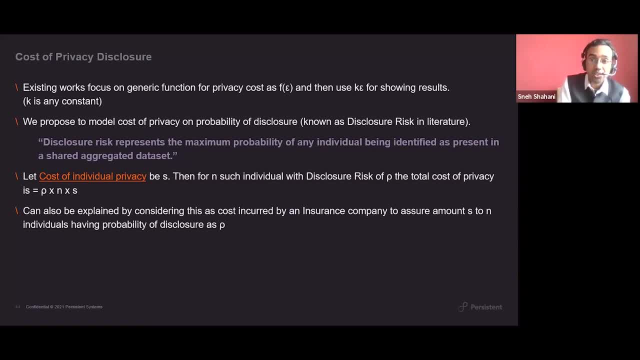 Disclosure risk represents the maximum probability of disclosure, And disclosure risk represents the maximum probability of any individual as being identified as present in the data set. So let cost of individual privacy be s. Then for n such individuals with disclosure risk of rho, the total cost of privacy is s into number of individuals is the total cost. 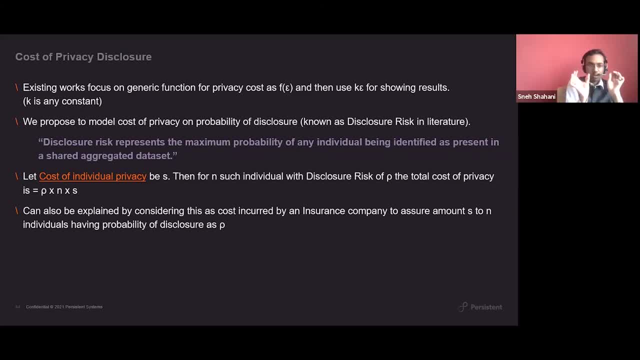 And depending on the probability of disclosure. say probability of disclosure is 0.1, then you multiply 0.1 into n into s. This can also be explained as cost incurred by insurance company to assure the sum s to n individuals having probability of disclosure rho. 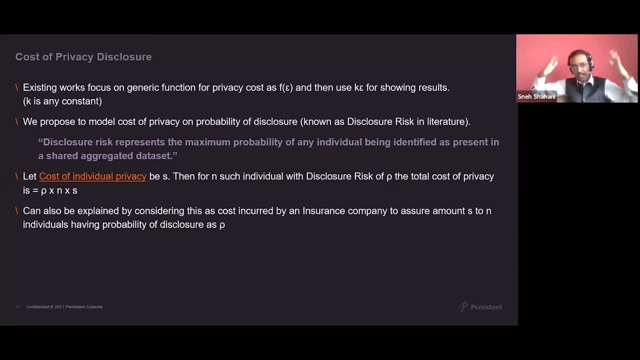 So insurance company will only incur the for a large number of individuals. if probability of disclosure is 0.1, then insurance company has to pay only in case of disclosure. So the total payment made is multiple of the probability of disclosure. 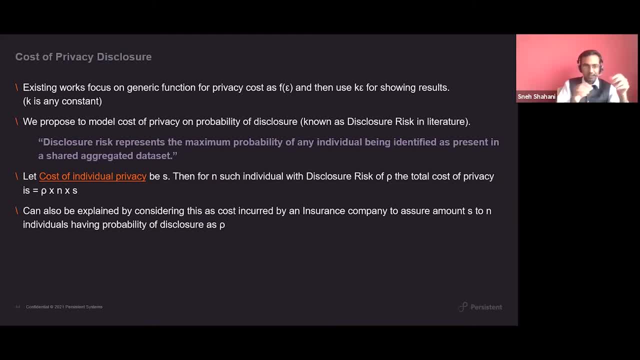 So that is the amount of premium that they can charge. Of course they are going to charge some additional service charges also, But this is fairly how simplest way to calculate the probability of insurance cost. So this is the actual cost that data aggregator will be paying to provide assurance of privacy to an individual. 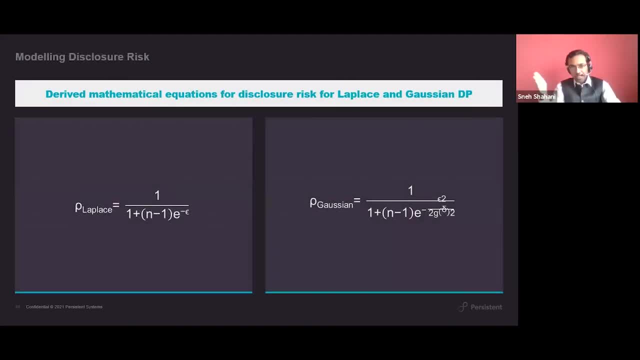 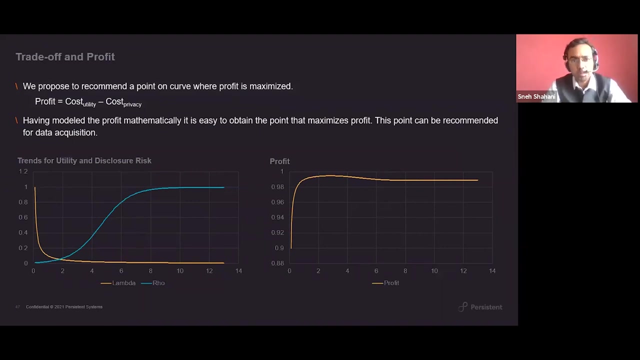 So in our paper we have mathematically derived the probability of disclosure in terms of epsilon for pure and approximate DP. So now we so what we propose is we propose a point on the curve where profit is maximized. So profit is cost of using the data and cost that we paid for loss of privacy. 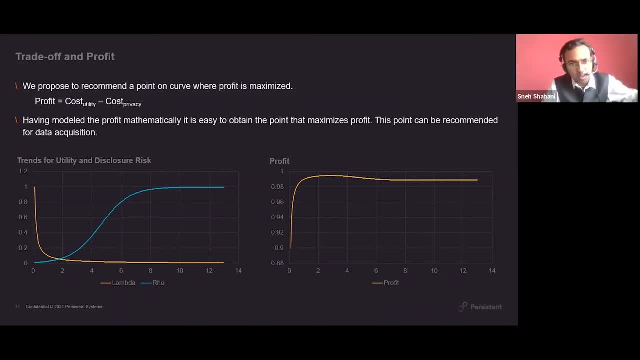 The difference between these two costs is the profit, And as we have modeled all these things mathematically, now we can simply vary the value of epsilon and obtain the point at which the profit is maximized. Here we can see that lambda is the usefulness that is reducing, and disclosure is that is increasing. 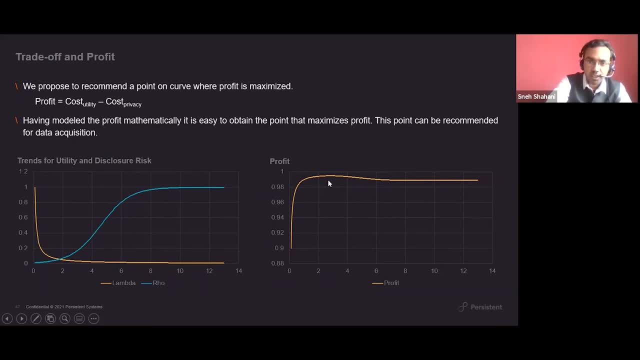 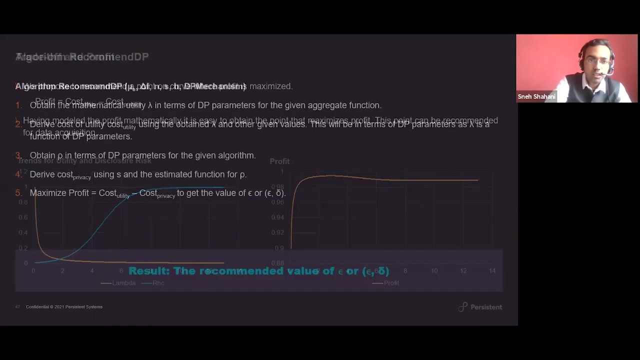 And this is the profit curve. The point at which profit is maximized is recommended as the optimal point of: Okay, this is the value of epsilon. The x-axis in both the cases is epsilon. Okay, So we have derived an algorithm to recommend DP. 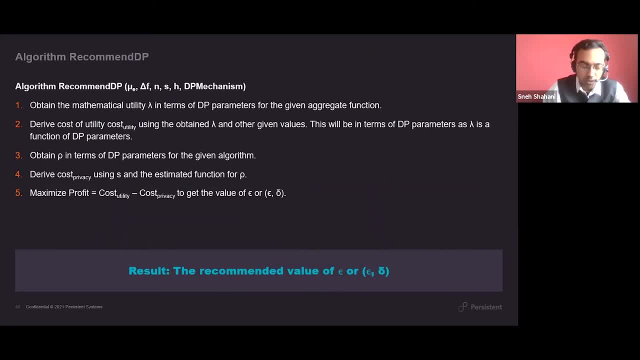 So we use some data parameters like mu, sensitivity, number of endpoints. We also need the value of cost parameters h and s, And we need to know the DP mechanism. Using these inputs, we can follow this algorithm to get these estimates and then maximize the profit. 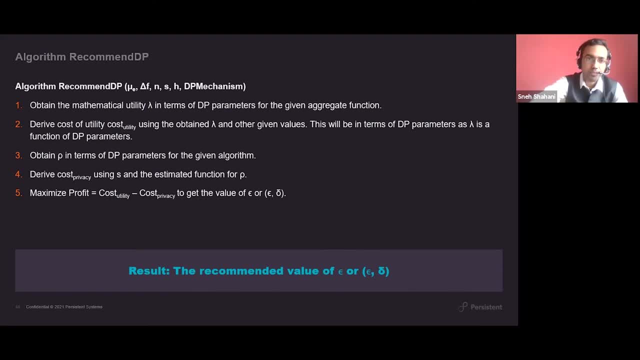 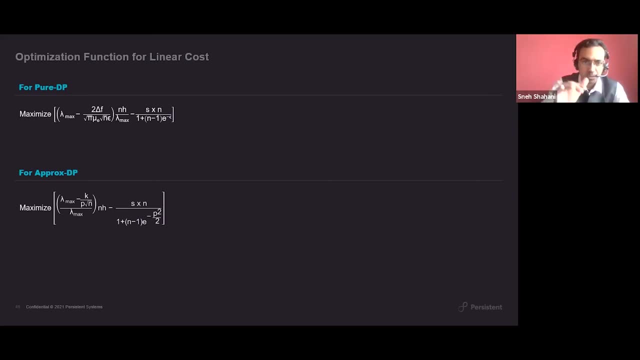 To select the value of epsilon. So we have derived these optimization functions for sum for pure DP and approximate DP, So lambda, max minus 2, delta f by root, pi, mu, root n, epsilon. So delta f, mean and number of endpoints are constant terms. 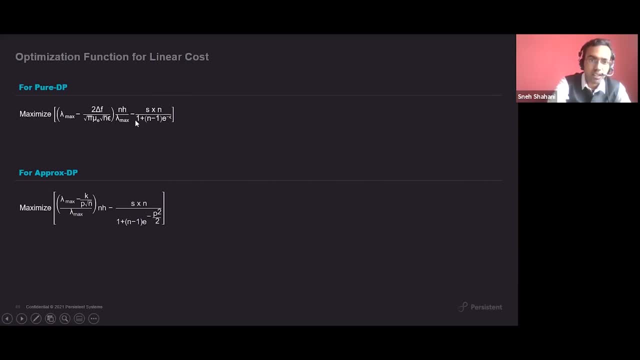 Also this h and s are the costs that are known values. Okay, So only variable term in this equation is epsilon, And by varying the value of epsilon, the point at which we get the maximum value of this profit is selected as the recommended value of epsilon. 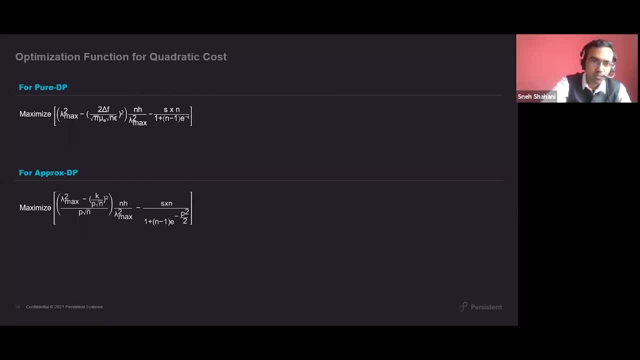 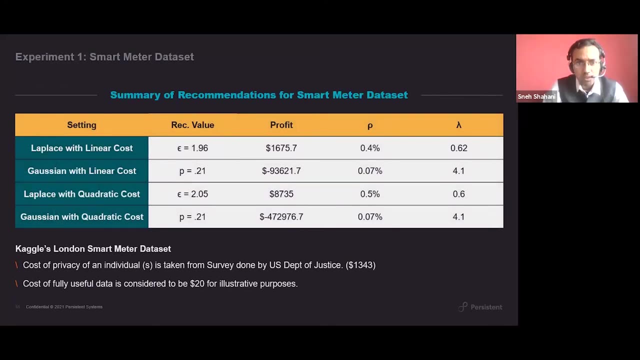 Like that we have derived for other cost function also. So using our formula we have identified recommended value of epsilon for Linear cost as well as quadratic cost for different techniques. So Laplace mechanism as well as Gaussian mechanism of differential privacy. 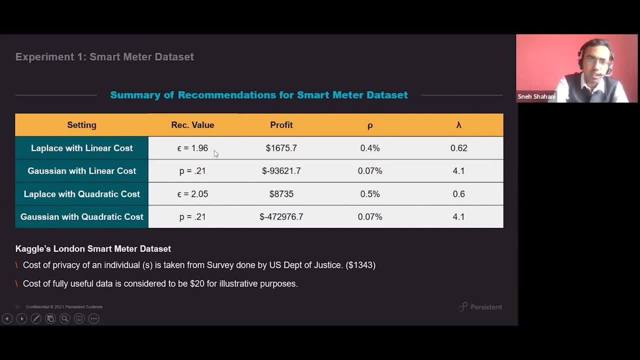 So here we can see that at optimal point Laplace technique is giving some profit, while Gaussian technique is giving some loss. So in a way we can also select. if there are multiple techniques of differential privacy for same mechanism, We can also select that at optimal a particular technique has more profit. 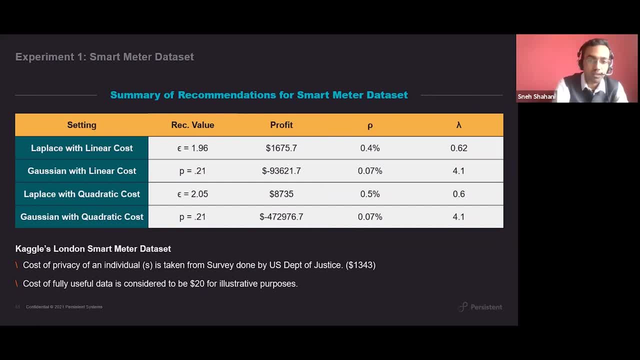 As compared to other. So we select Laplace cost Laplace mechanism for this technique. Also, the cost of privacy that we have used is taken from survey done by US Department of Justice, That is $1343.. And cost of using the data has been selected as $20 for illustrative purposes. 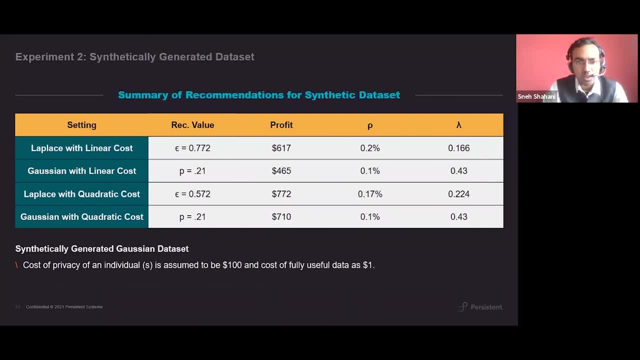 We have derived same values for synthetic data set also. Here also we can see that When we use Laplace mechanism, the profit is $617. And while using Gaussian mechanism profit is $645.. So in this case also, Laplace mechanism is preferable. 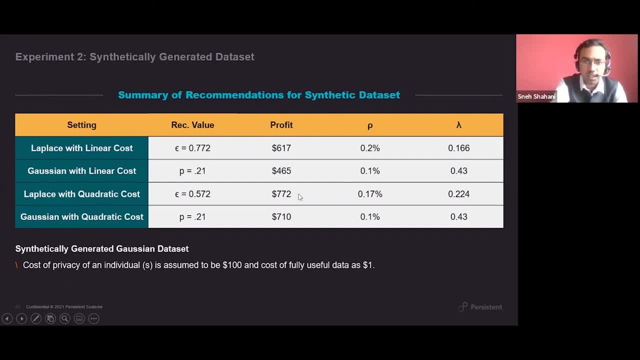 Even while selecting quadratic cost, the Laplace mechanism is giving more profit. So at optimal, Laplace mechanism is more suited for this particular data set. So we use this particular method to make a general recommendation of the technique, But when we know we have to implement data aggregation scenario for a particular type of analysis. 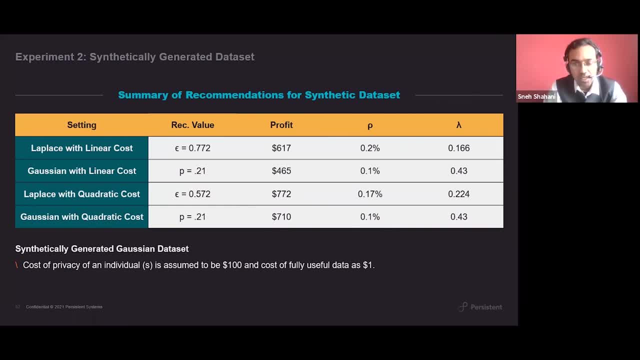 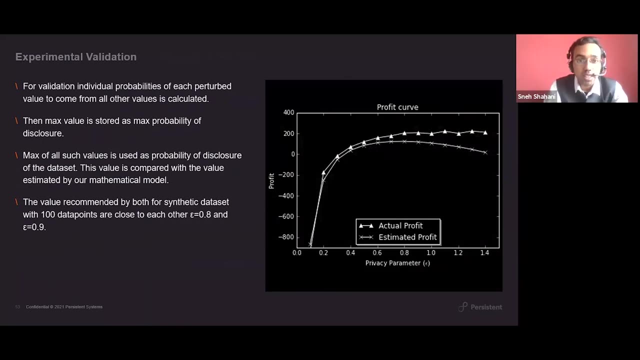 then we can select the value of method of differential privacy for that kind of analysis And also we can select, recommend a value of epsilon for that technique, once we have selected the technique. So we have also experimentally validated of our technique the recommended value of epsilon. 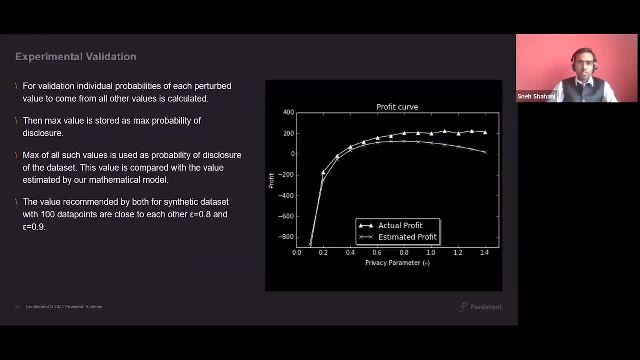 so for that purpose we have to calculate the probability of disclosure experimentally. this is a very computationally intensive process, calculate large number of probabilities. so so we selected, took only 100 data points, and then we computed the probability of disorder like this: say, there are four actual n and actual values. 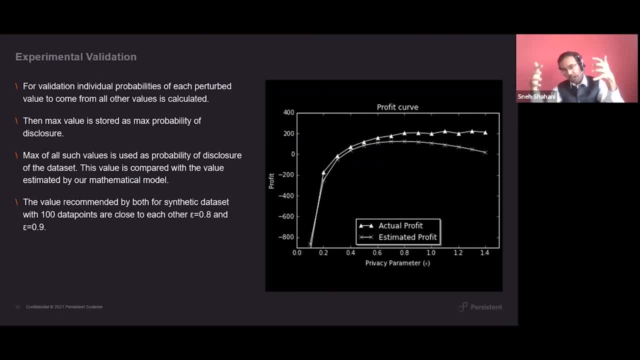 in actual data set and then we add some random noise and we get n number of transform values. then, selecting only one transform value, what is the probability that it came from this data set, that we can identify where we can associate it to the any one endpoint in the data set? 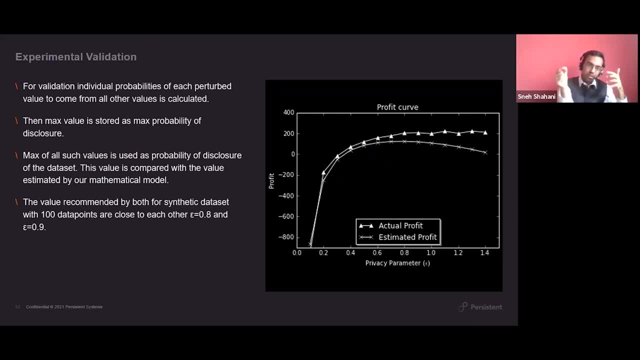 this data set. so we calculate probability of that value coming from any one value first, and like that, we calculate the probabilities for all the value. then maximum probability of that coming from any value is the probability of disclosure of this one data point. like that we calculate probability of disclosure for all other data. 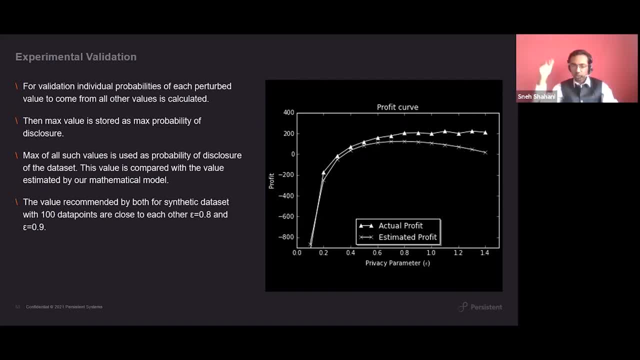 points. and maximum of all these qualities is probability of disclosure of the data set. so, using this experimental value of probability of disclosure and experimentally calculated utility, because we identified the value of epsilon as, say, 0.9, and the mathematically obtained recommended value of epsilon is 0.8, they are fairly close to each other, so our 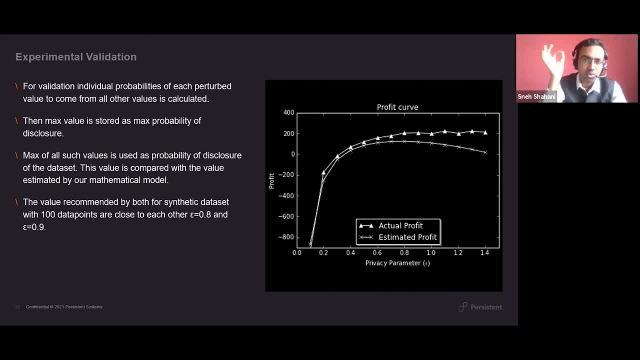 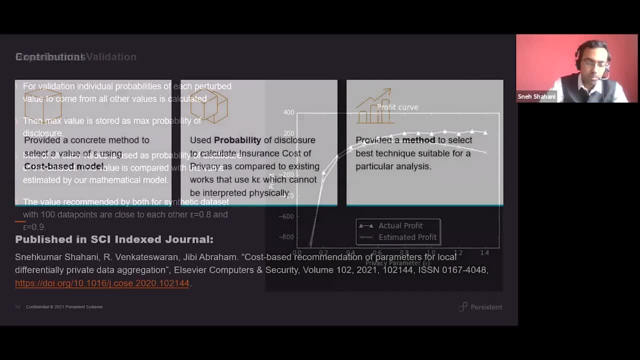 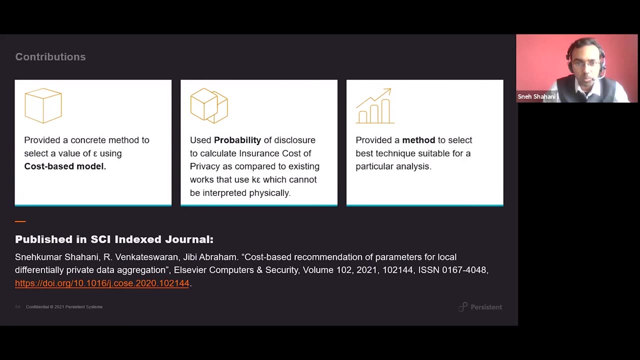 technique is our mathematical formula to recommend the value of epsilon is validated experimentally. So the contribution of this work is we have provided a concrete method to select the value of epsilon using a cost-based model. we have used probability of disclosure to calculate insurance cost of privacy as compared to existing works that use k epsilon, and we have provided 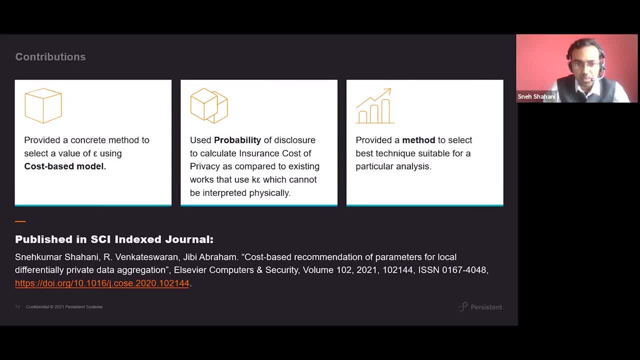 a method to select best technique for a particular analysis. So this work has been published in an SCI index journal and this is known as cost-based recommendation of parameters for local, differentially private data aggregation. So I would recommend everyone, request everyone, to have a look at this paper and we have come. 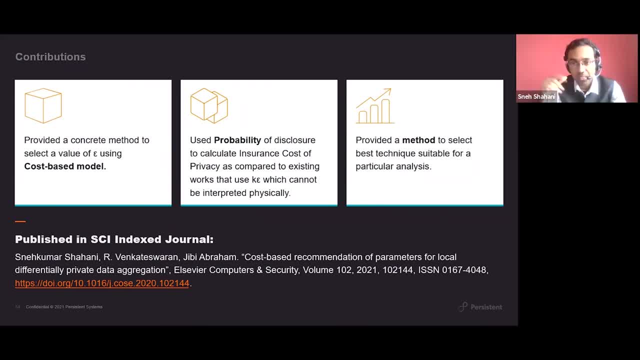 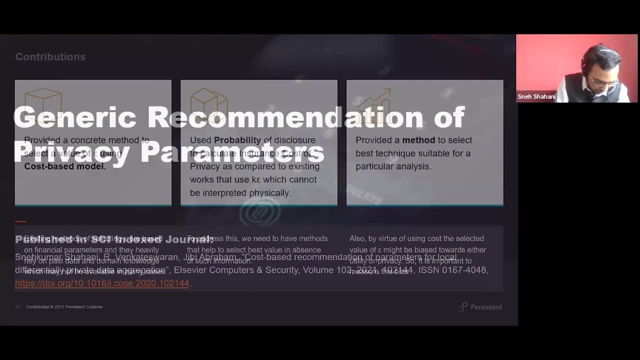 covered all this recommendation technique and all those mathematical derivations in detail in this paper. So we still have 7 minutes, So I have some other things that I can cover. but if you have question, we can answer the questions first and then, if we get time, we will cover all the other things. 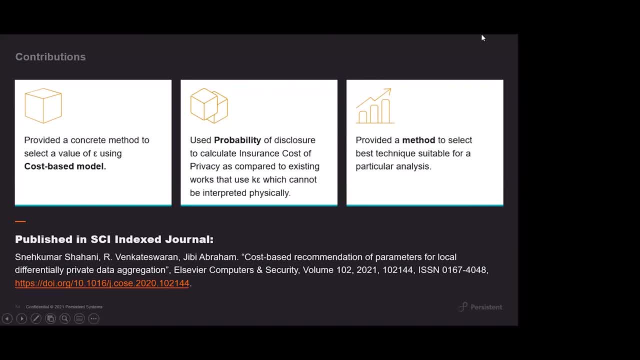 Yeah, Hi Sneh, This is Abhijit. Yeah, Yeah. So this study which you showed of calculating profit, etc. would these algorithms and the studies eventually pressurize companies like Facebook to share their revenue with their users? 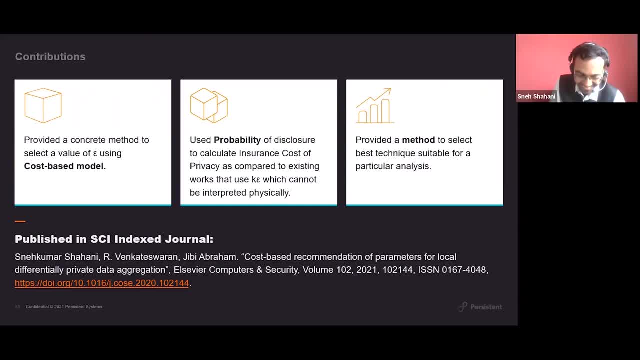 Yes, Actually that's what we want, Because there are some calculations where they have calculated what is the cost of an individual for Facebook and Google. I don't exactly remember, but it was something like $5 for Facebook and $20 to Google. 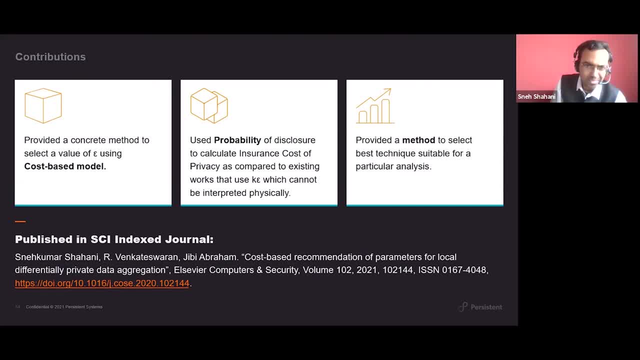 So for each login they gain $20. for the same month- I don't remember the exact time- a year. So there are some calculations where they have calculated what is the cost of an individual for Facebook and Google. I don't exactly remember. 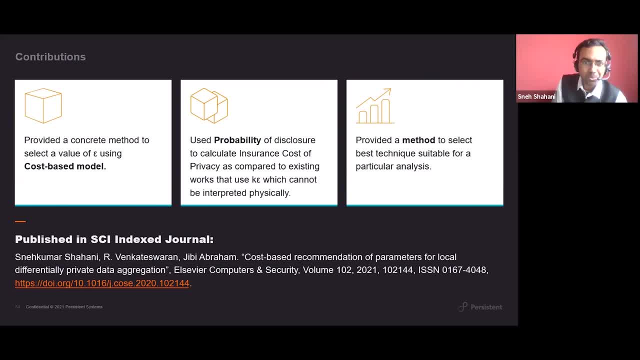 But there is a research paper on that. So if they are gaining so much out by using our data, we also deserve at least some protection, that in case of a data disclosure we should get some money, If not the share in the profit. we deserve some compensation in case of data disclosure. 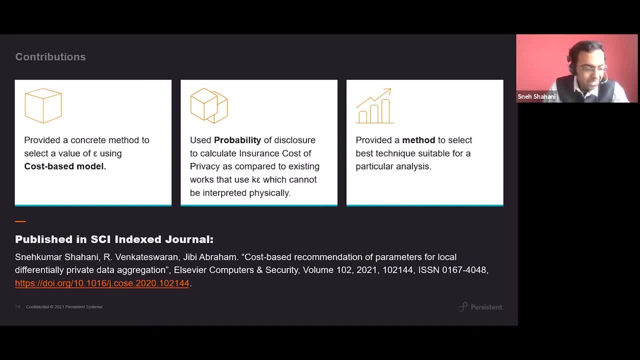 There are some organizations that actually paid people for using their data. Yeah, because, knowing how the US works, There will be enough people putting pressure on these companies using these kind of studies. Yes, That's what we want. Nope, It happens soon. 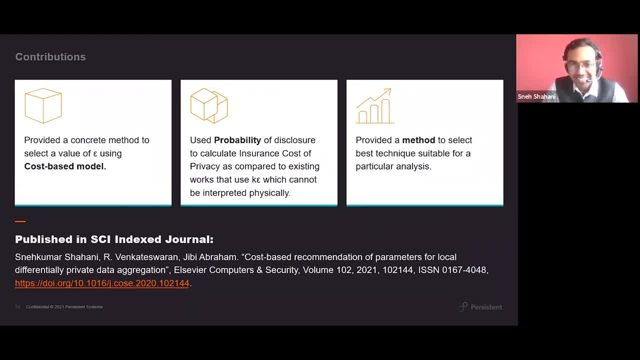 That is our right. Premisee is our right Sneh. one question, Add on question to this: These algorithms and the approaches you have taken for both the differential thing. Have you open sourced these in the public domain? It is published work now. 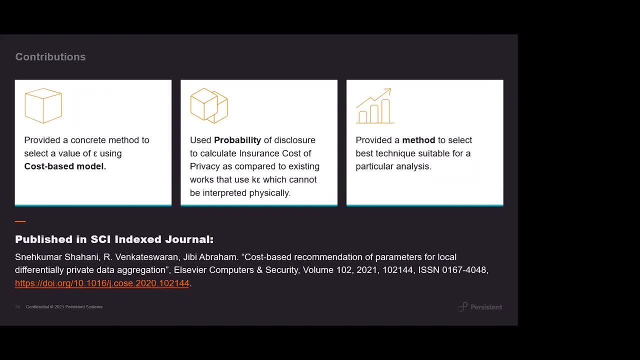 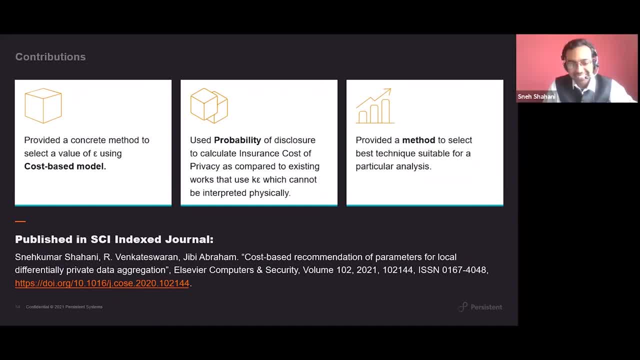 Thank you. Okay, So when you publish you have to sign that all rights have transfer to the publisher. So I have one paper that is accepted, not yet published. I can describe that, But if there are questions we can…. 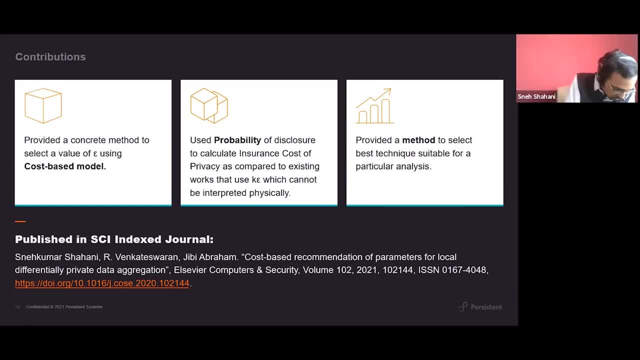 I just have one quick point that you can share later. Yes, please, Please, go on. If you have some of these different kinds of like what you showed on the sample data, these easily…. Yes, the sample data sets that you worked on, um. have you have these curated somewhere on github? that? 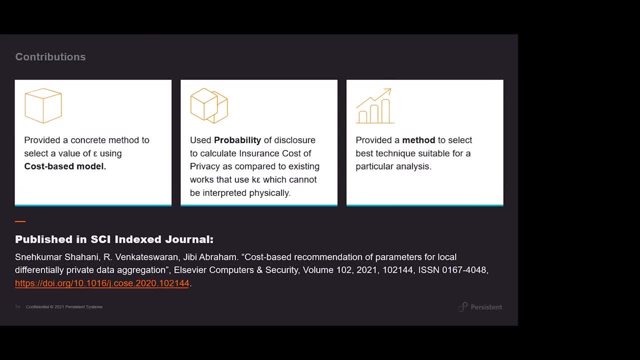 you can share in terms of how you've done some of these analysis that you might actually all this algorithm has been described. i've been described in the paper published a source code. i can think we can think about it. just let me know, yeah, if in case that would be helpful. 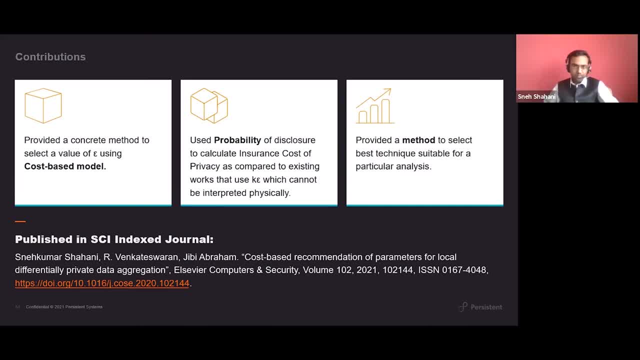 and you don't. you have not published on it on github yet. yeah, in case that happens, do let us know. yeah, thanks, we have three minutes left now so we can even discuss about this federated learning. so in case of predator learning, each individual endpoint is emitting some model, local model of that, that is. 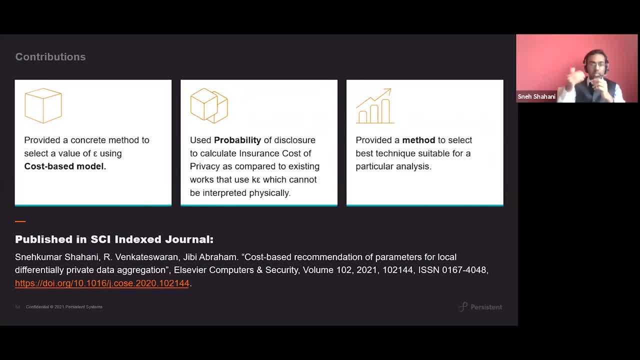 learned from that local data set and using this local model we can run some model inversion attack and get the presence of some individuals on that data set. as we know that any machine learning model will provide very high accuracy on the training data set and comparatively less accuracy on the 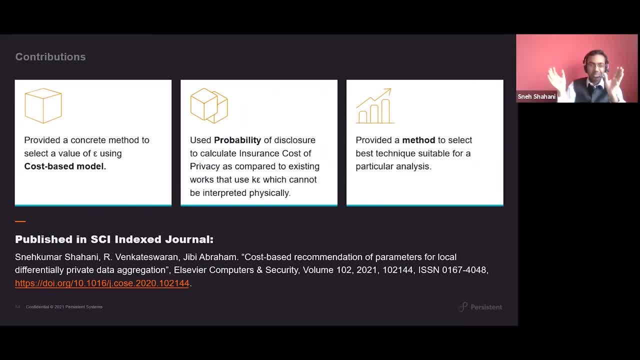 testing test data set. so by comparing these two accuracies we can identify presence of the individual in that data set, whether that was a part. if we get very high accurate. if, say, about one individual, we know all the values, we can predict the value using the model model and we 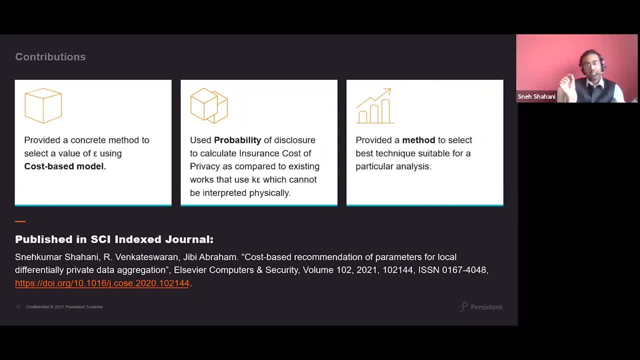 can say: this is very accurate, so this person was a part of the training data set. and it is not accurate, so this person was not a part of the training data set. so using that we can actually identify, say, it is a banking data set. using these models only we can identify whether 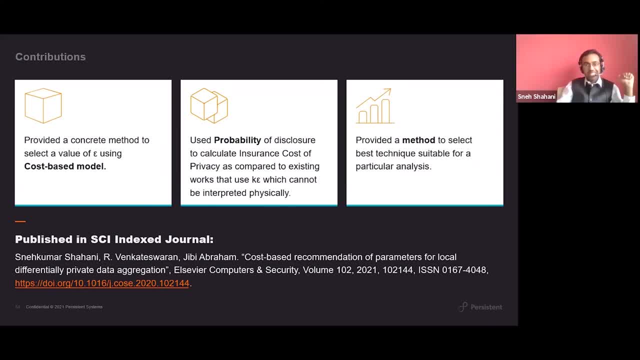 that person has a bank account in that bank or not. so that thing was not supposed to be revealed. but just because we had that model we were able to identify the membership inference or the presence of that individual in that data set. so this kind of a attacks are known as model inversion attacks. so to thought this kind of attack we have to use. 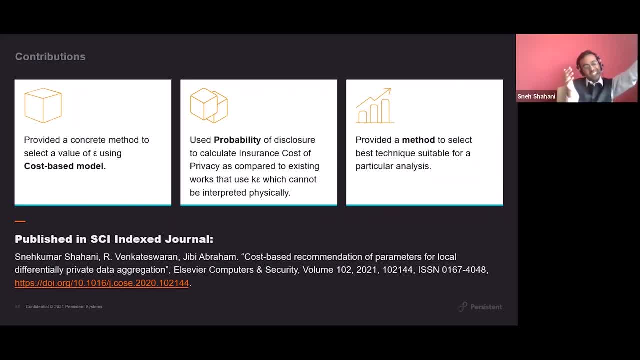 differential privacy on those learned models. so each bank, before revealing the model, will add some noise to the weights before revealing the model, and then, using this noisy version of the model, we compute the final federated model. so that's how it can be applied to federated learning. 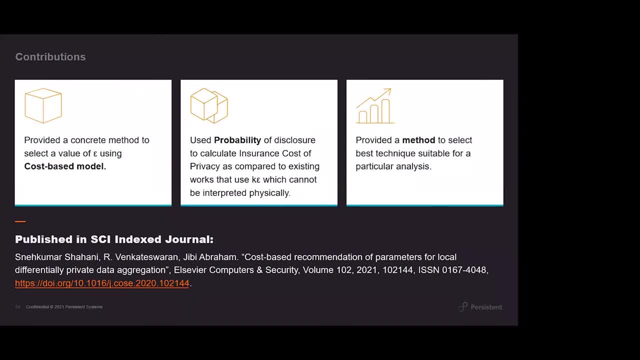 the one question which i had was: see, i think these are extremely powerful and very relevant techniques for privacy preservation. by and large, i'm taking out the security aspect of it, because that has to be factored anyway. now, when it comes to large organizations and large people who have 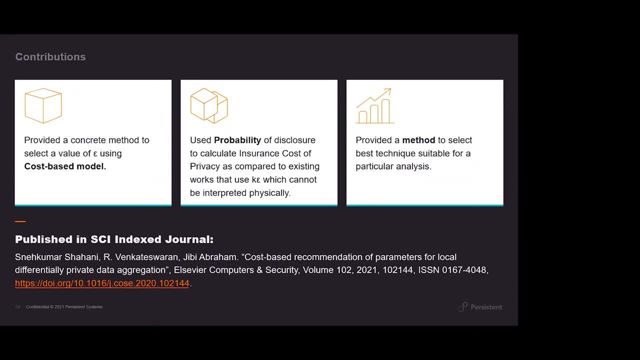 the data. so it almost means that they have two variants of the data that are kept. one versions, of course, which is pii, which is available, and the other version is applying these kind of differential techniques. another version is applying these kind of differential techniques, another version of the data that gets generated, which are already in a, in this kind of a dp formed. 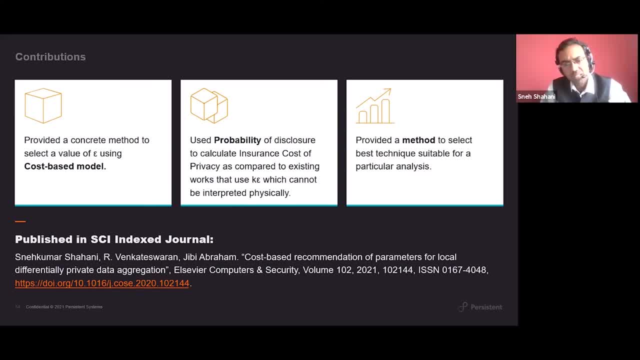 data. so have you seen this being implemented by any large financial institution or any large custodian of data? financial institutions? i have not seen yet, but the largest, biggest implementation till now is this: us census data set. okay, the us census. they have to release uh data of the last decade at the end of every decade. okay, so they have this mandate and 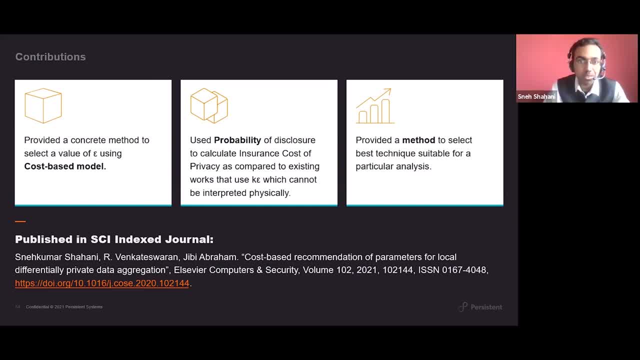 uh, in last ticket, some privacy laws were also passed in us. okay, they are not allowed to reveal everything without providing some plausible delineability to individuals. so they are the biggest consumer of this differential privacy technology. and actually that release of that last ticket data is delayed because this work is going on. how to select the right value of epsilon?